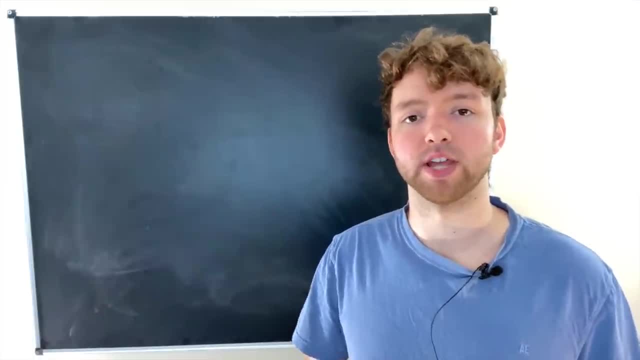 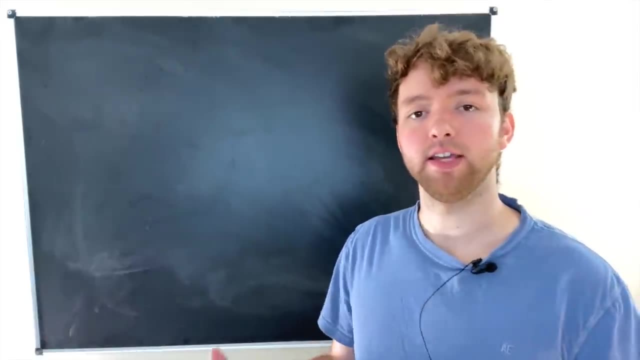 So object-oriented programming helps us represent things in our code. What exactly do I mean? Well, one of the biggest challenges with programming is how do we represent data in our code. In our text culture, we typically, Luckily, programming should be less than three or five ways. The 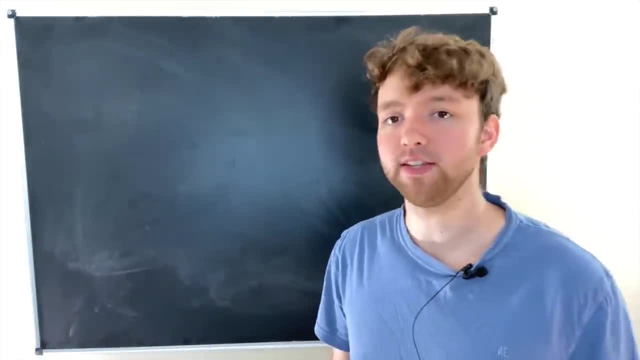 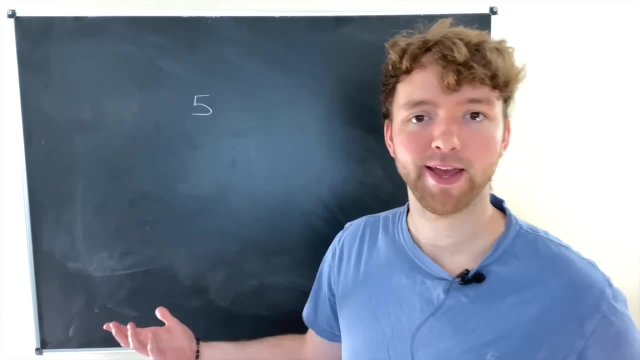 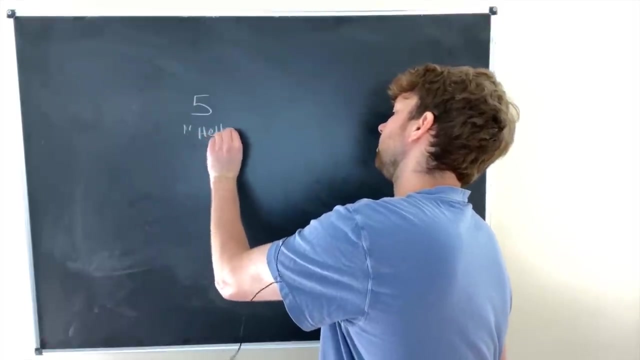 code. If you're just working with very simple data, this is easy. You can use primitive data types and collections. So, for example, if you just had to store the value 5, hey, it's easy, It's just a number. If you need to store a string, no problem And heck, you can be wild, You could. 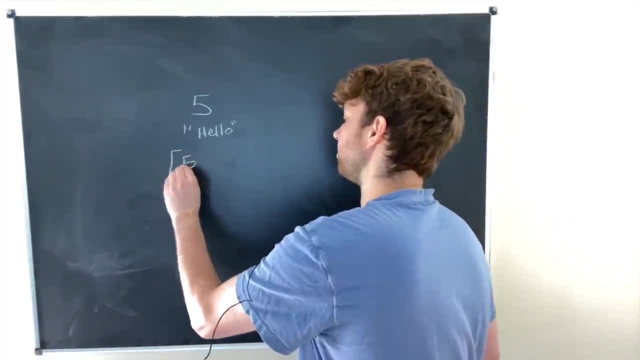 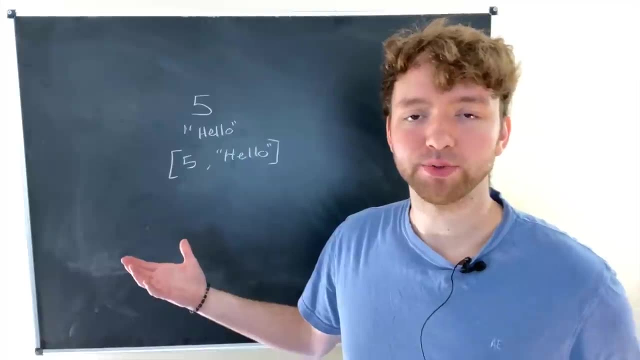 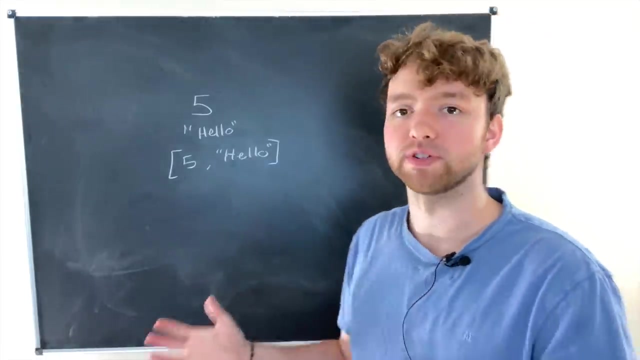 even store multiple things together in a collection such as this, And this would be a list in Python. Okay, So pretty simple data, very simple to represent in our code, just using simple variable types. Now what if you want to represent something a little bit more complex? 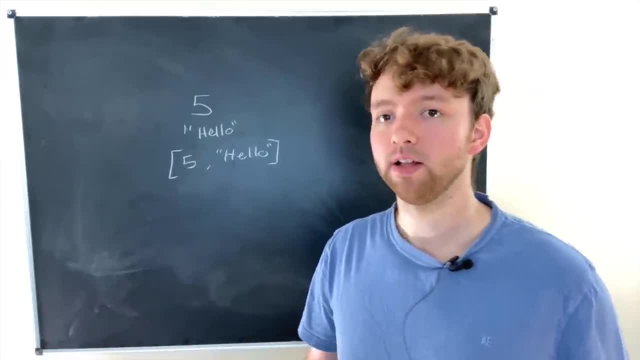 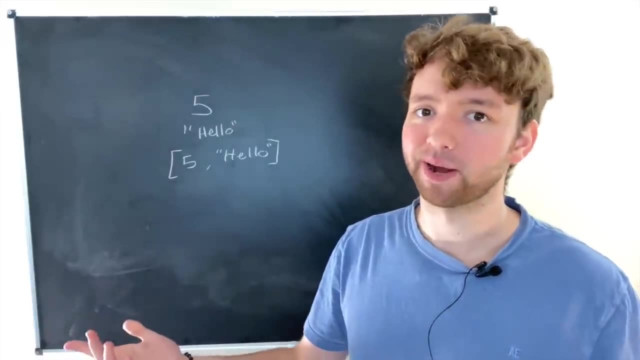 There's various ways to do this. You could use JSON or XML, You could use just numerous collections or you could use object-oriented programming, And that's what we're talking about in this video And another positive side effect of object-oriented programming. 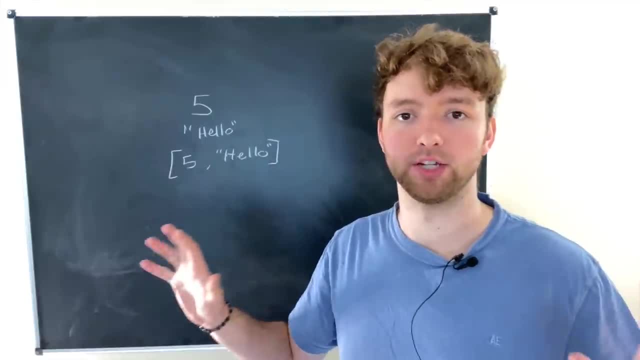 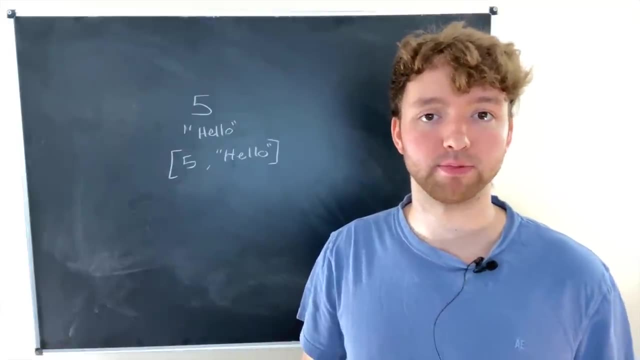 is. it allows us to represent data as a one-to-one relationship to the object-oriented programming, And that's what we're talking about in this video. So let's get into business problems. So, for example, if you wanted to create software to represent customers, you can make customers in your code And I'll show you what I mean. 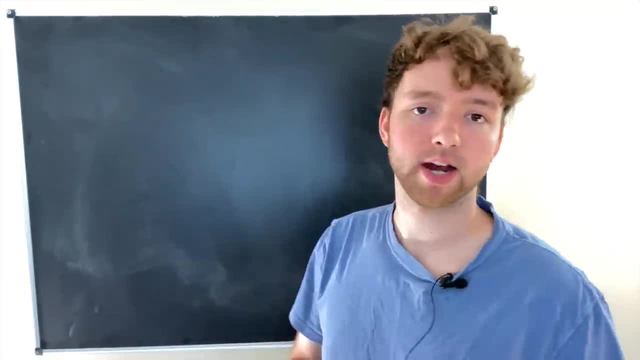 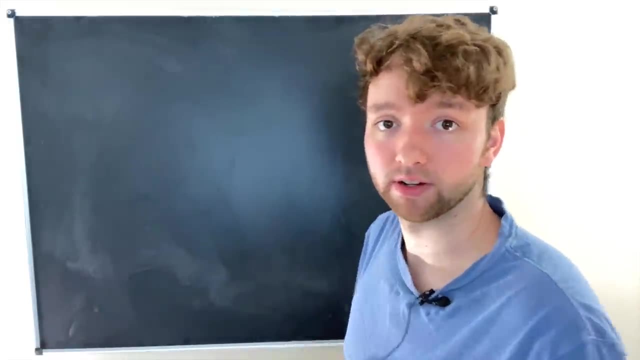 here in a second. So the two big things in object-oriented programming are classes and objects. Classes represent something such as a customer, and then objects are specific examples of that. So let's go through an example here. If we want to write software to work, 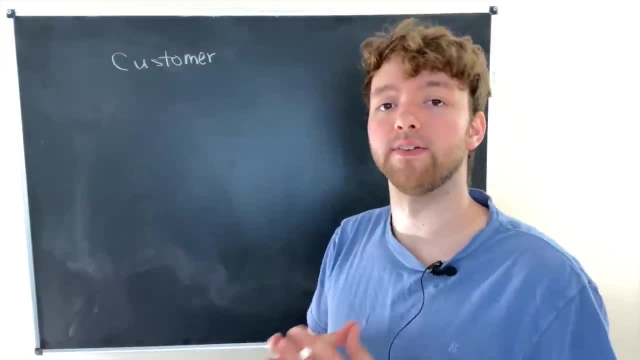 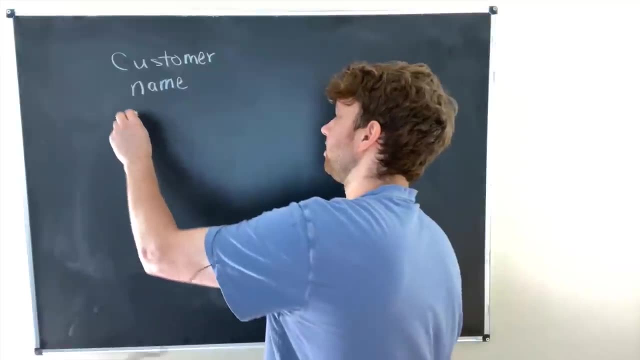 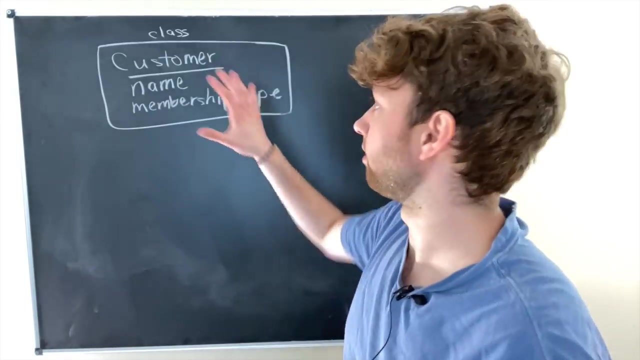 with customers. we could create a customer class and then give a customer a class And attributes such as the customer name or, let's say you had some kind of subscription website or something you could have- the membership type. so this is an example of a class. by creating our own classes, we can group things in. 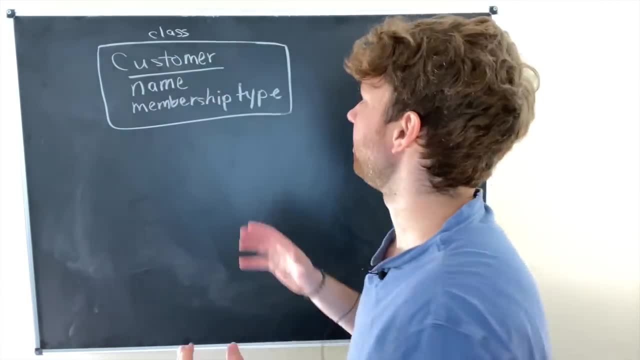 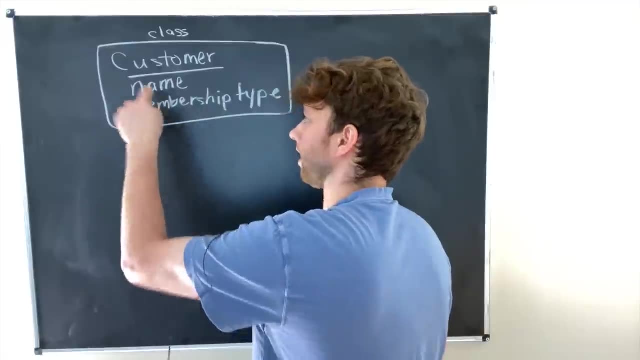 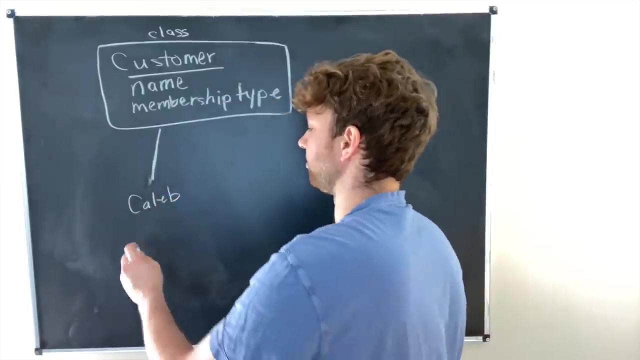 logical units- customers in this case- and then we can instantiate- very fancy word- this class into what are known as objects. so now, instead of having these general attributes, we give it specific values. so, for example, Caleb and my membership type- oh you better believe it's gonna be gold premium, you know. and 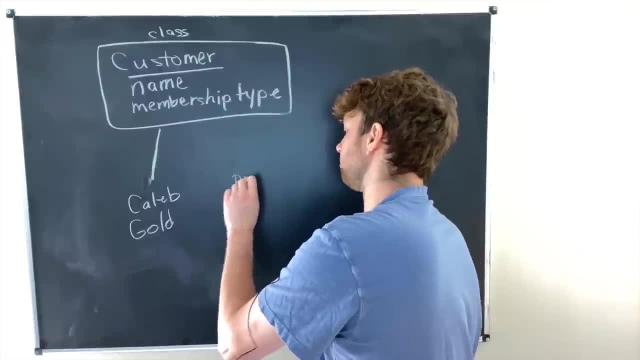 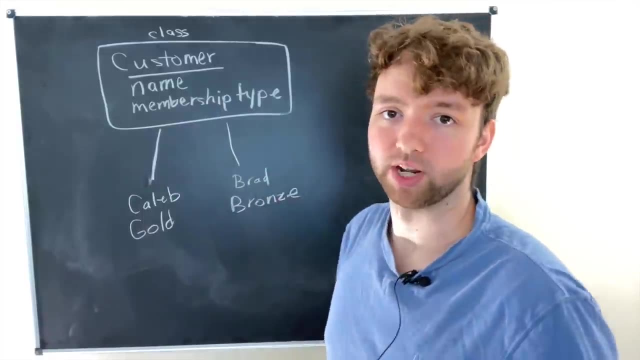 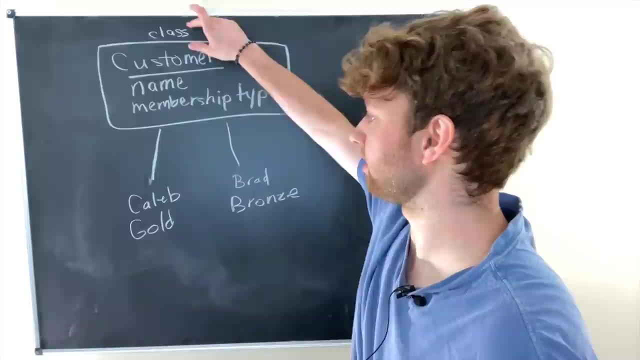 then we could have another object on here, such as Brad, and we could give him, like I don't know, bronze. so these are both objects, and that is the very first thing you need to understand. with object oriented programming, we basically define a structure and what's known as a class, and then we use that. 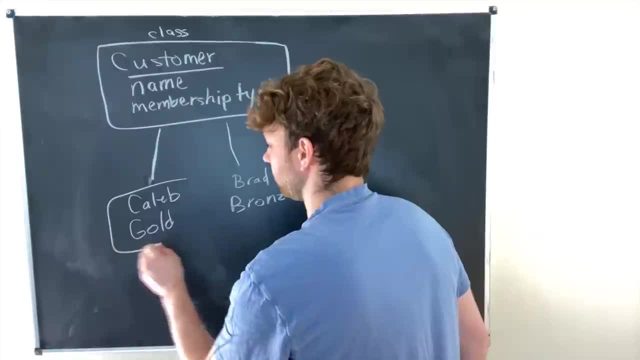 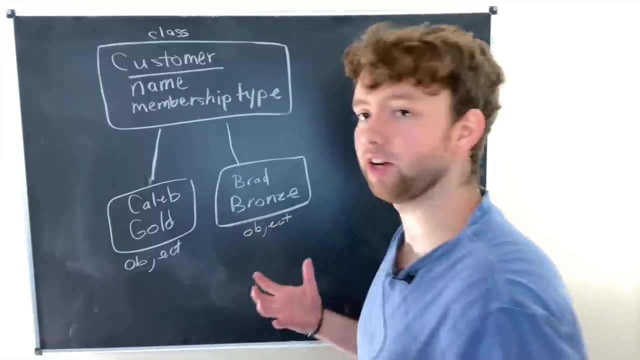 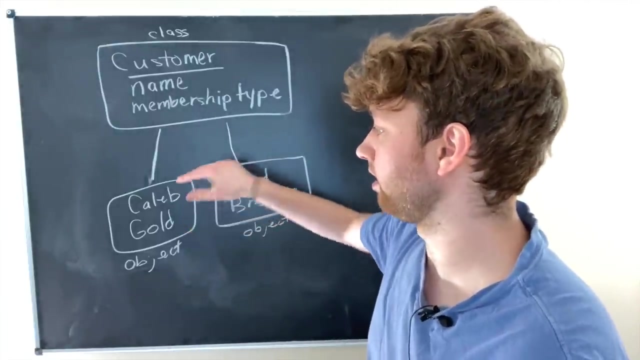 class to create objects. so this is an object and this is another object, and this is very ideal when you're going to have a common structure across numerous things. you know every single customer is going to have a name and a membership type, so that's the very first thing. you create classes, you create the attributes. 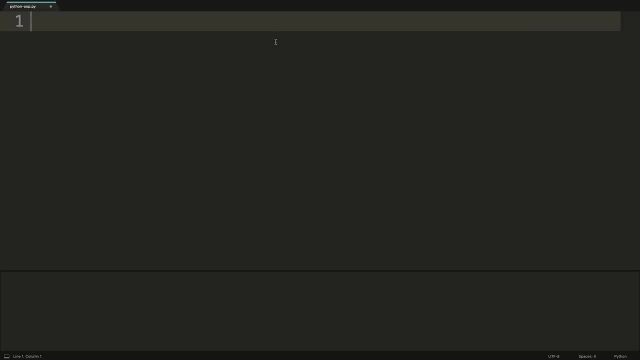 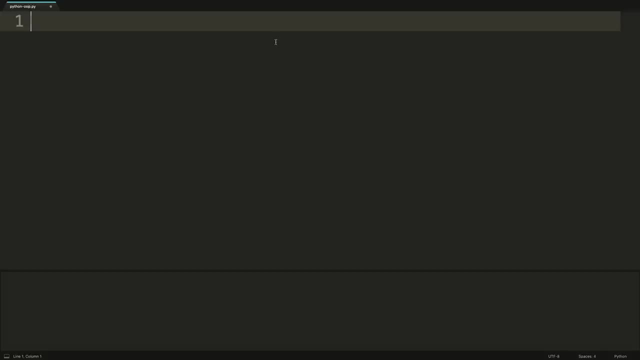 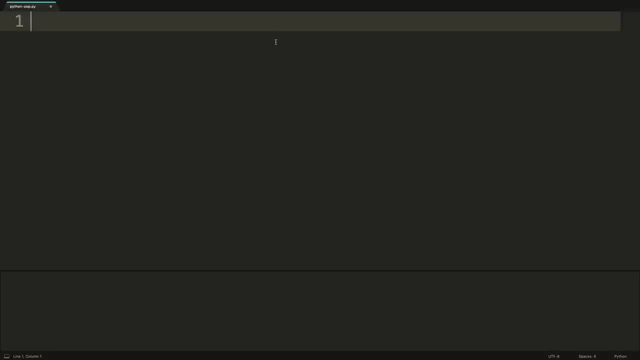 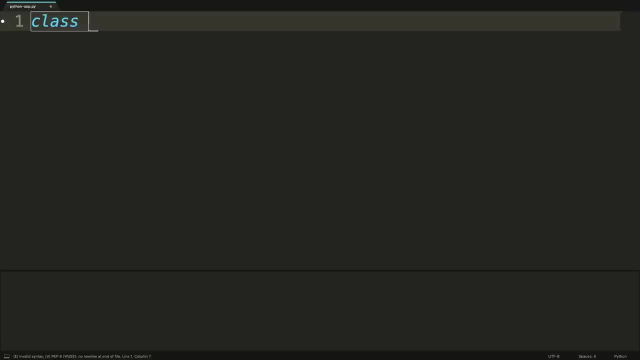 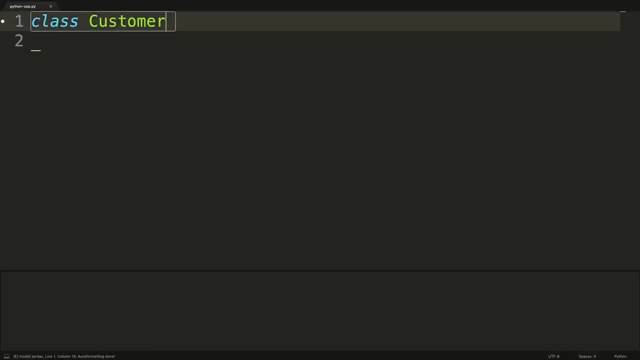 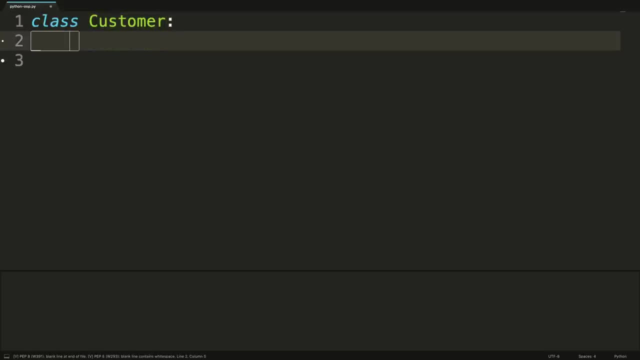 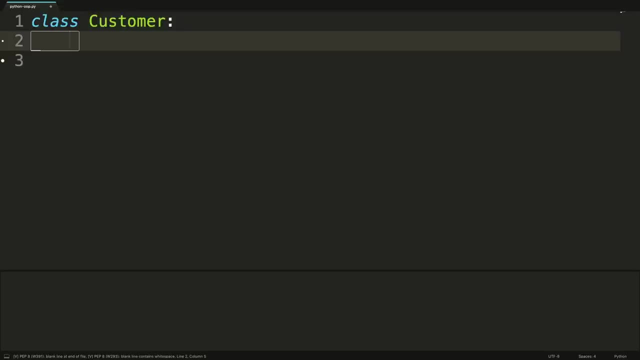 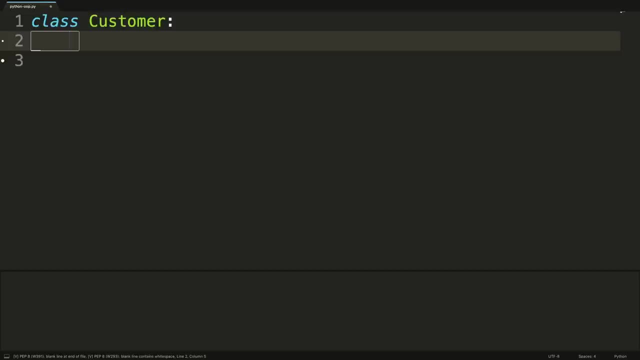 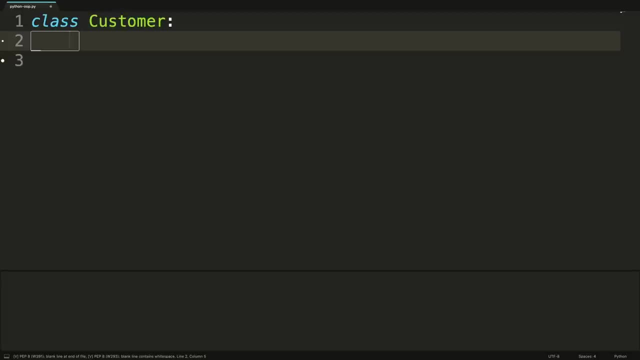 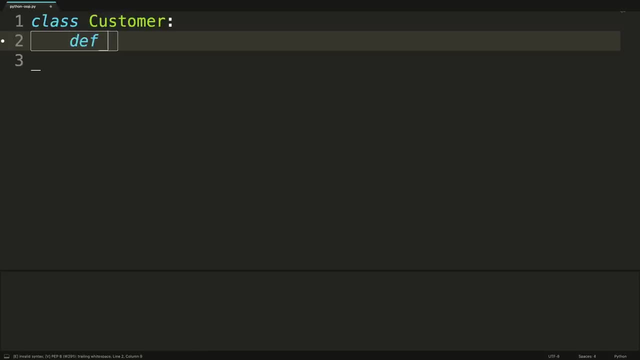 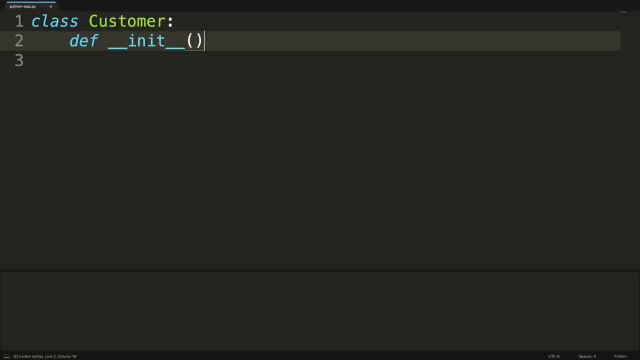 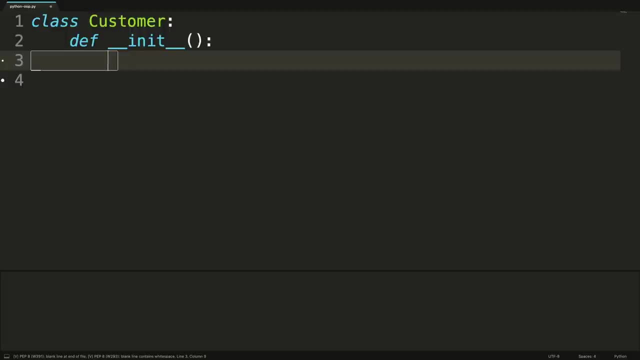 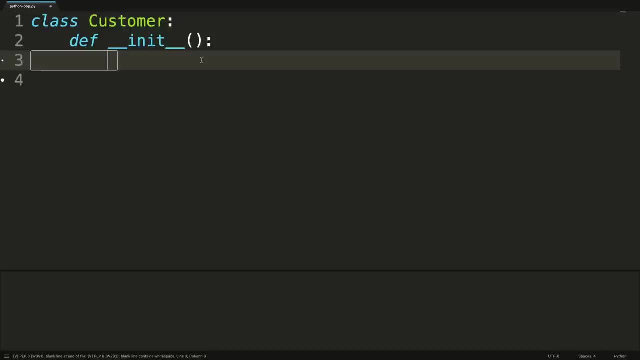 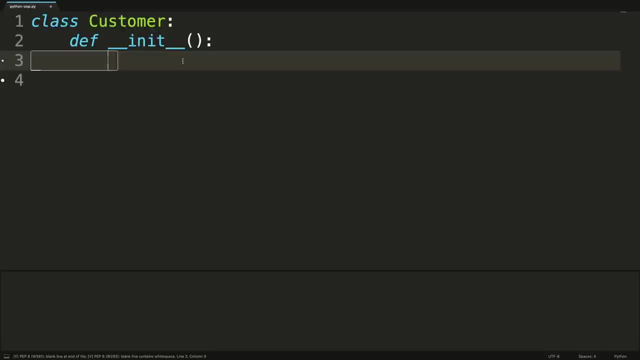 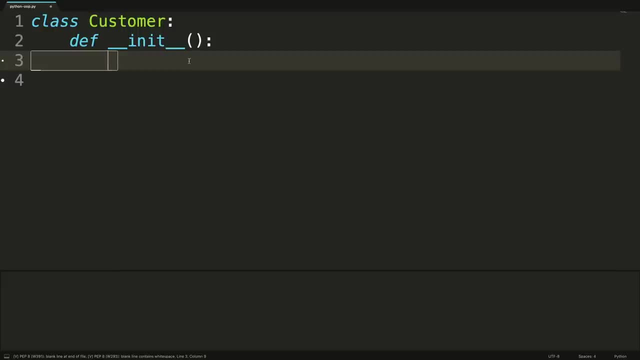 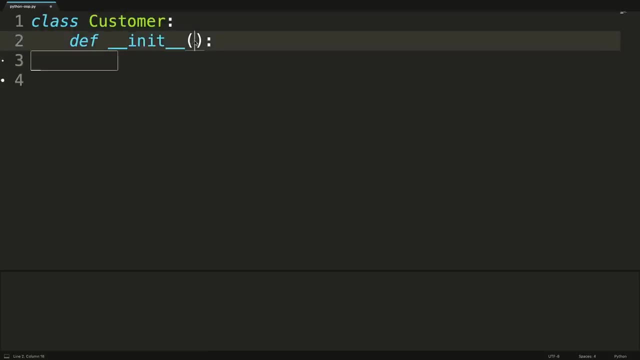 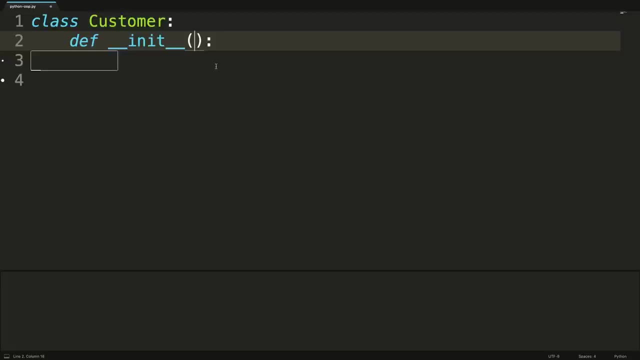 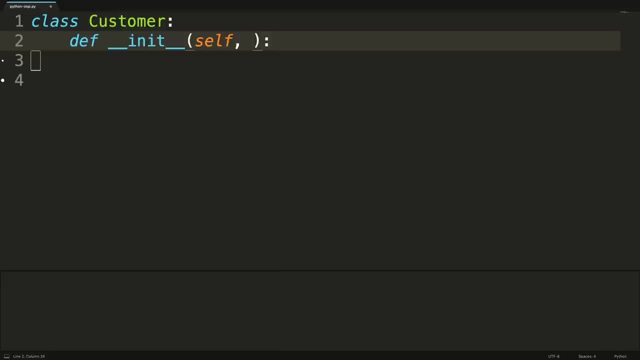 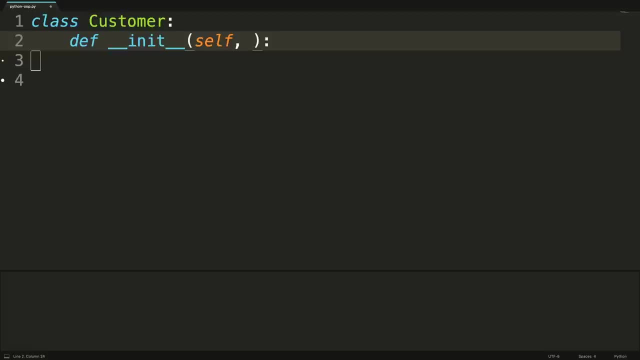 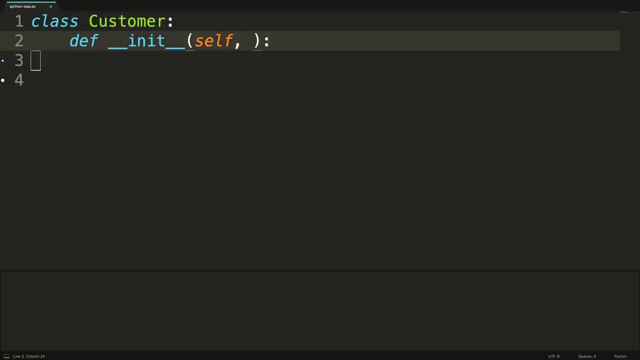 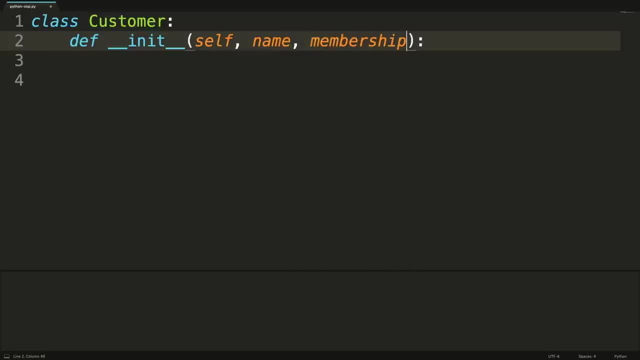 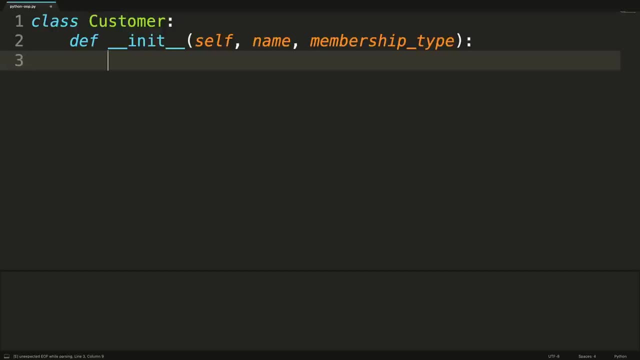 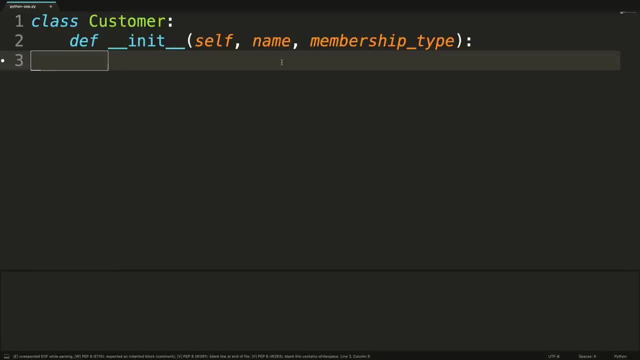 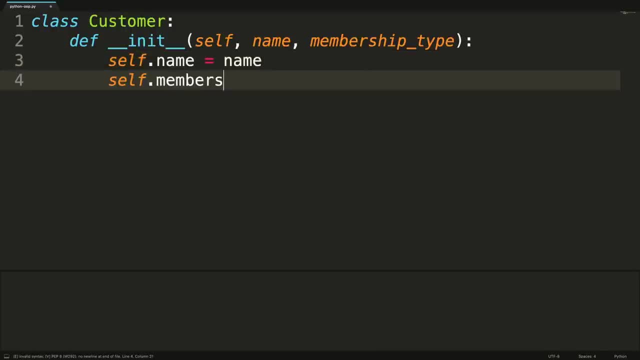 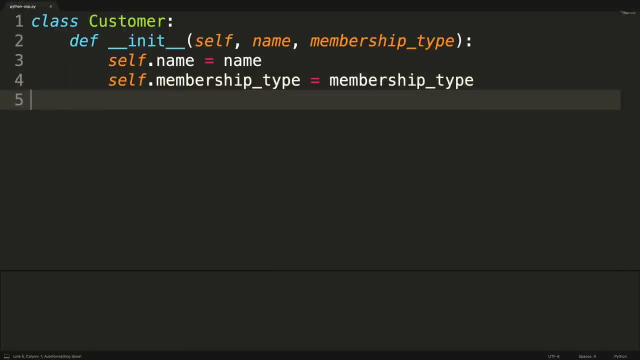 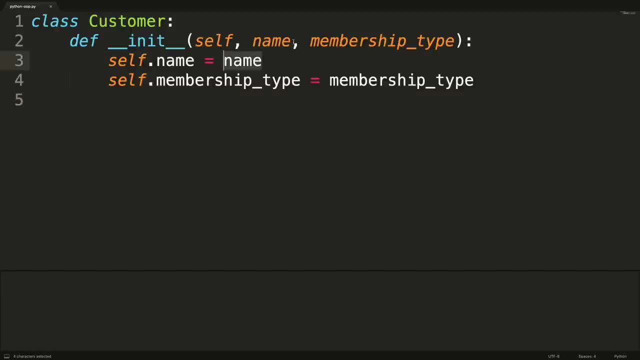 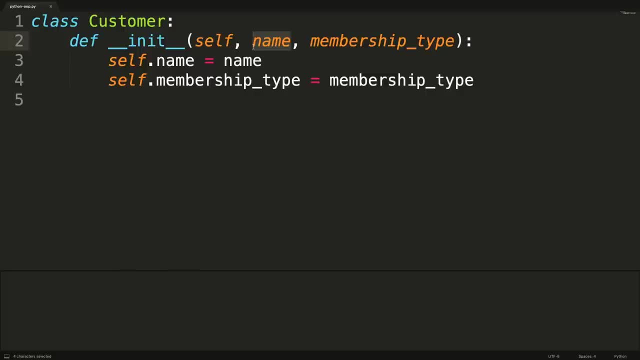 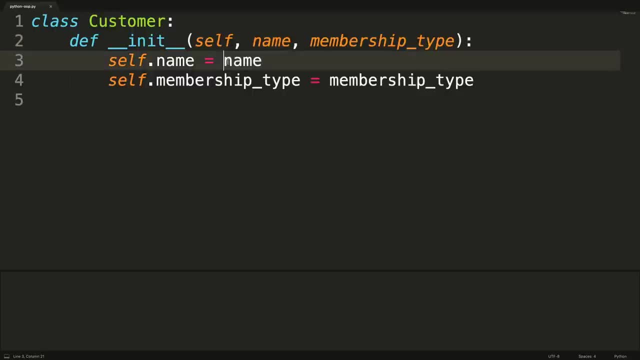 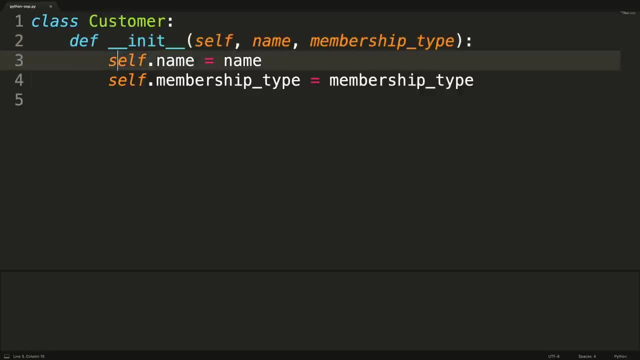 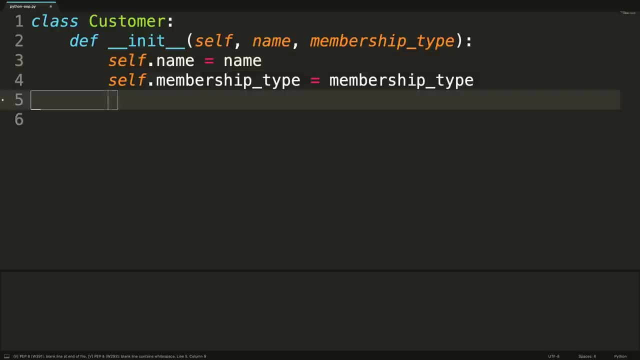 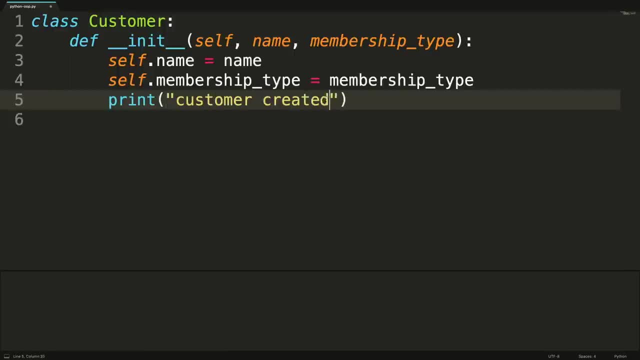 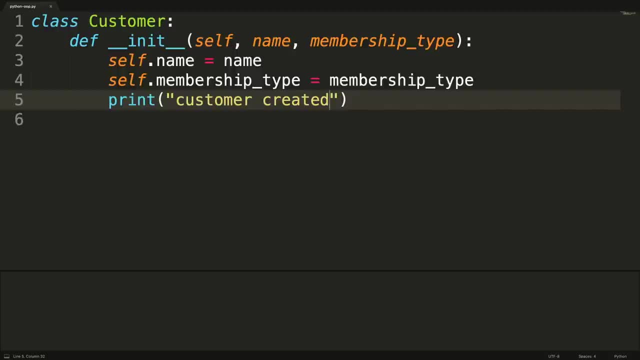 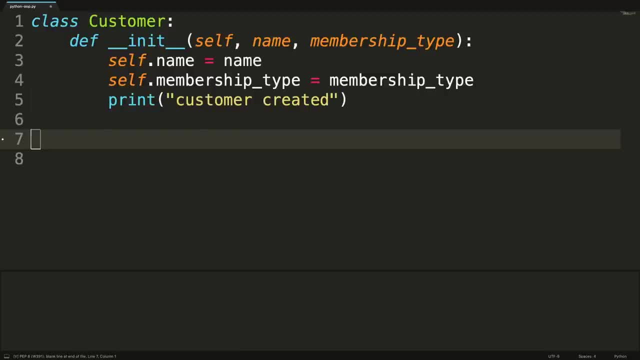 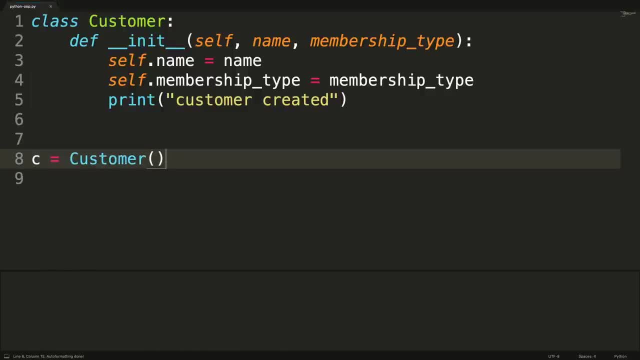 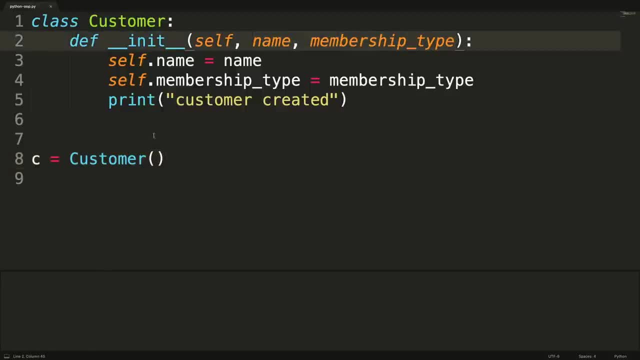 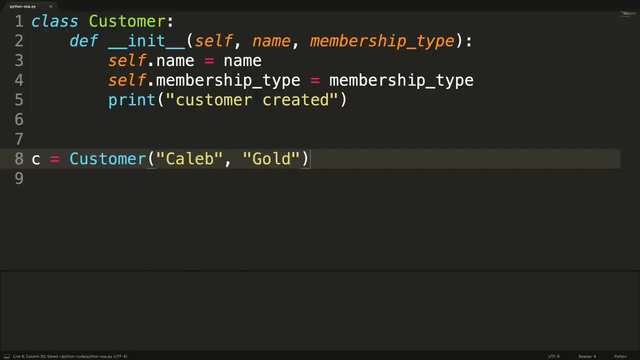 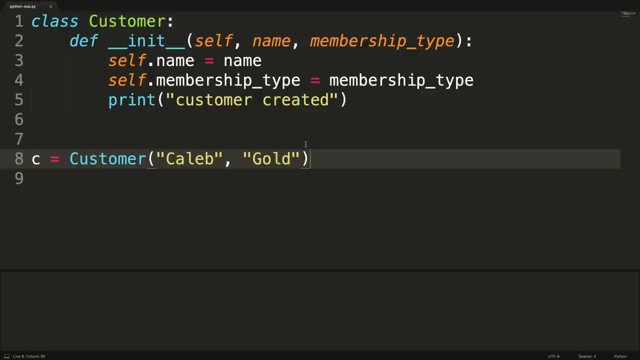 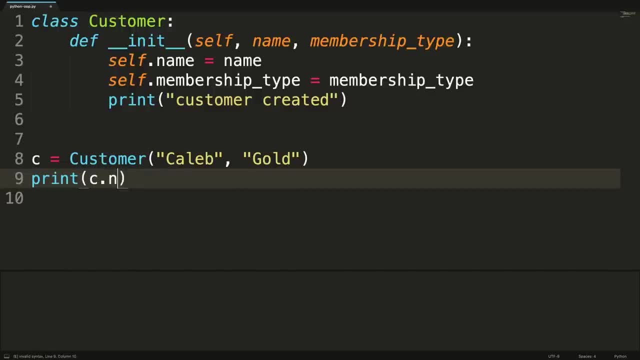 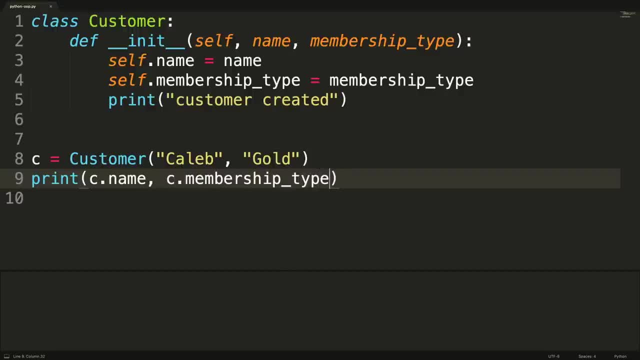 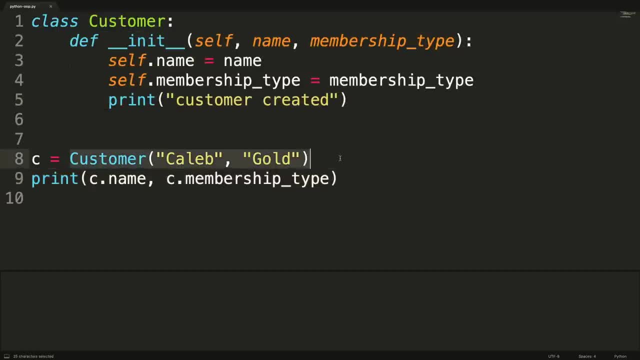 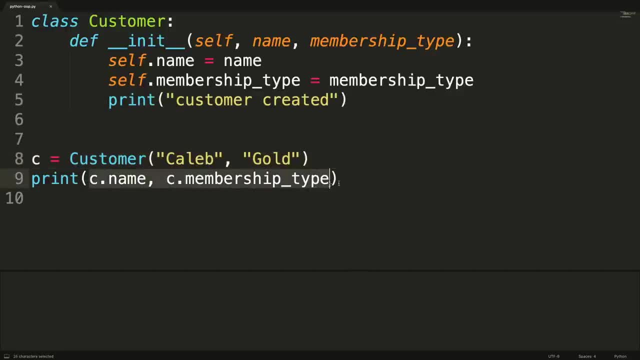 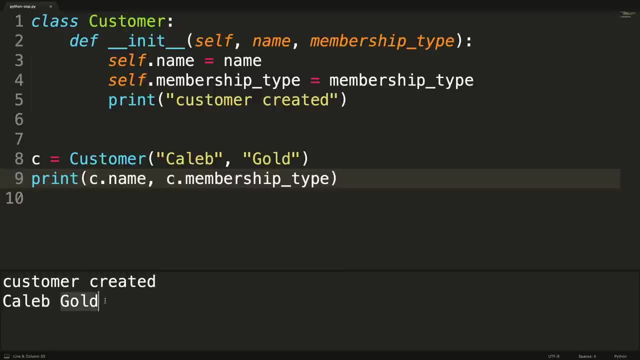 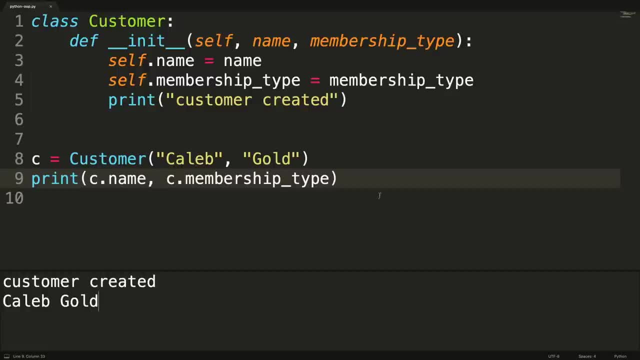 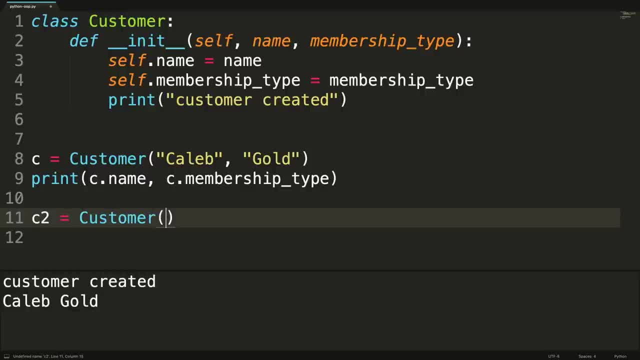 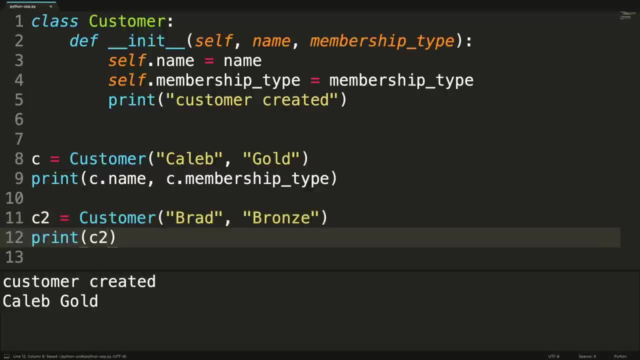 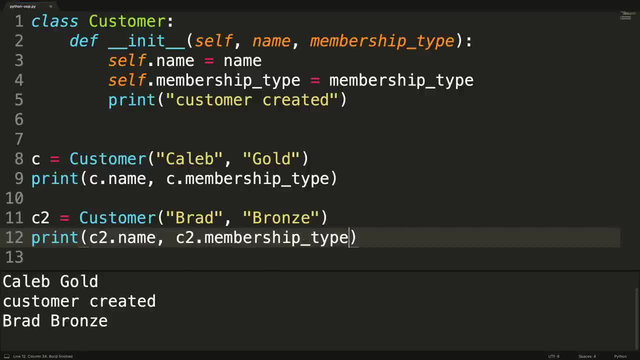 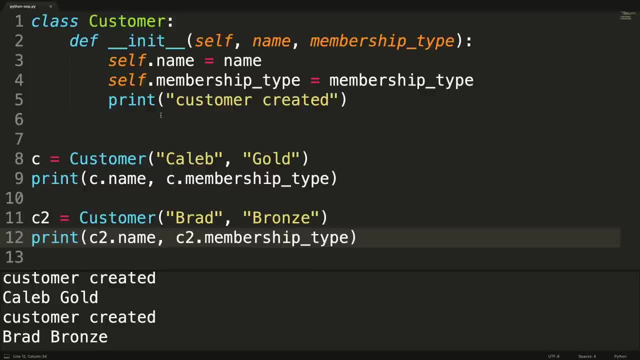 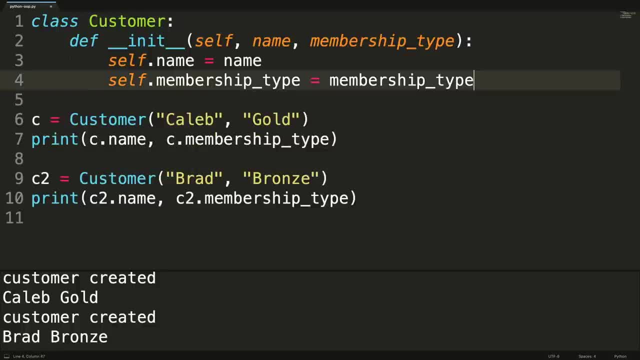 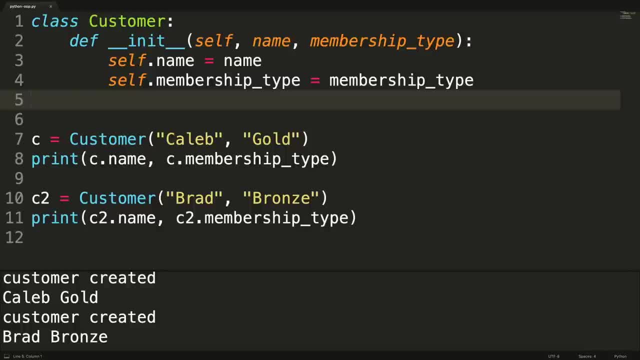 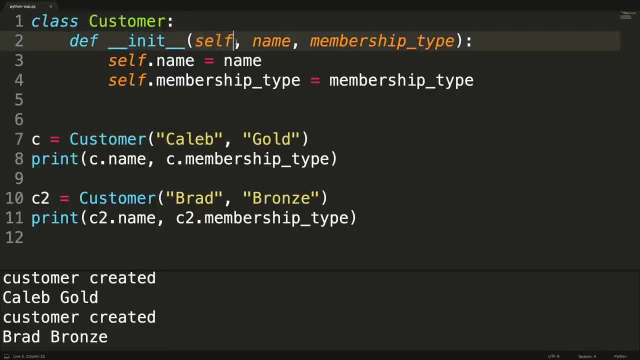 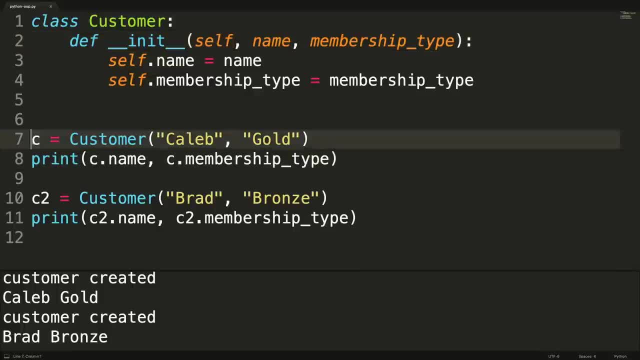 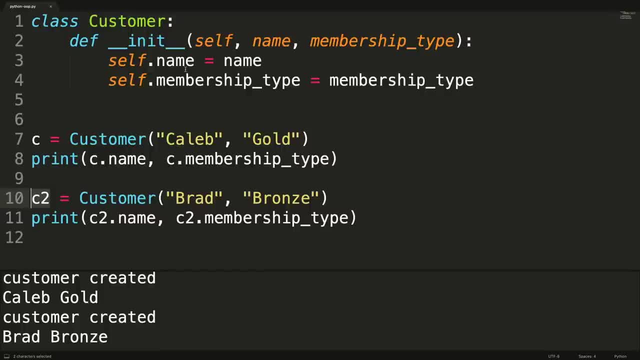 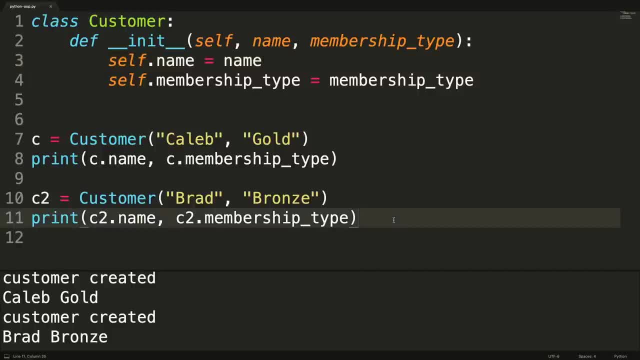 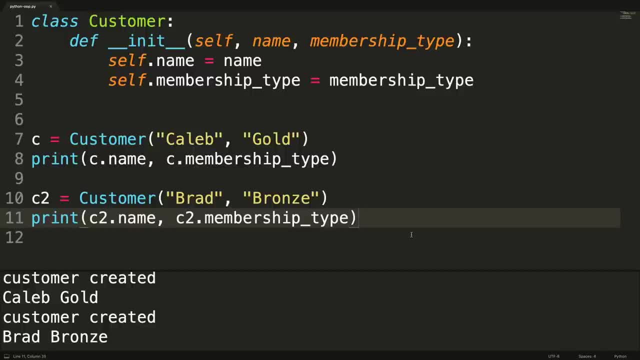 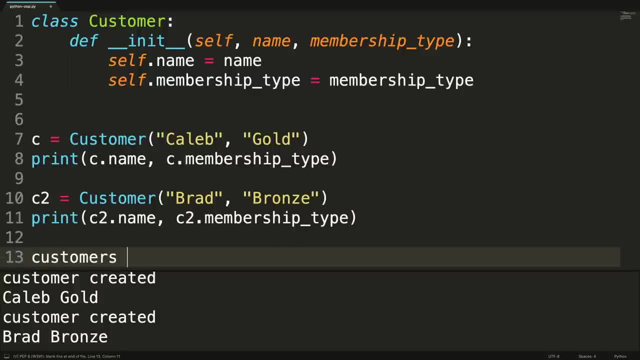 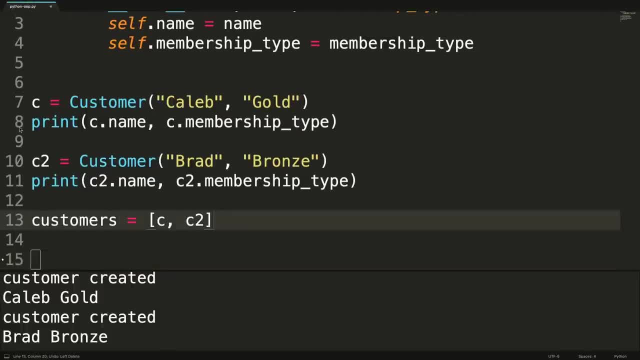 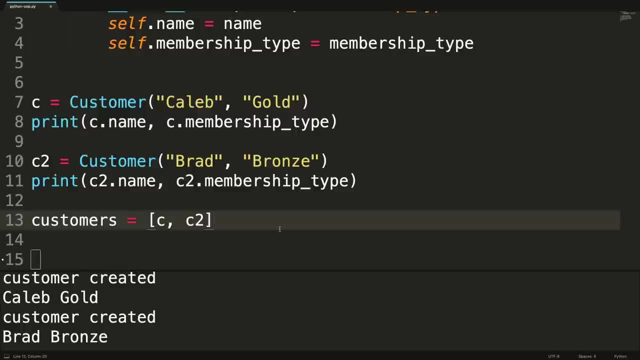 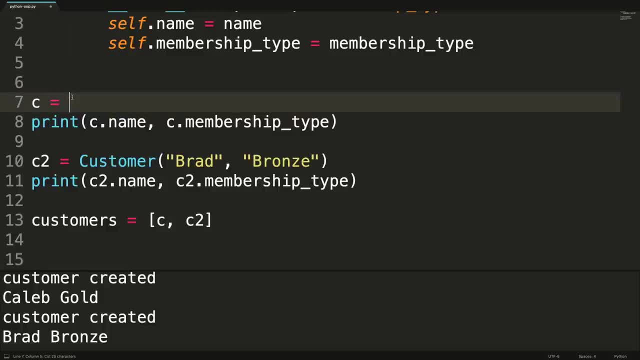 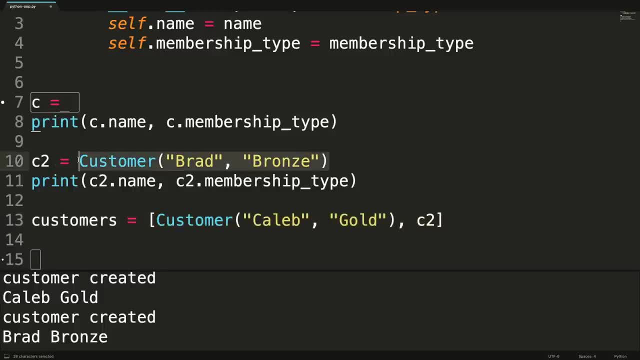 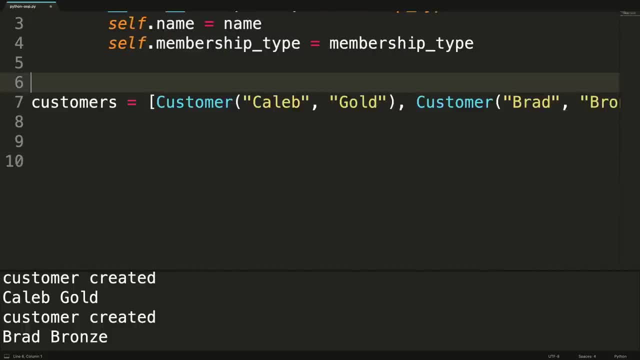 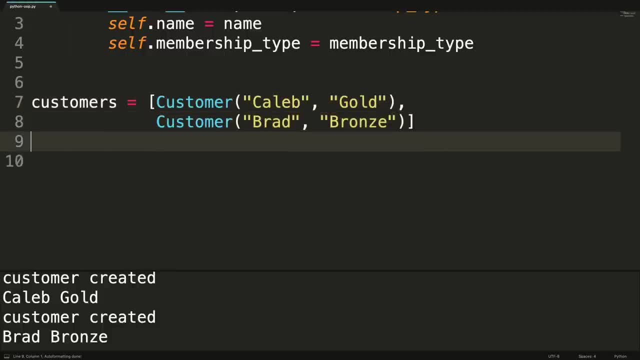 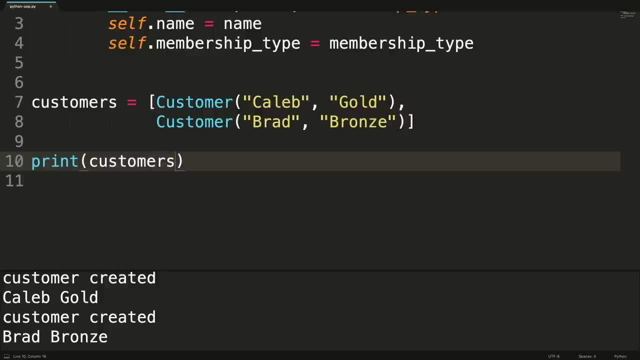 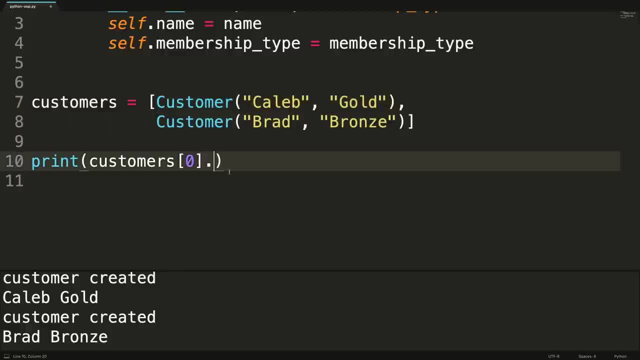 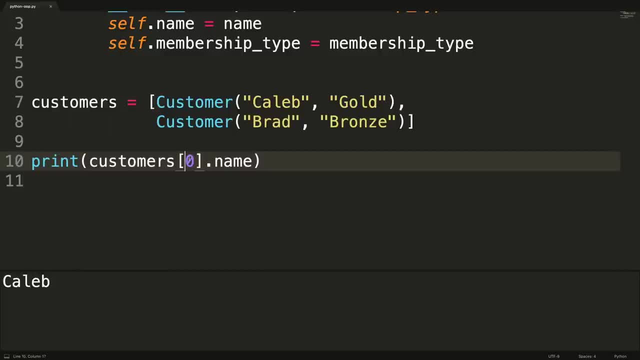 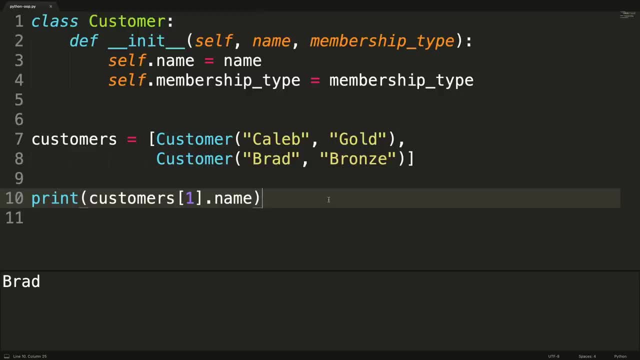 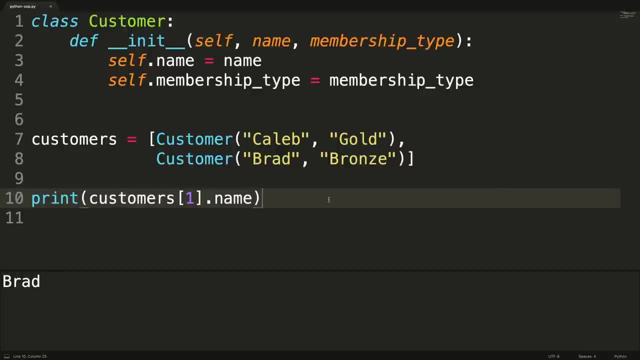 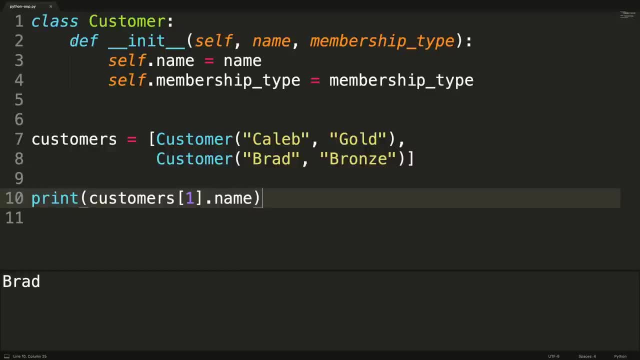 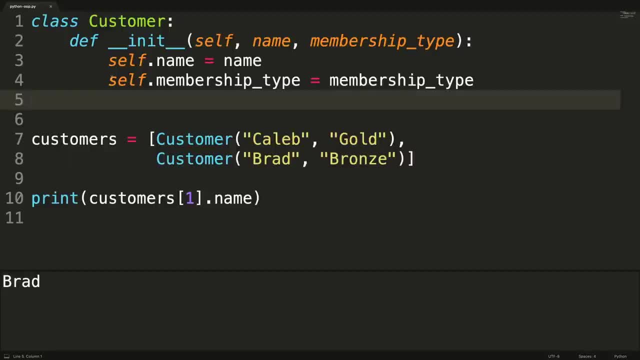 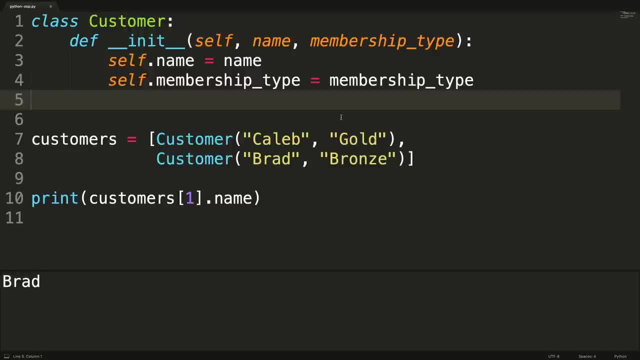 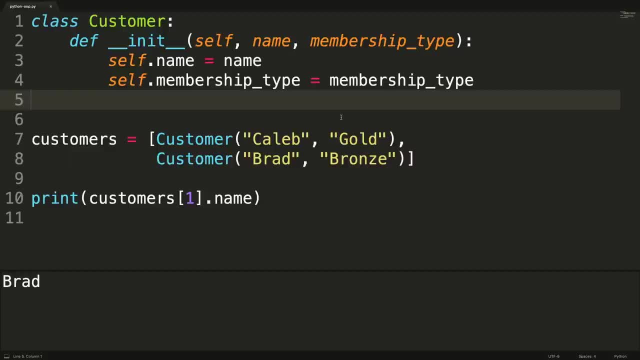 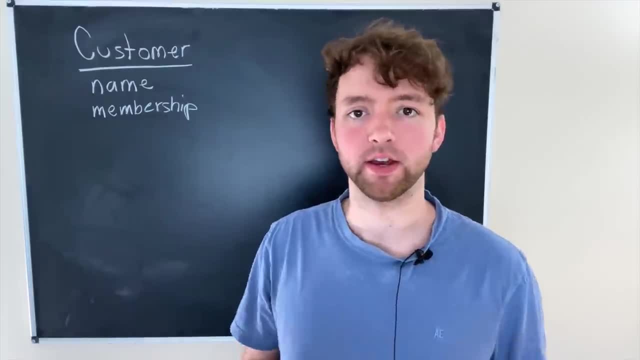 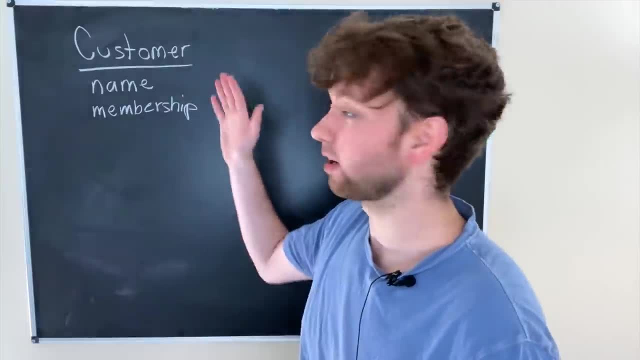 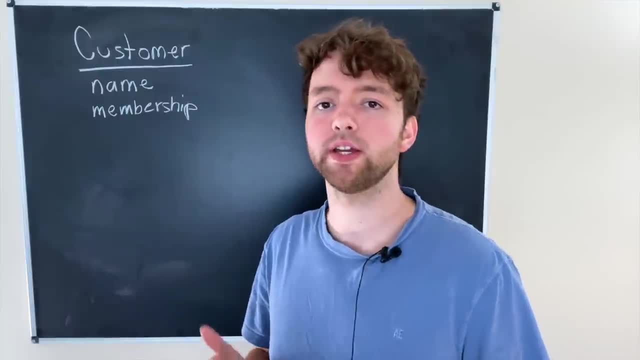 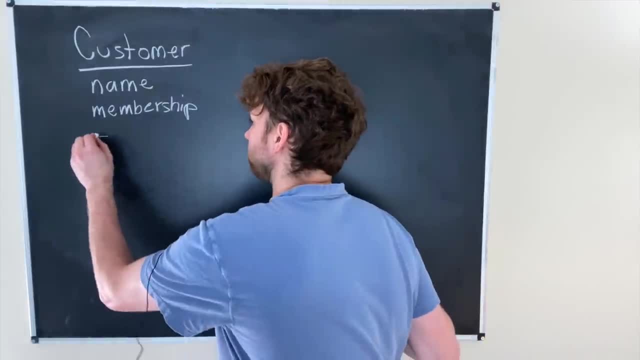 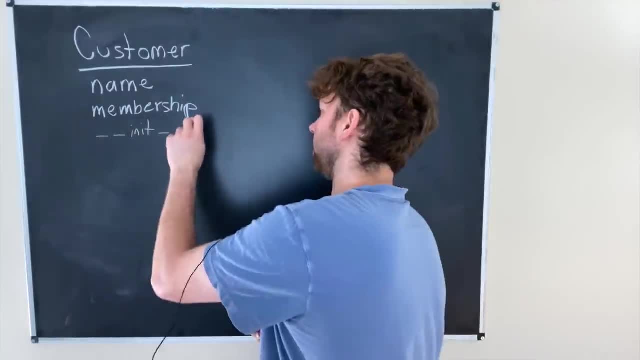 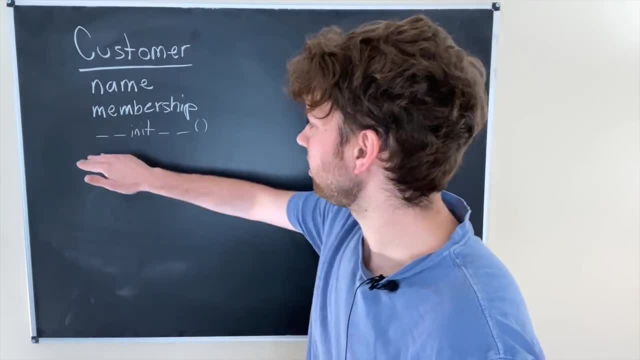 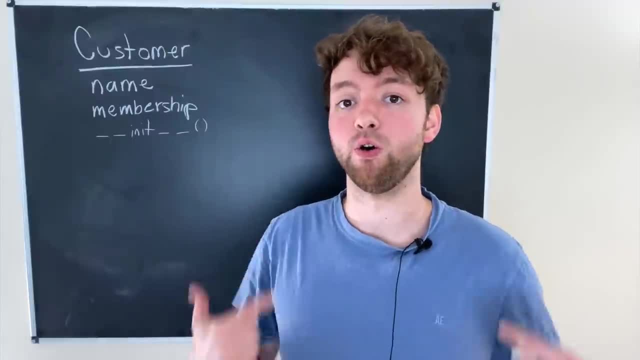 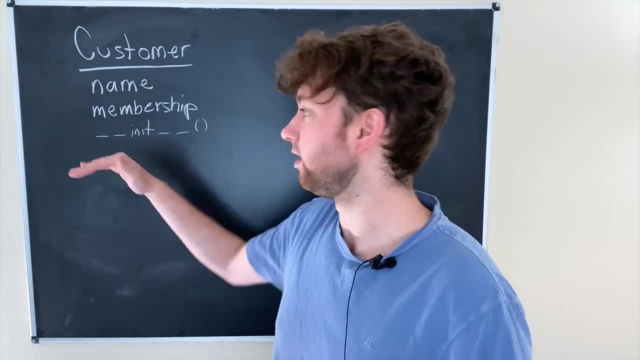 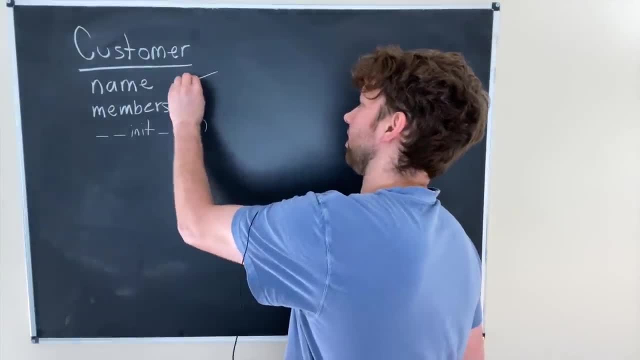 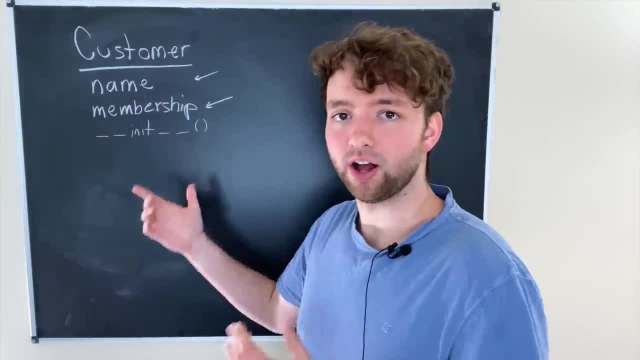 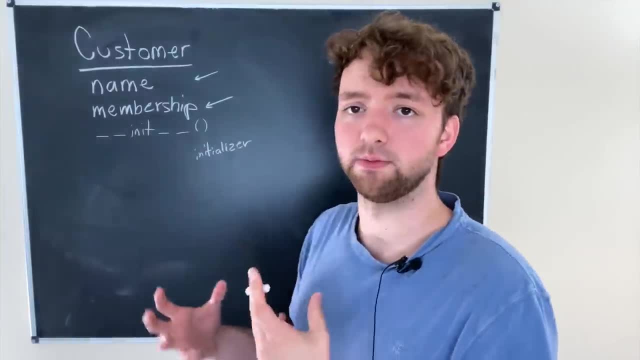 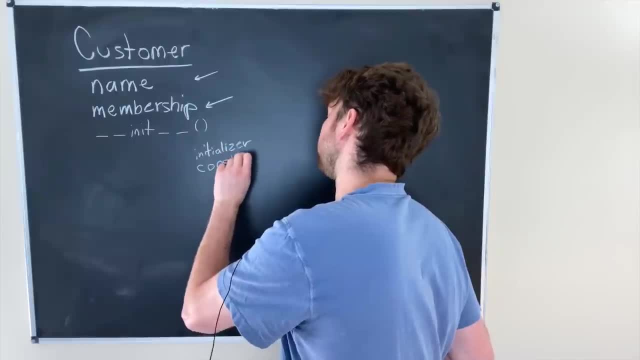 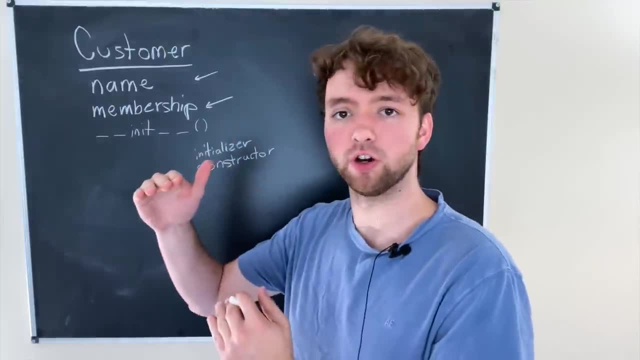 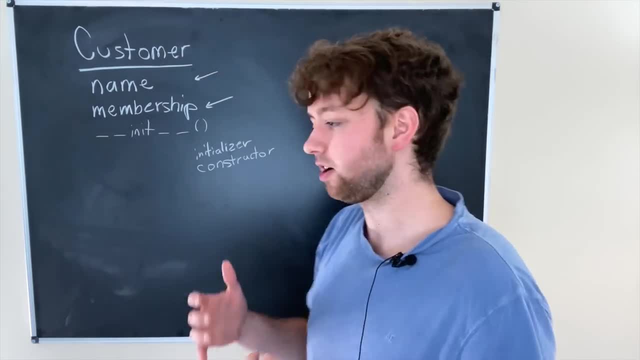 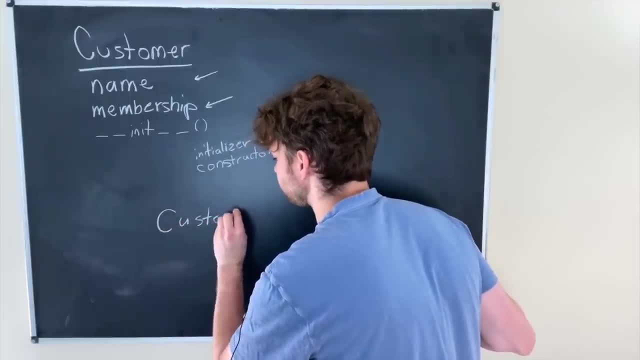 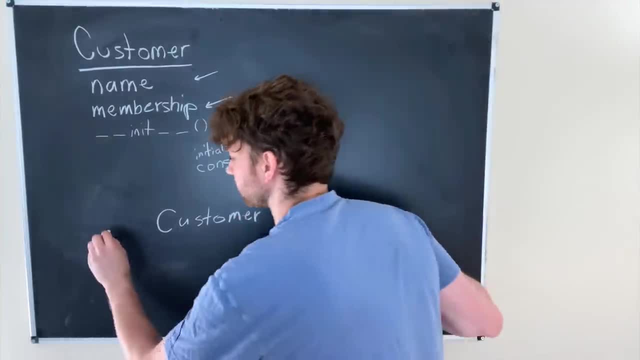 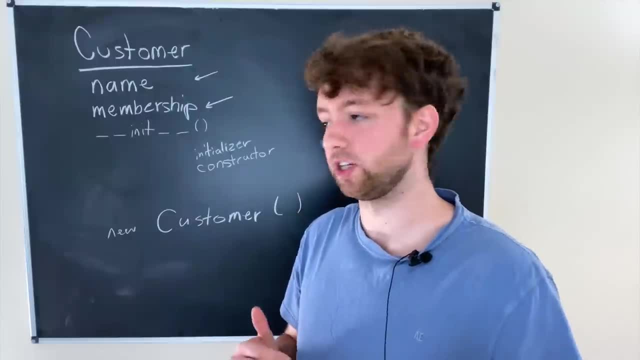 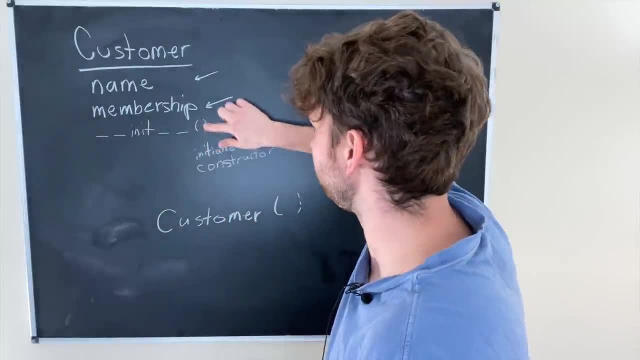 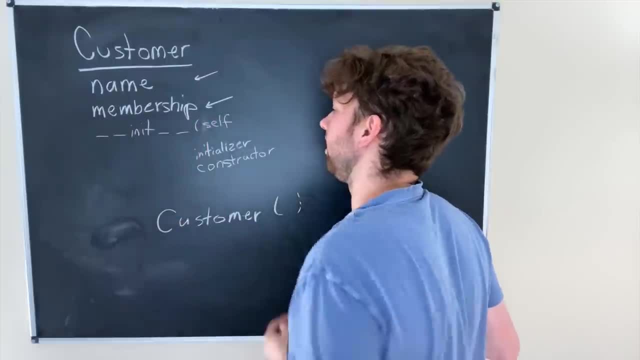 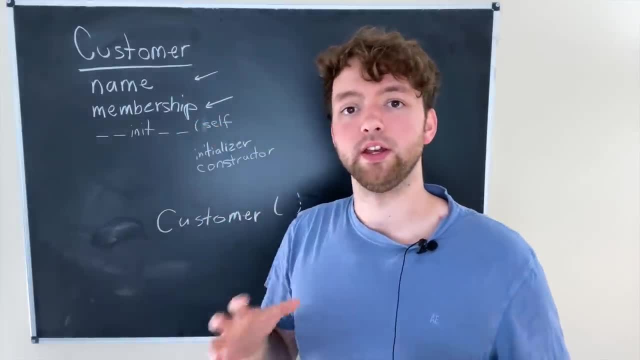 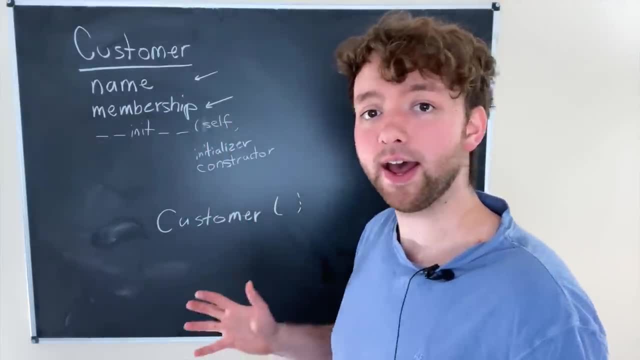 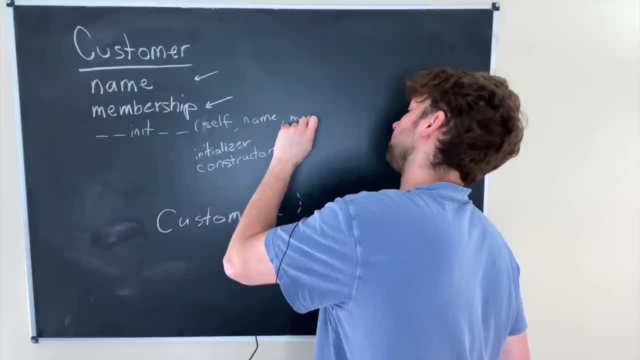 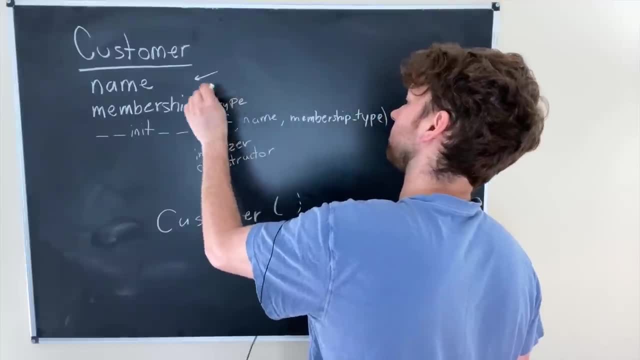 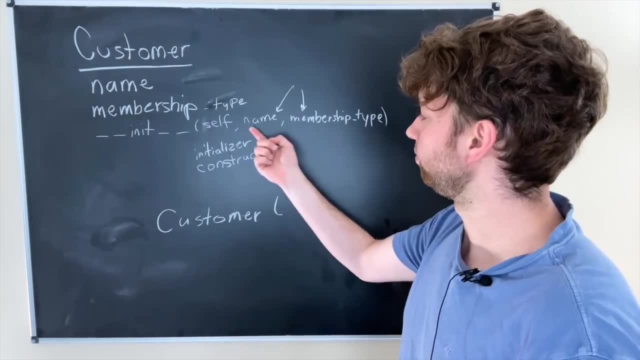 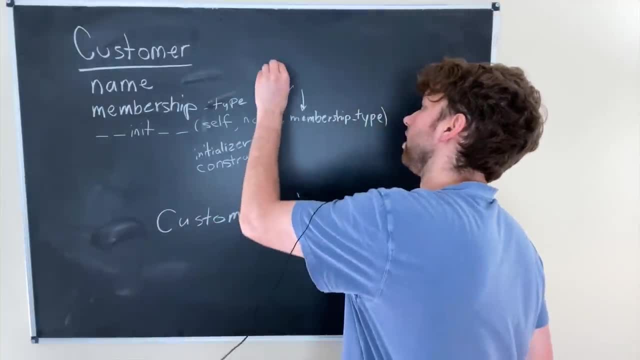 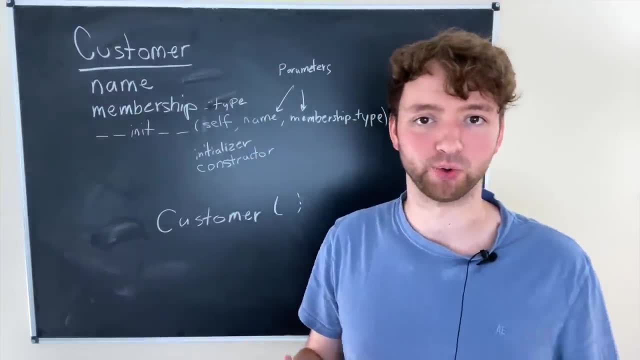 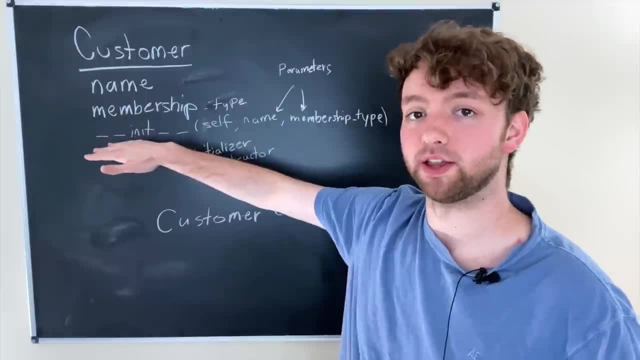 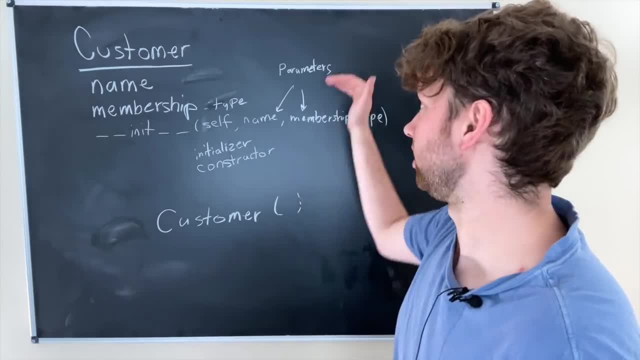 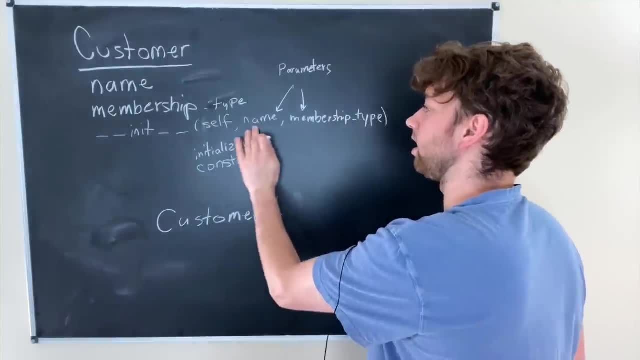 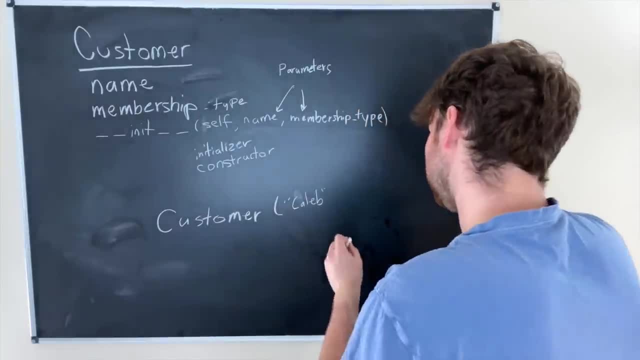 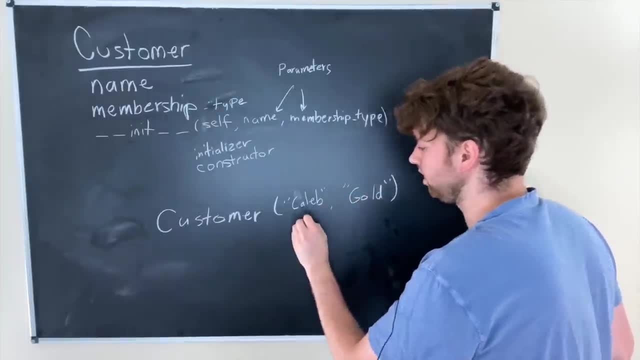 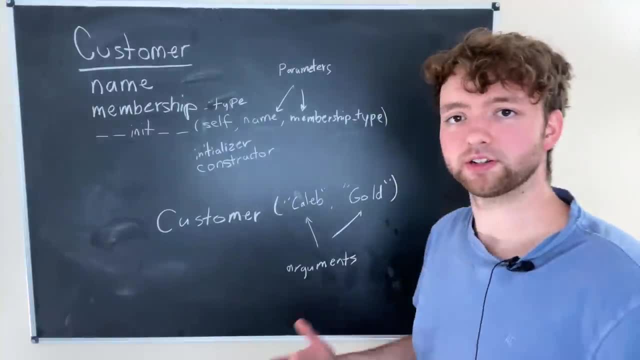 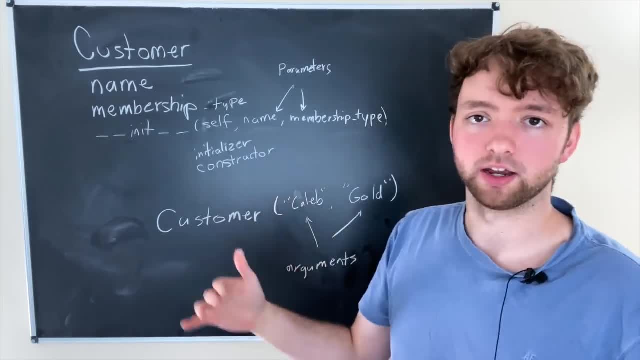 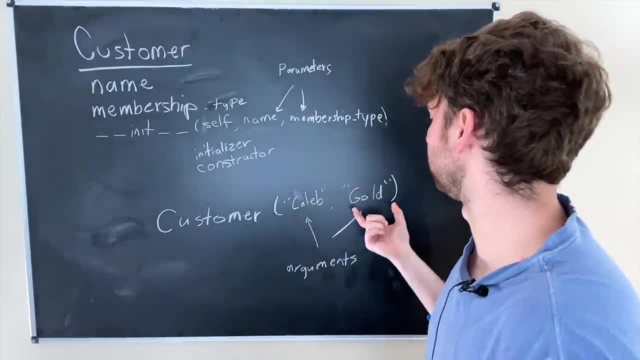 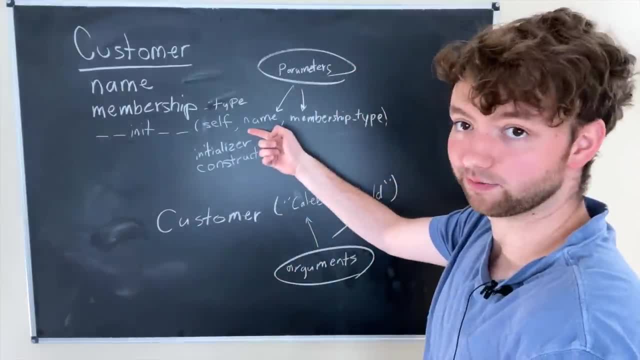 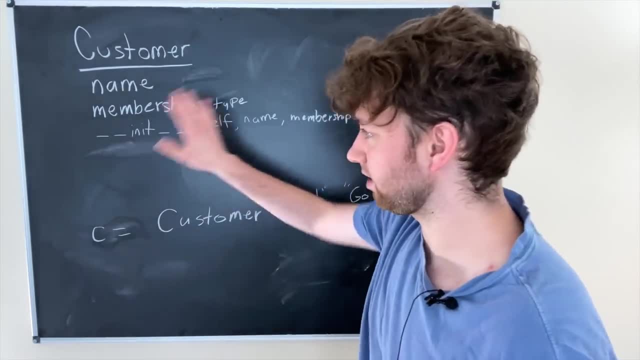 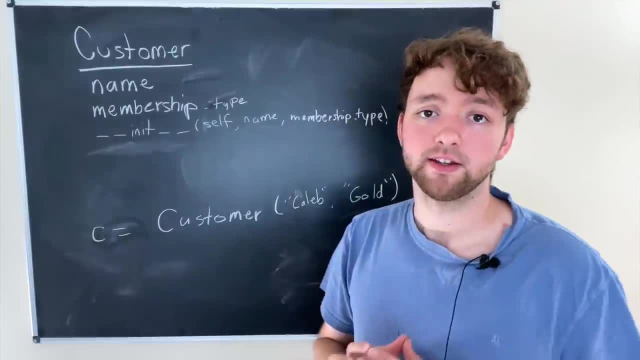 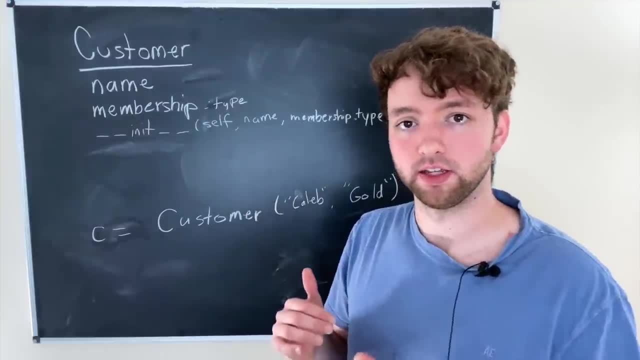 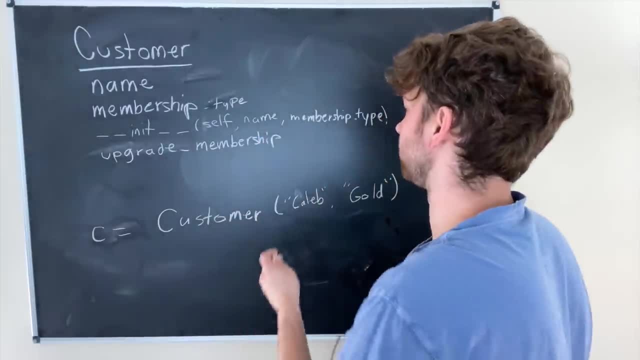 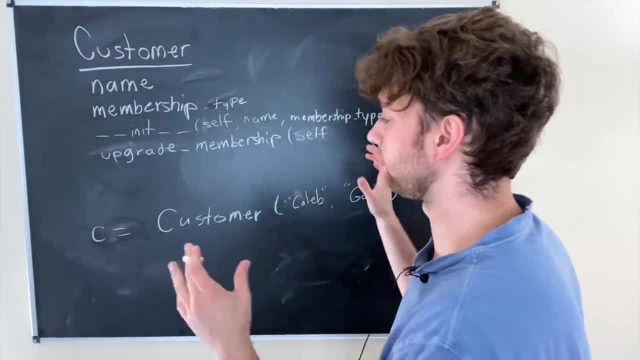 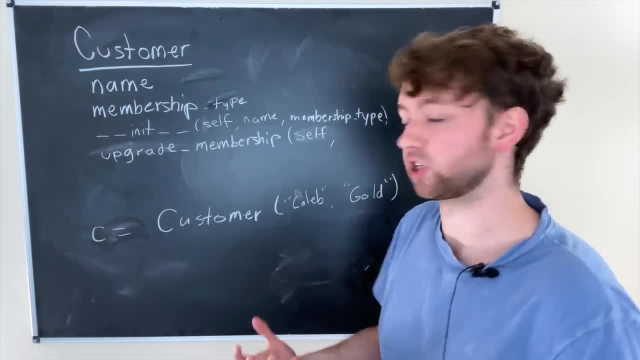 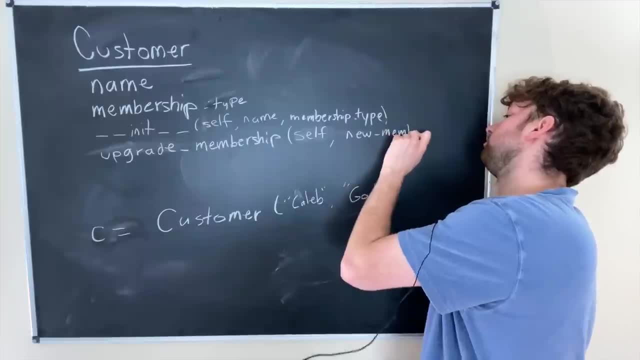 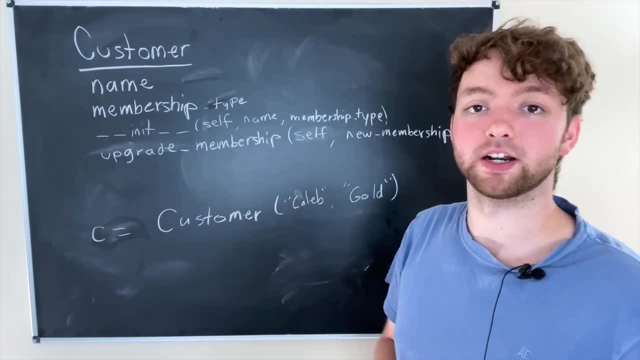 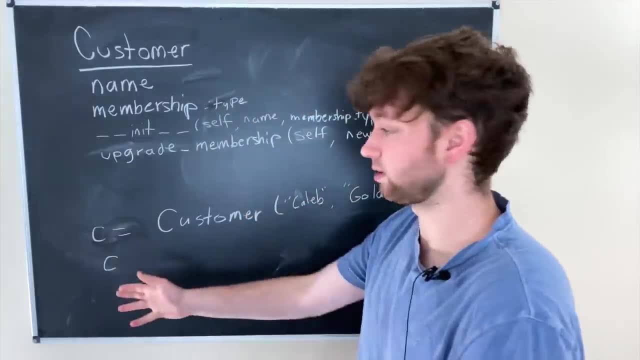 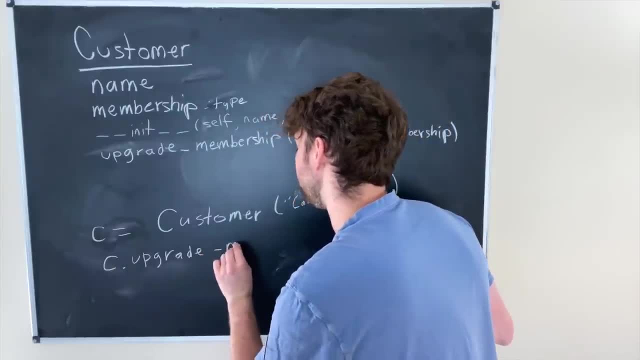 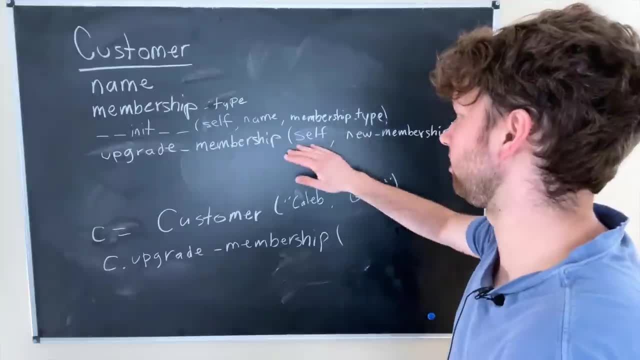 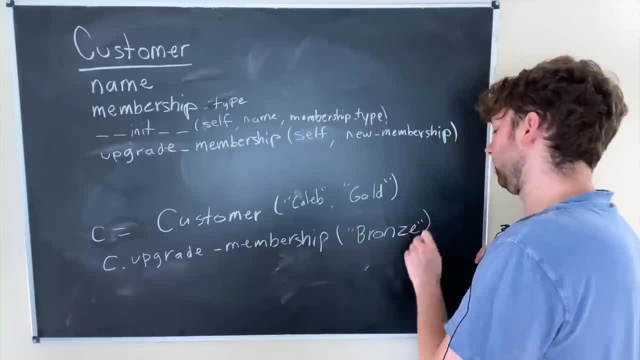 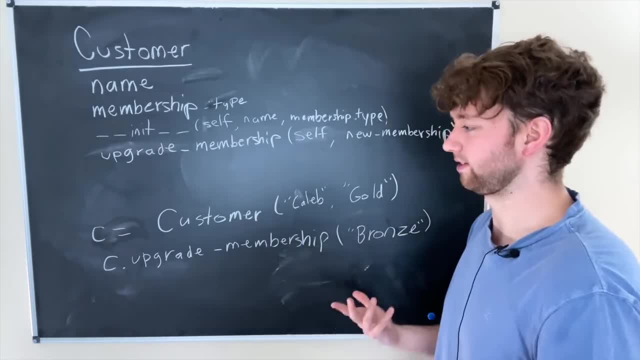 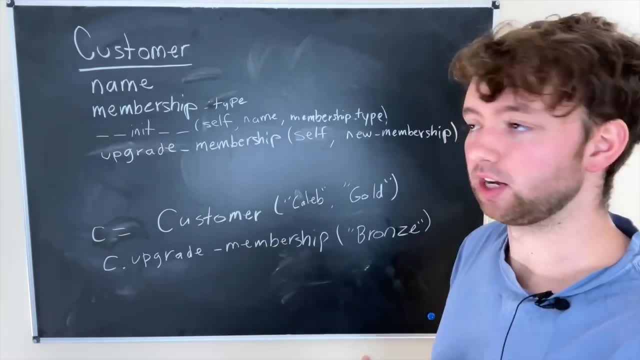 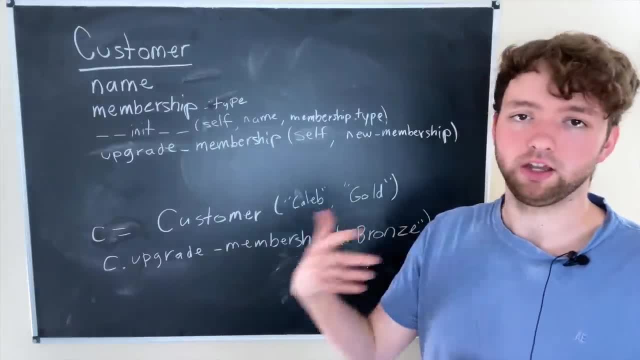 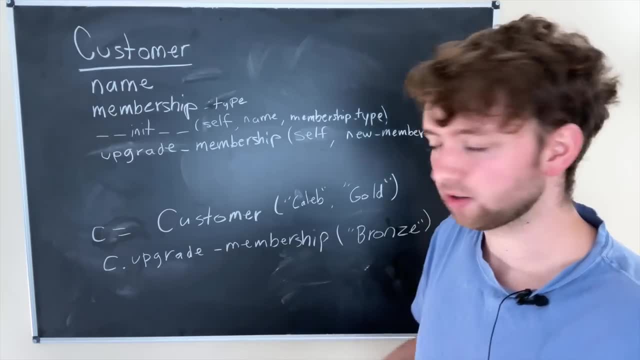 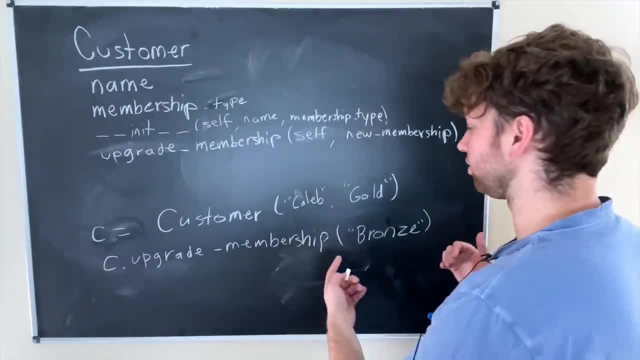 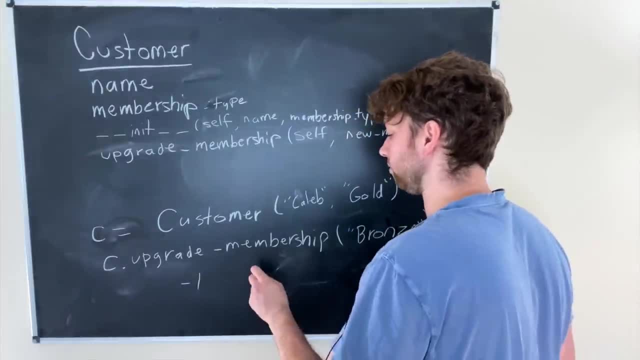 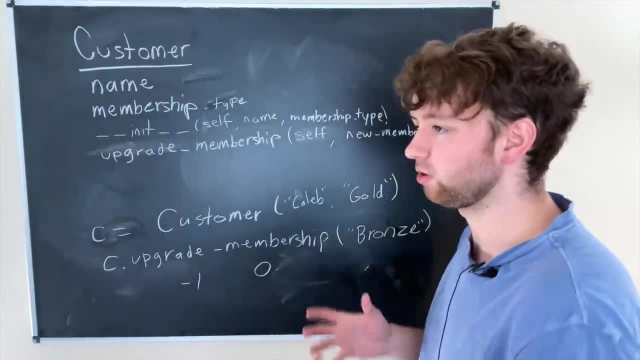 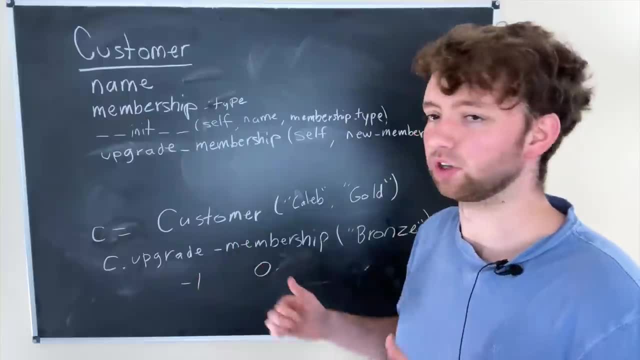 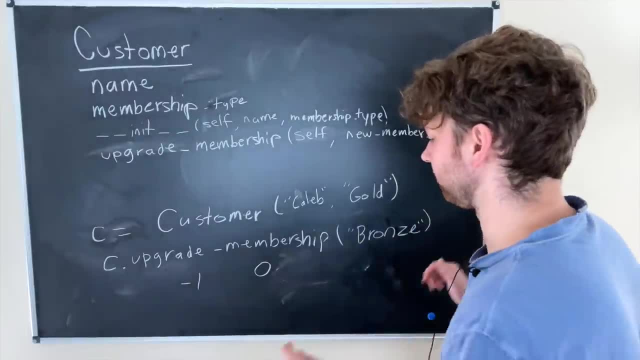 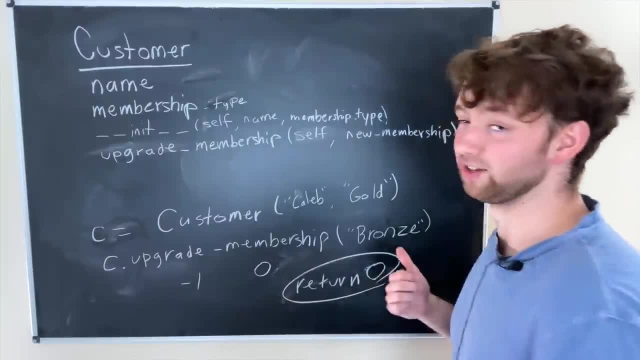 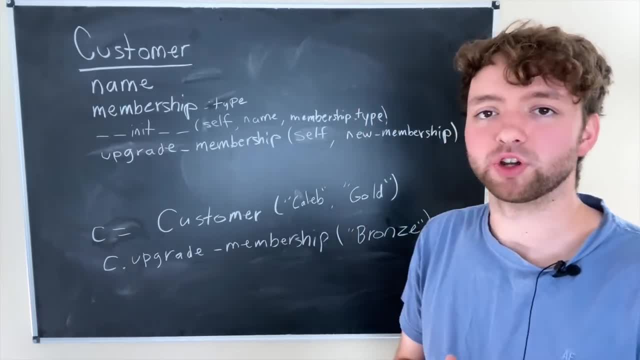 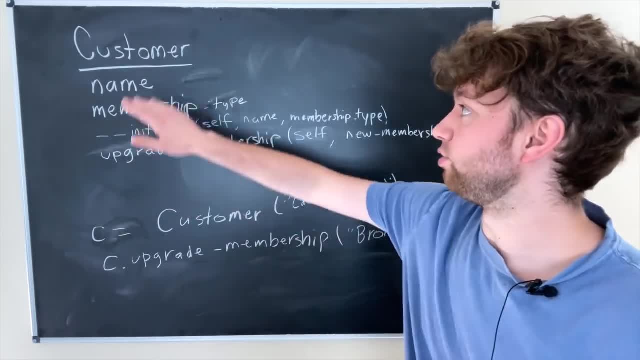 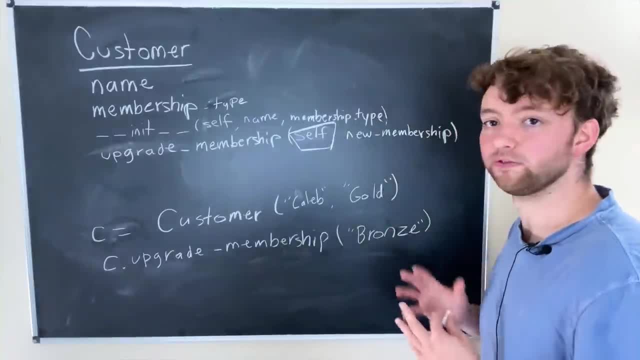 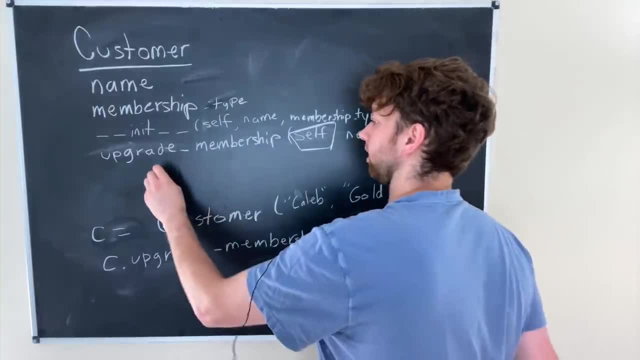 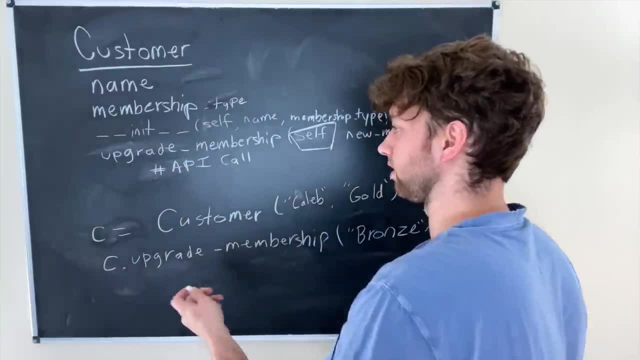 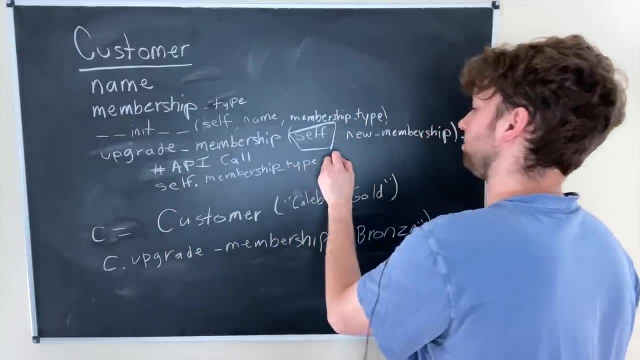 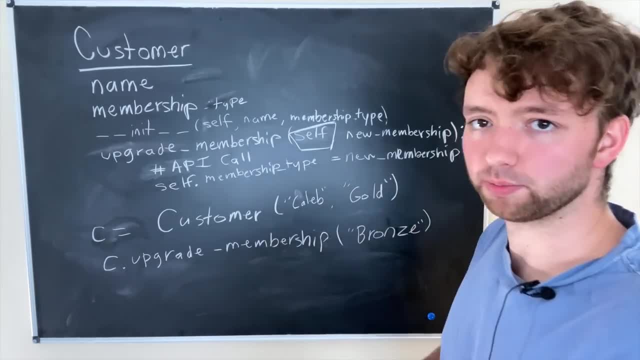 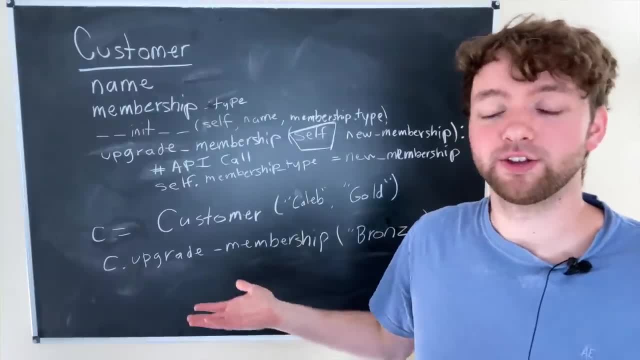 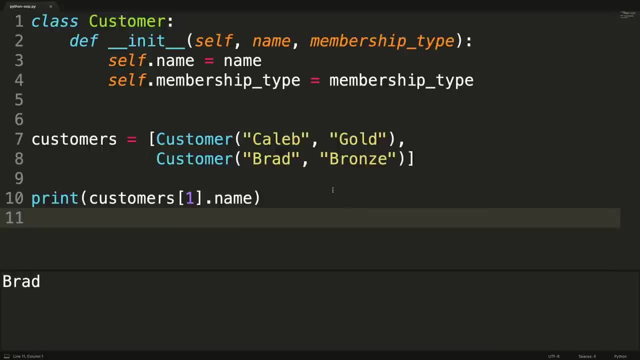 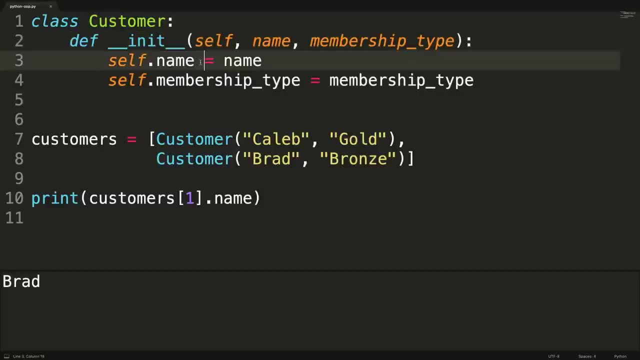 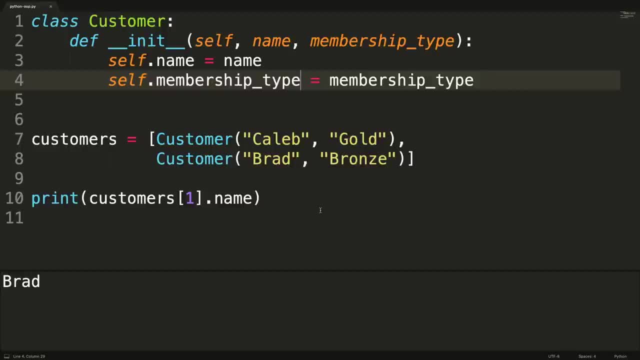 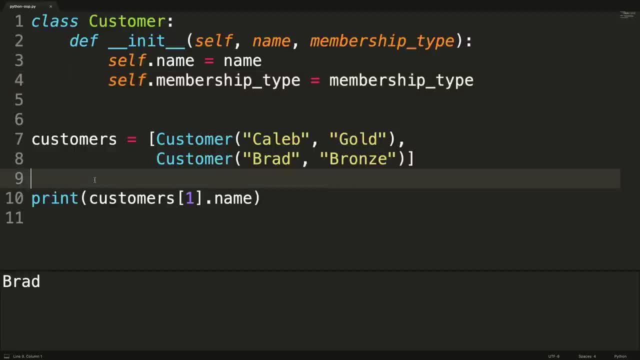 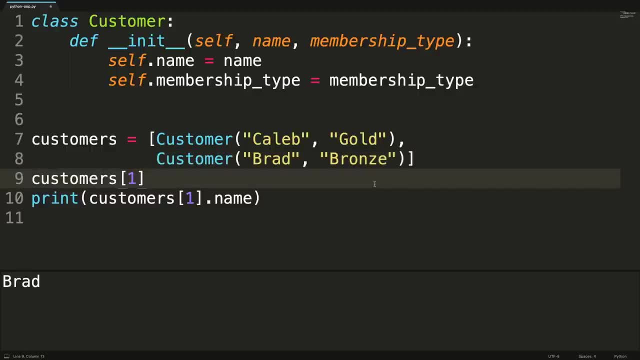 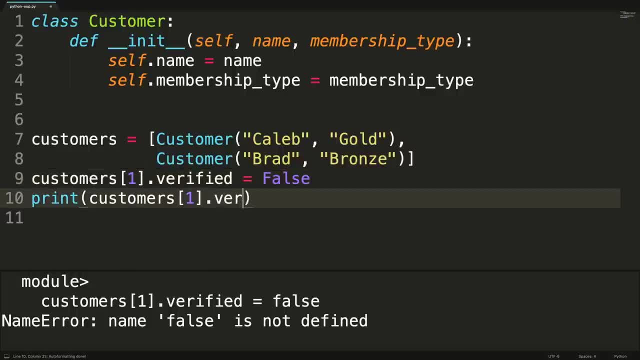 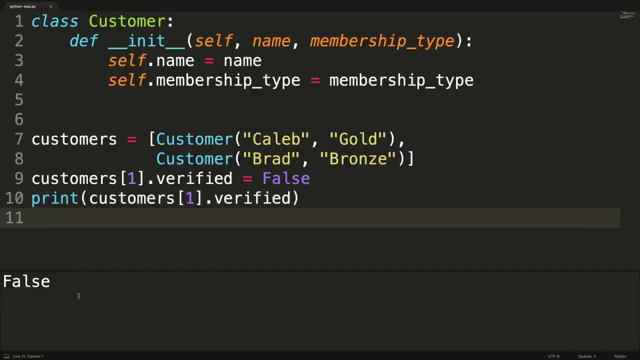 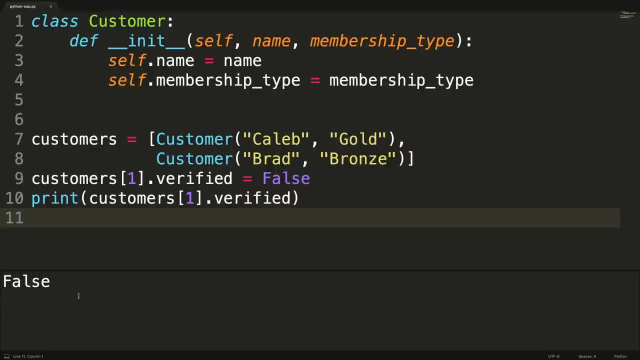 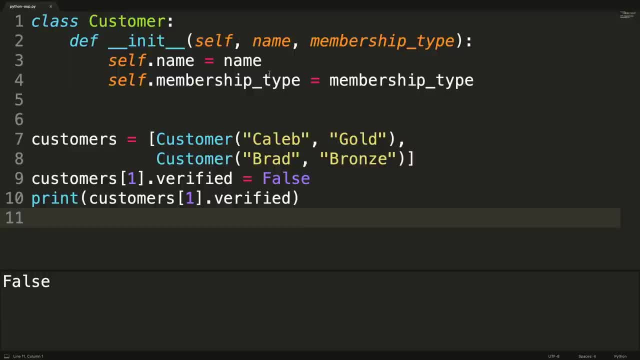 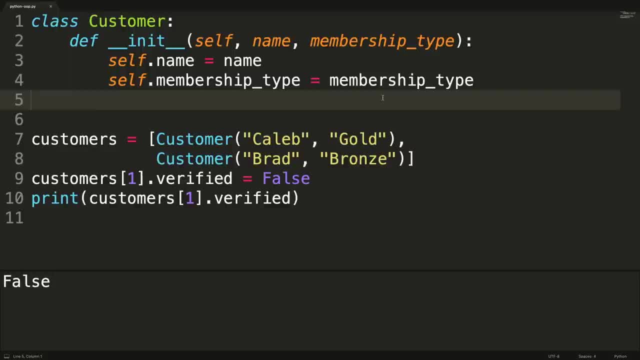 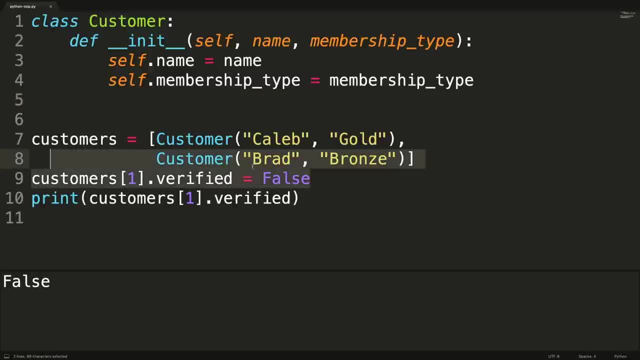 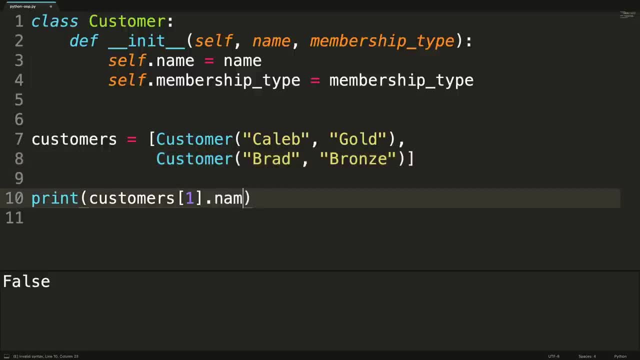 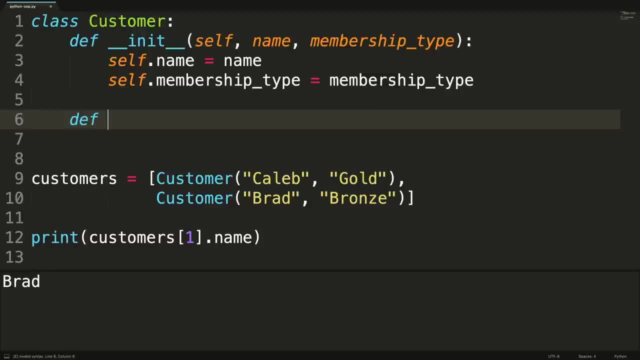 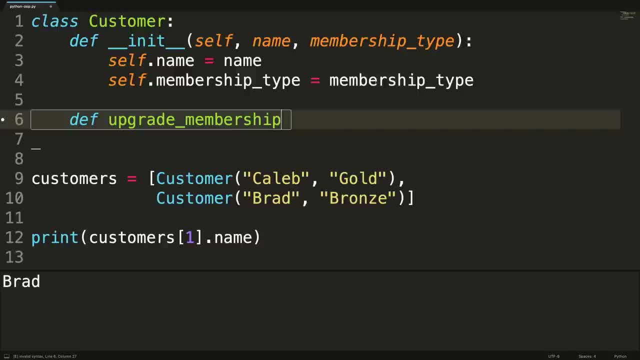 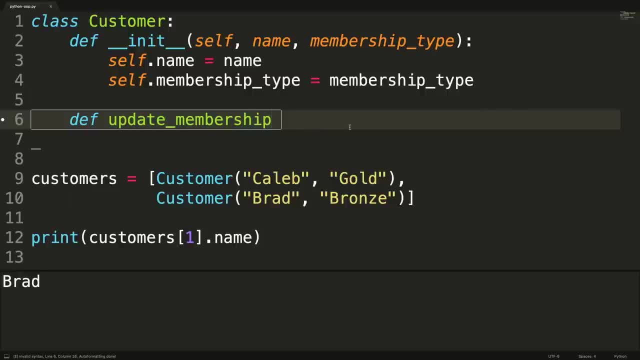 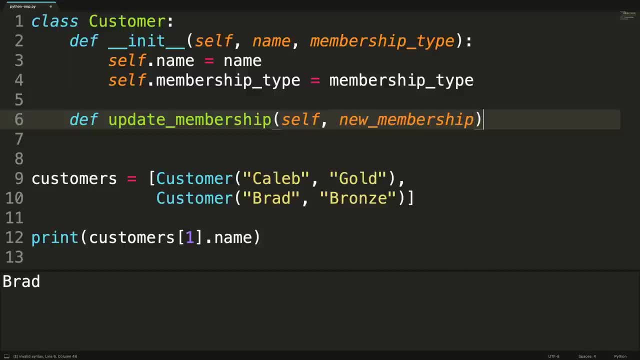 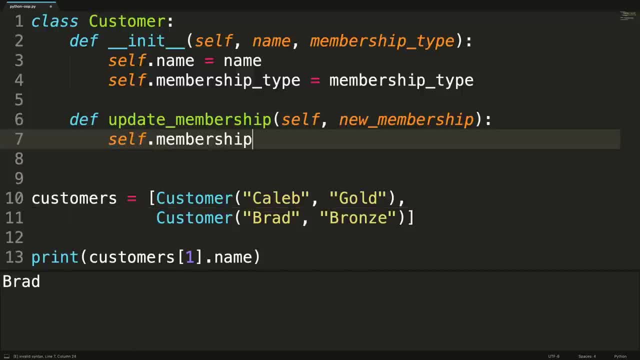 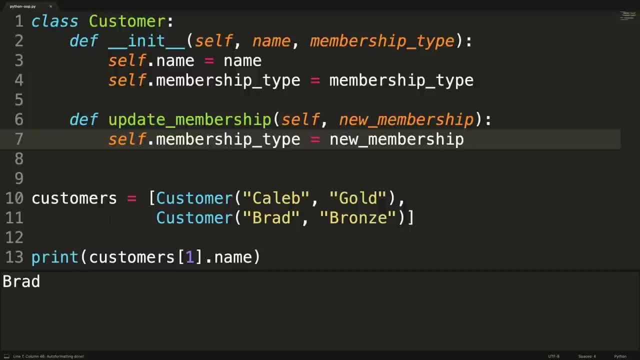 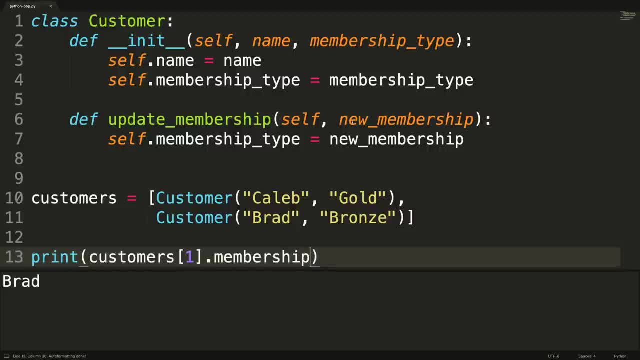 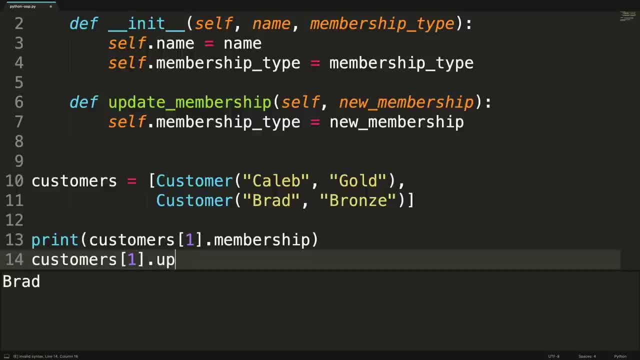 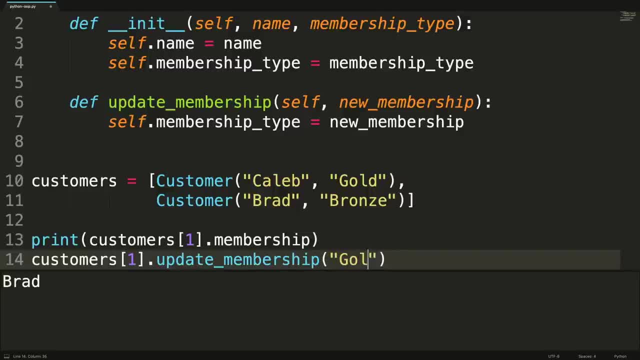 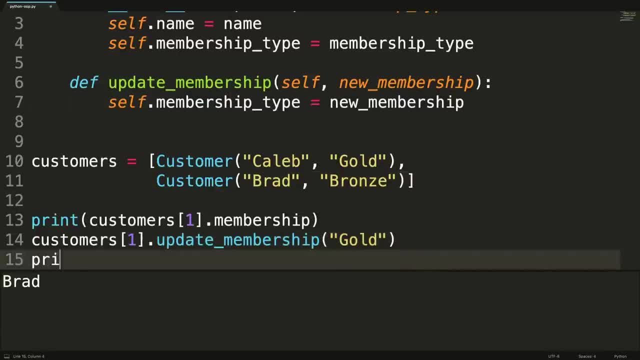 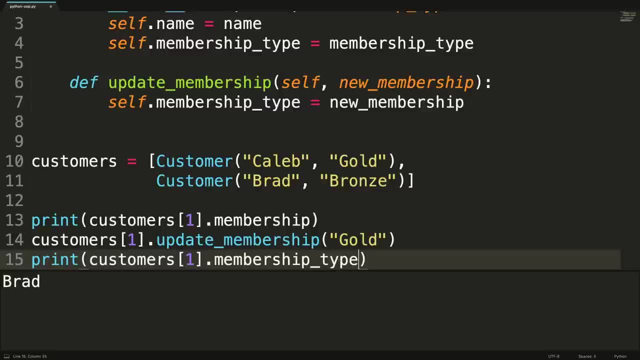 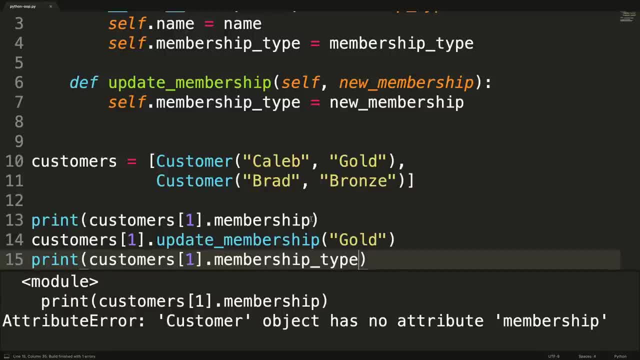 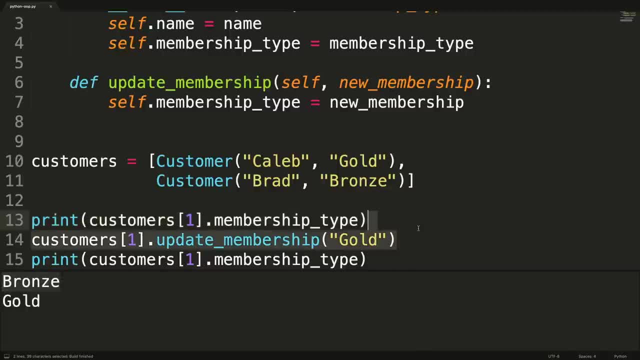 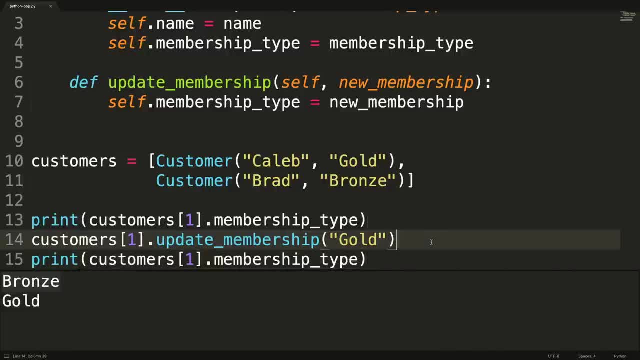 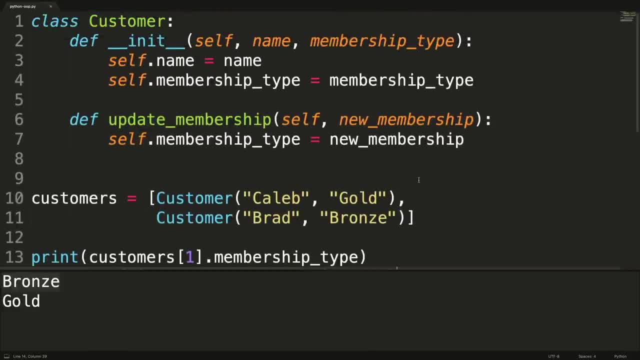 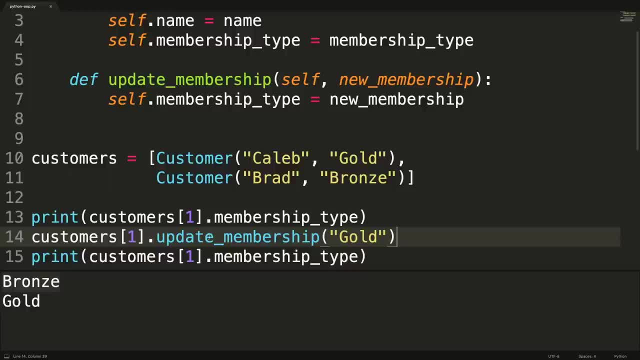 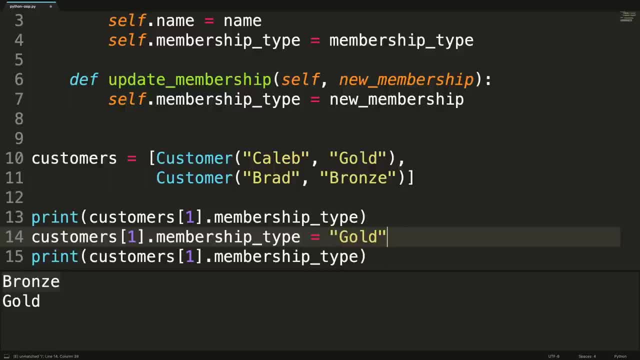 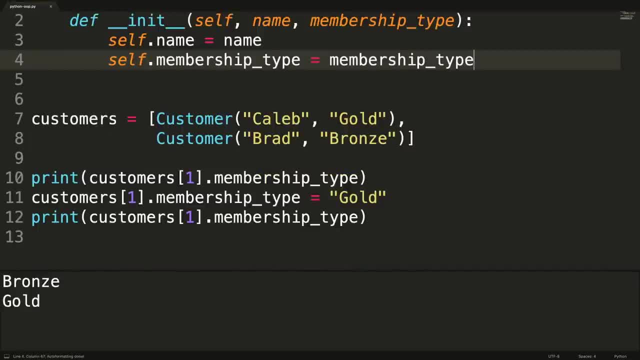 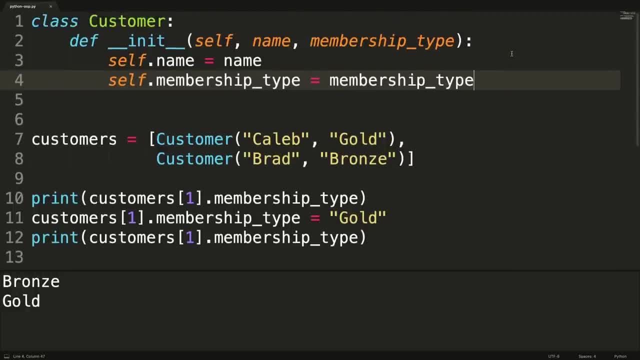 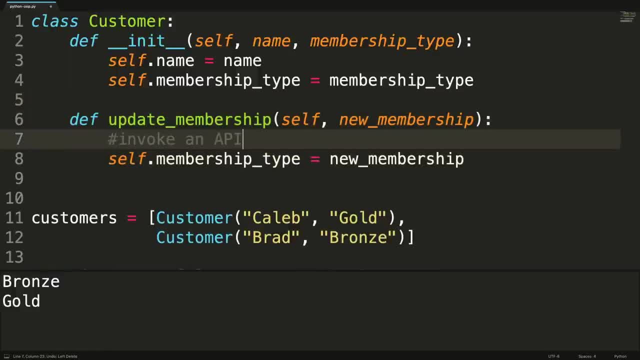 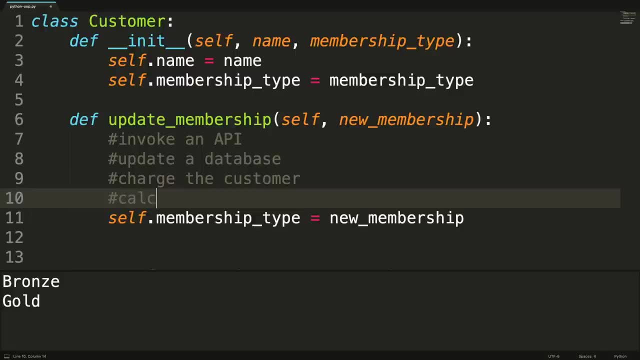 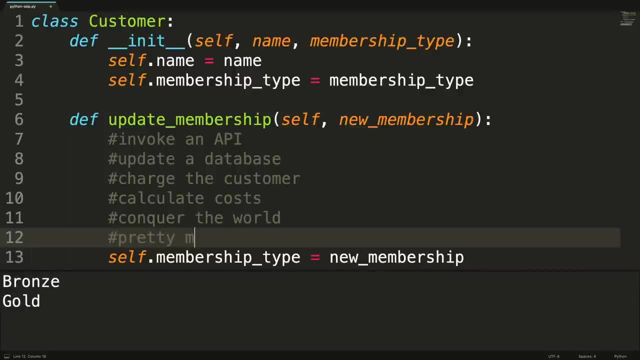 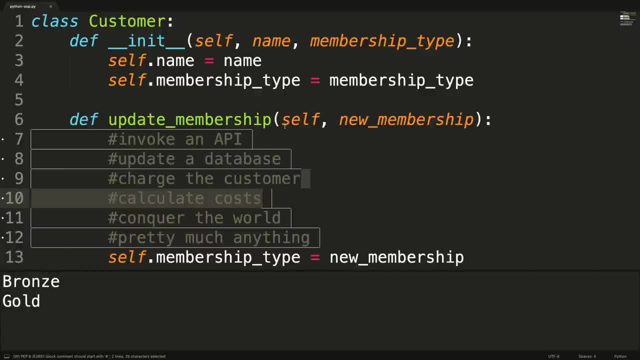 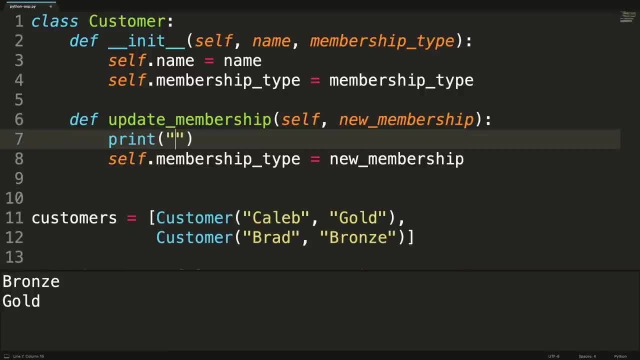 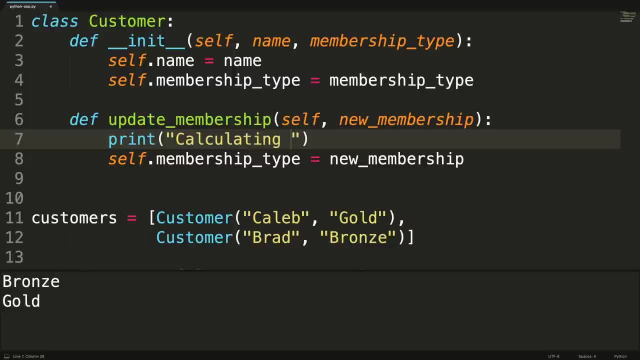 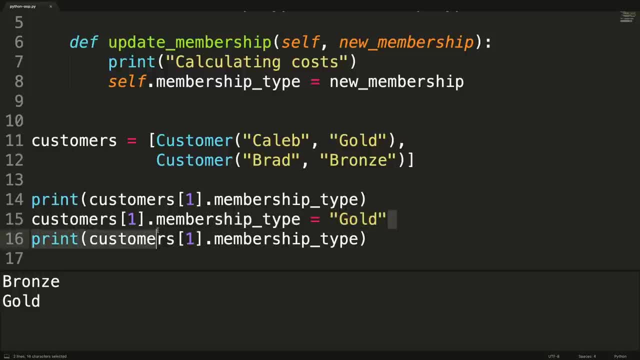 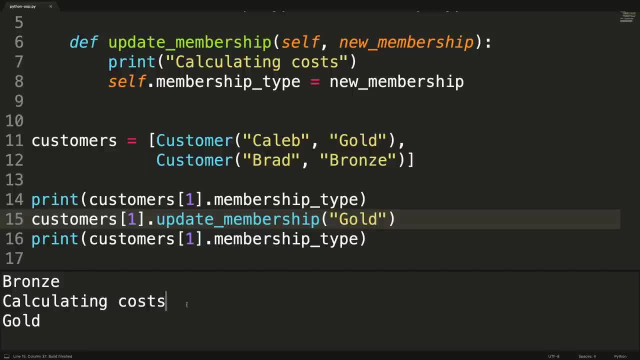 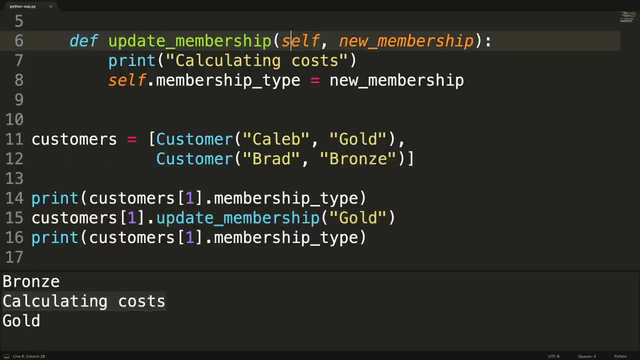 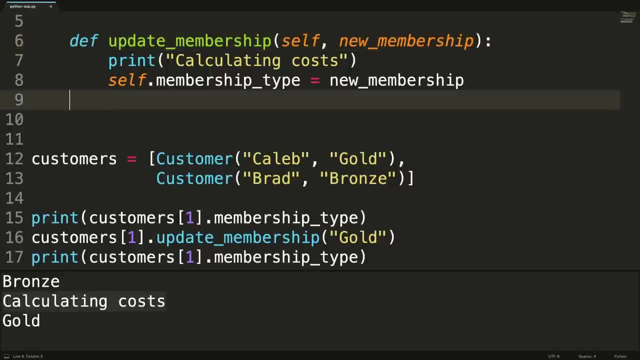 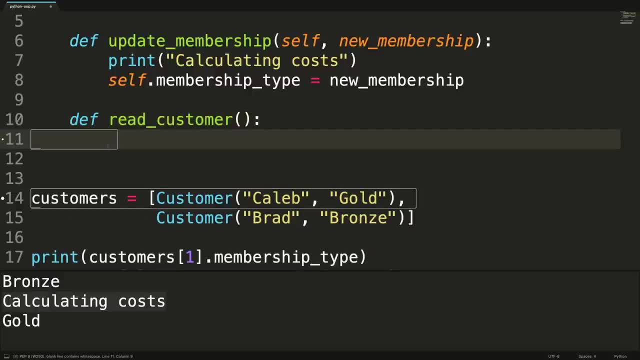 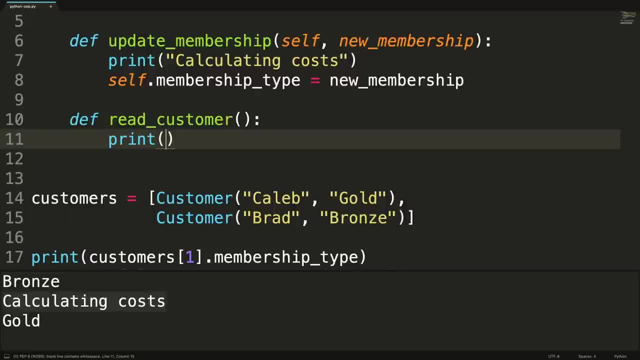 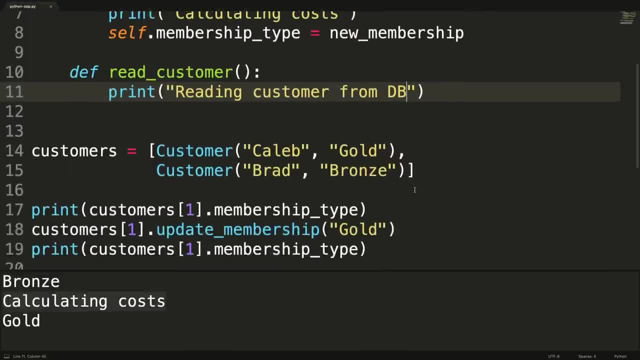 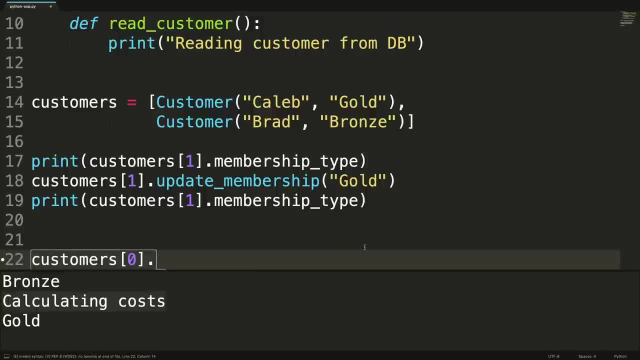 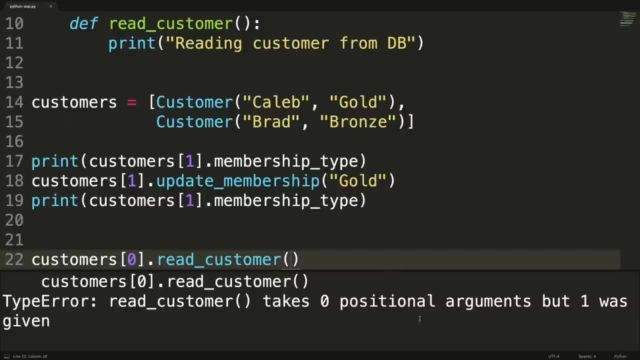 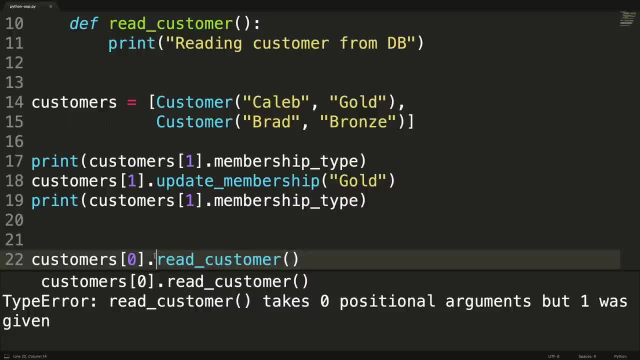 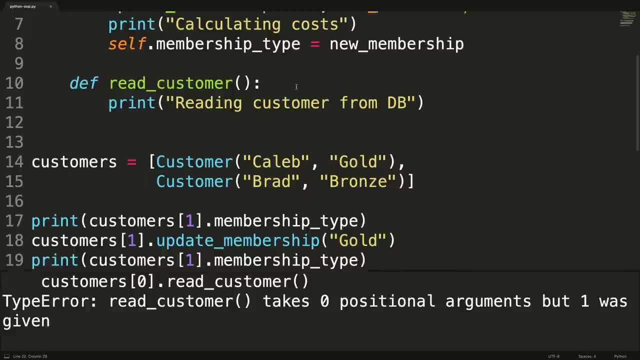 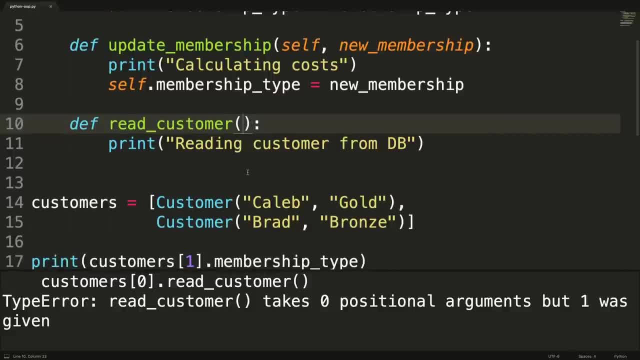 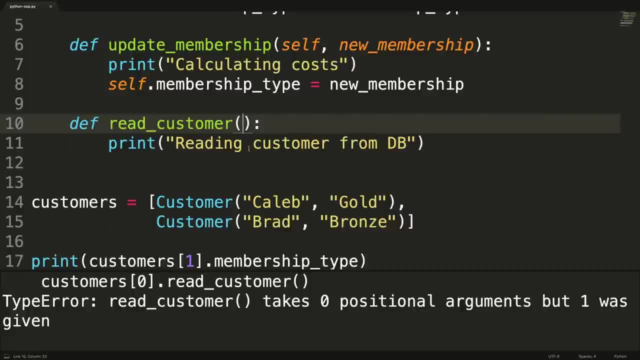 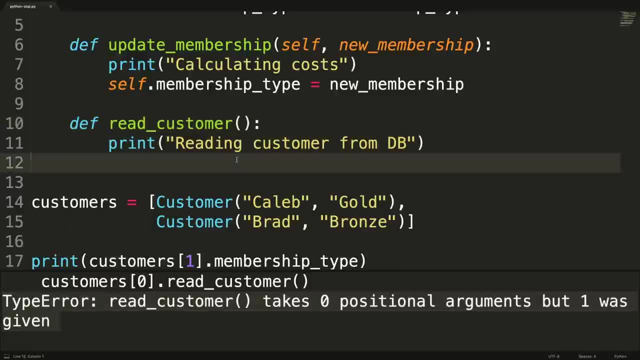 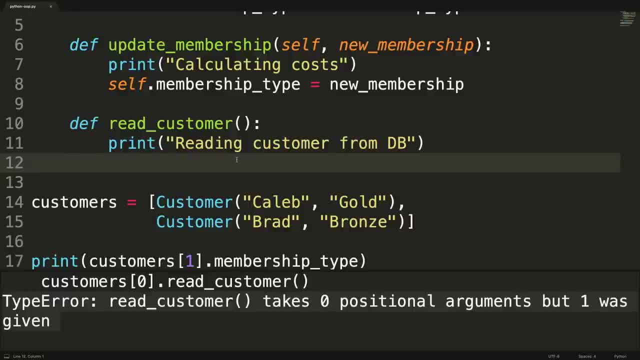 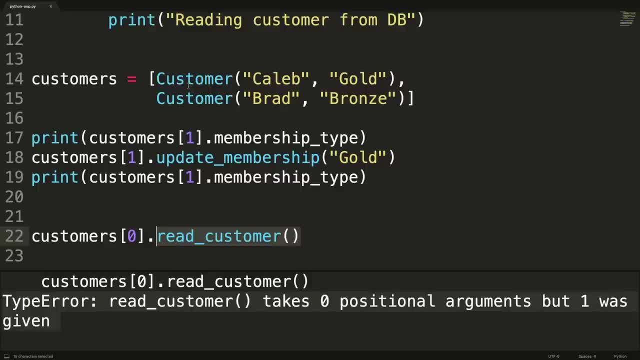 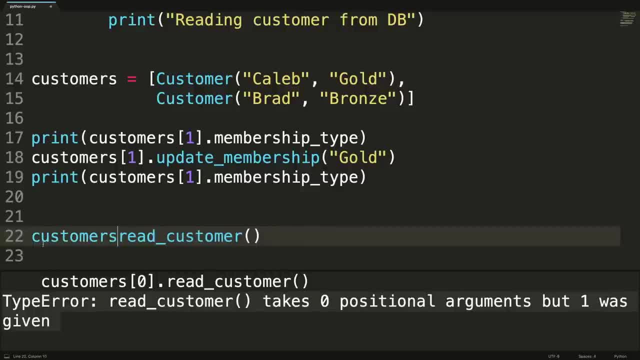 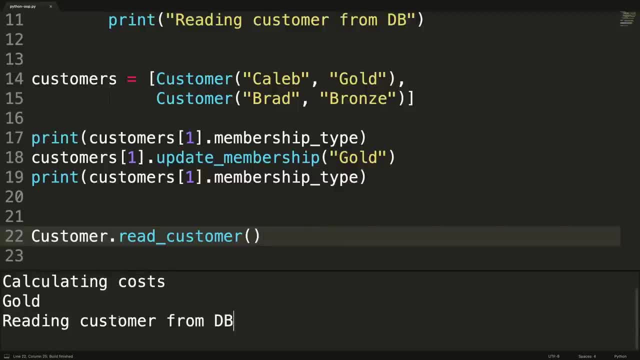 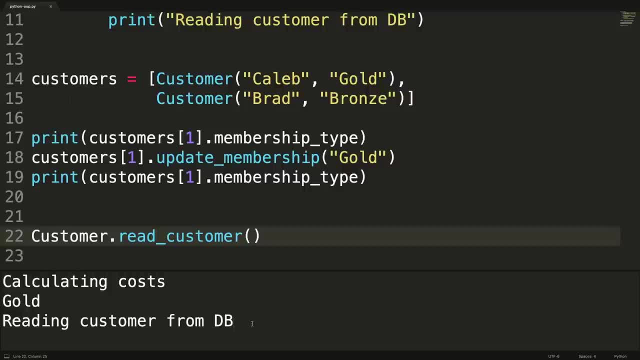 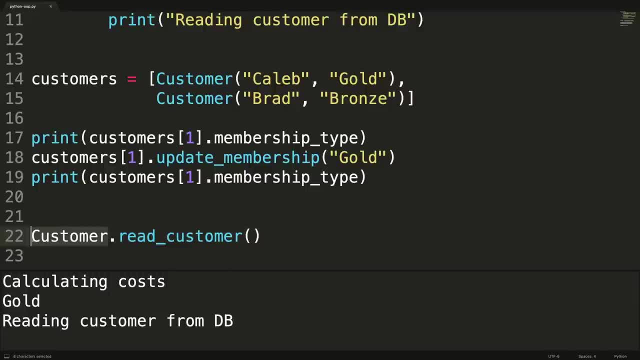 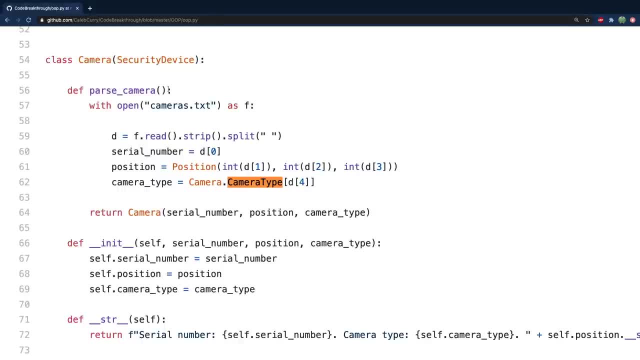 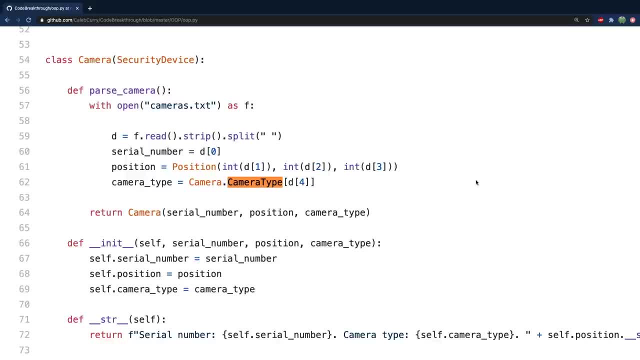 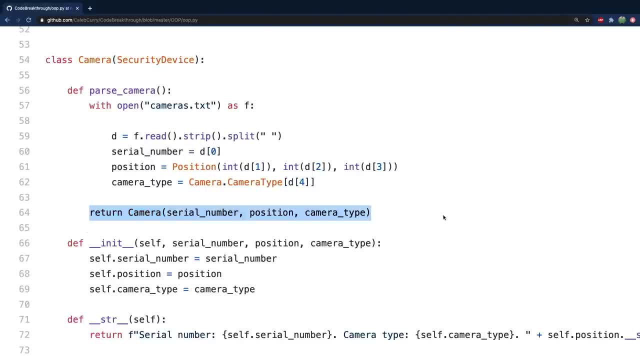 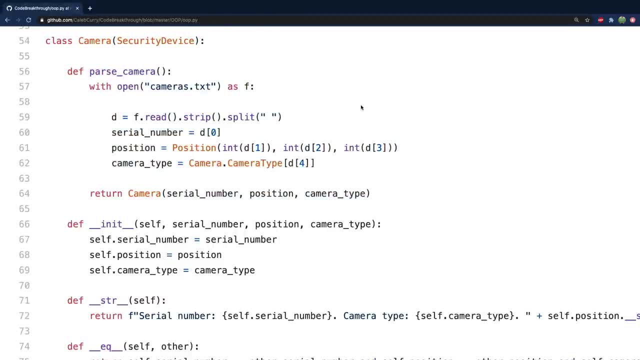 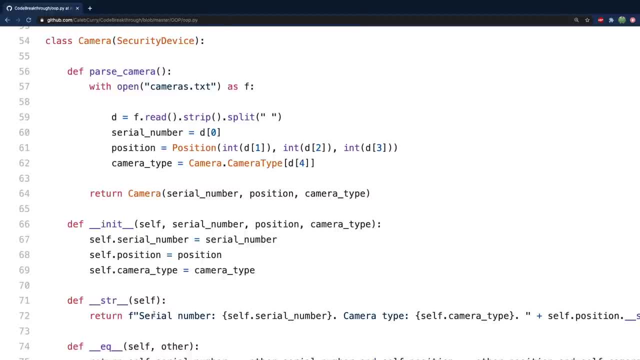 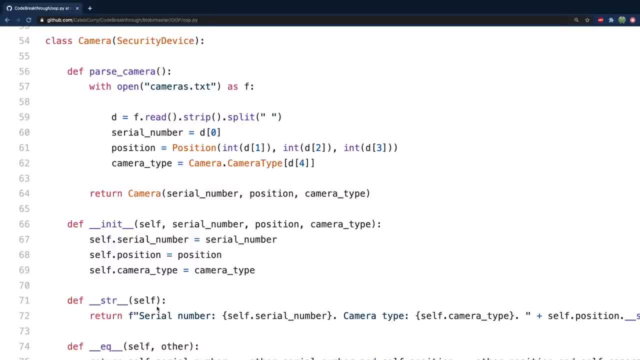 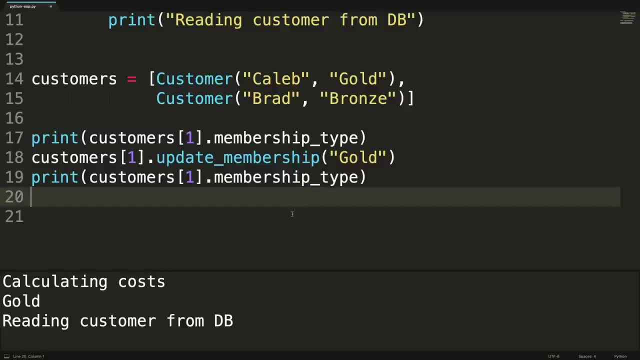 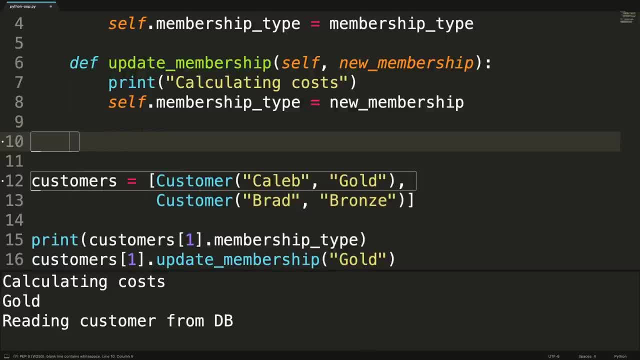 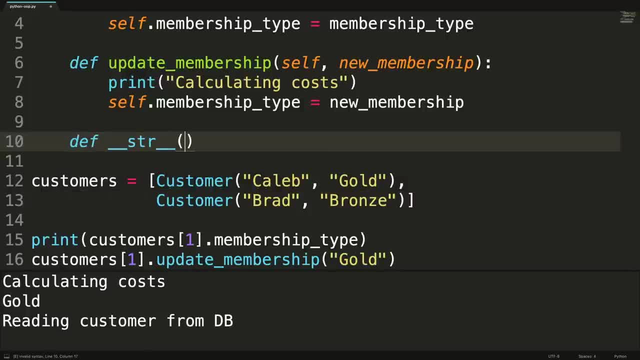 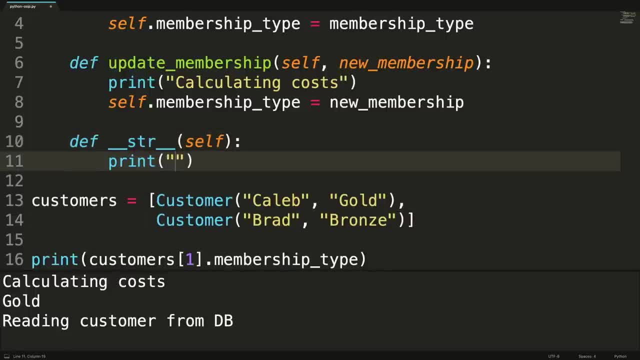 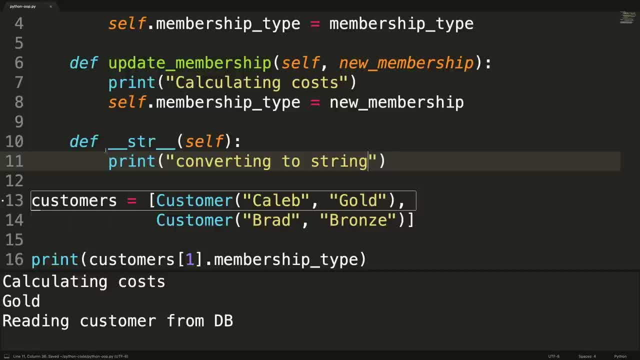 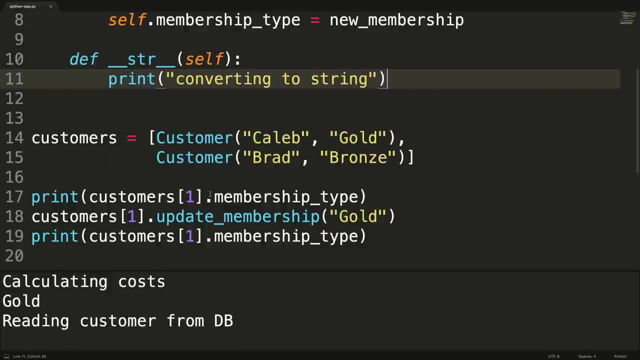 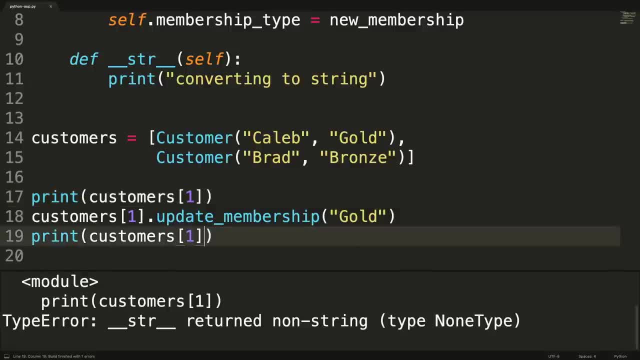 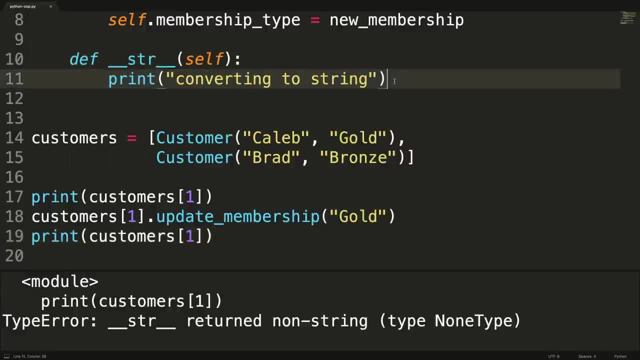 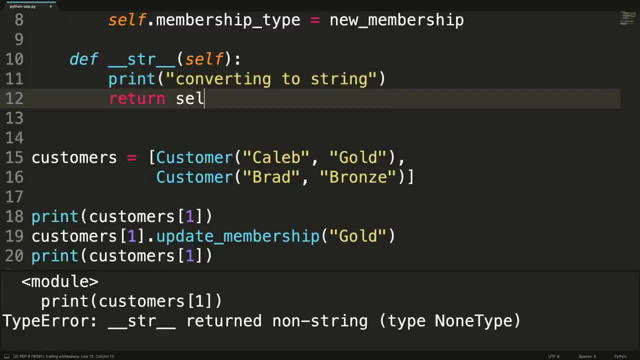 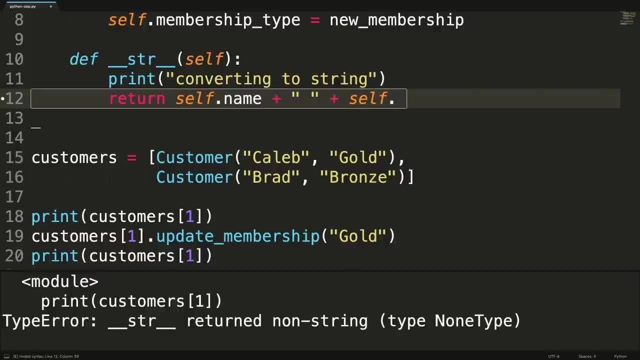 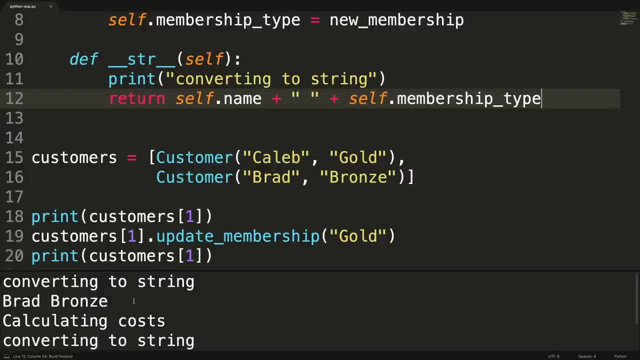 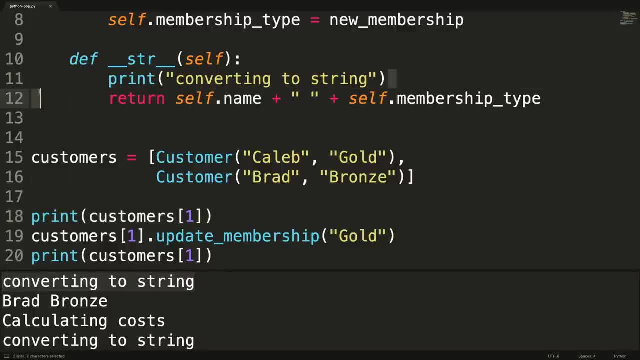 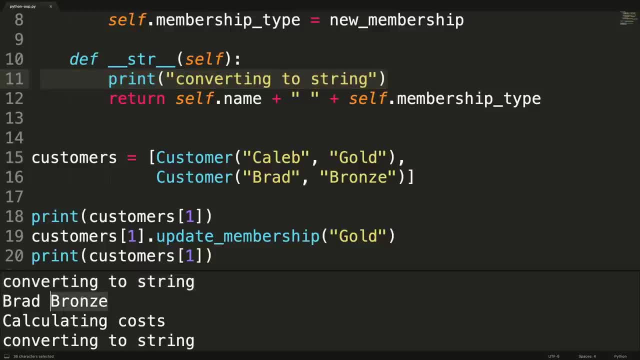 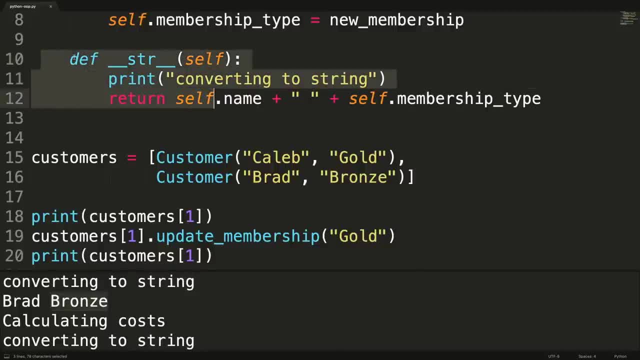 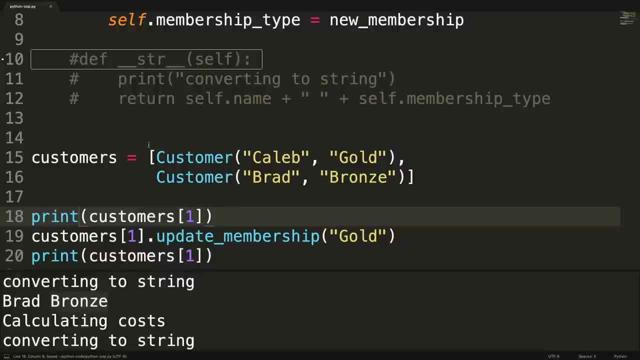 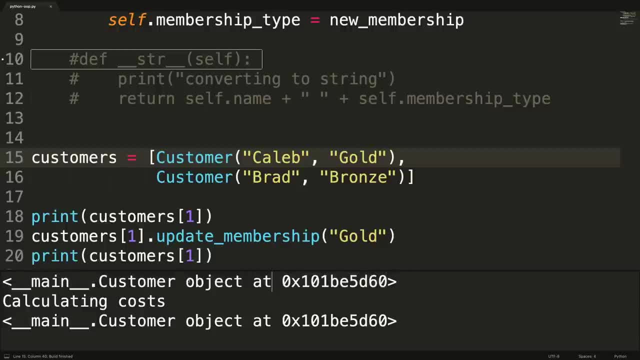 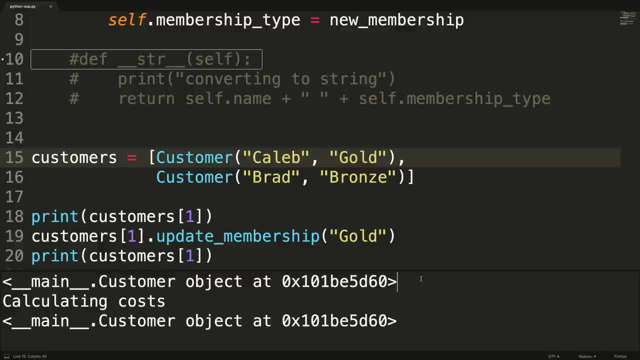 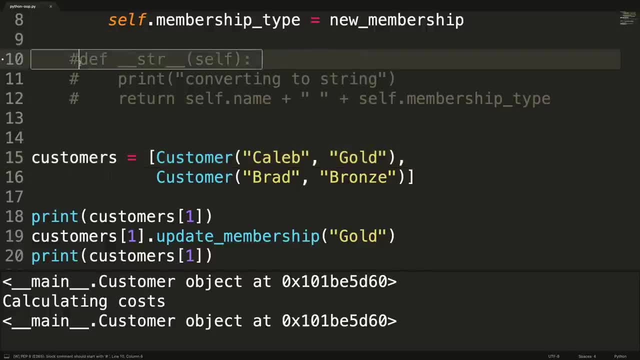 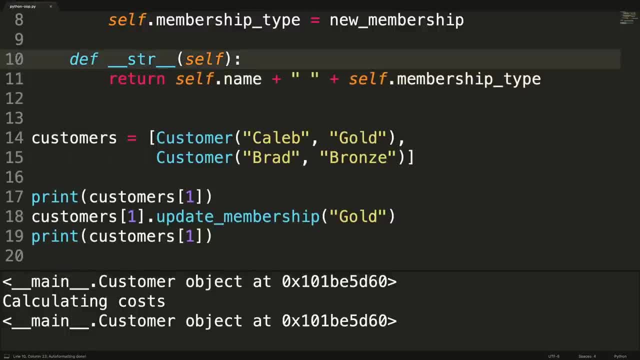 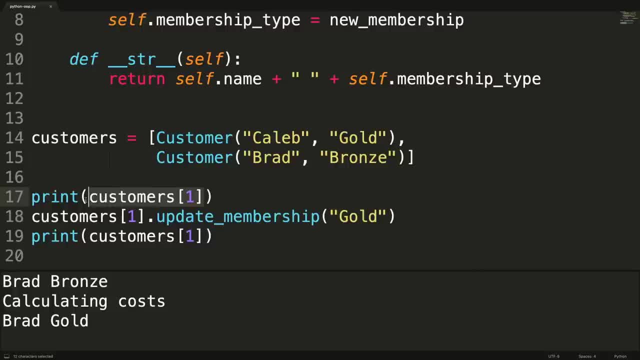 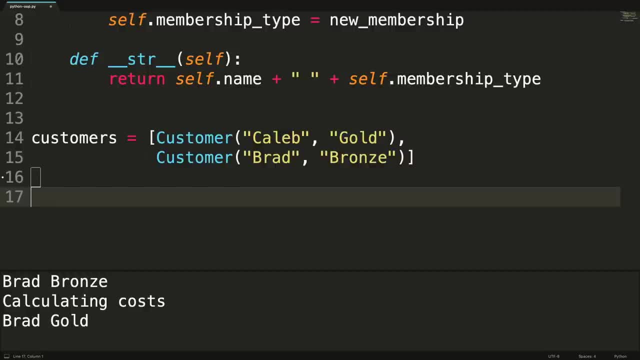 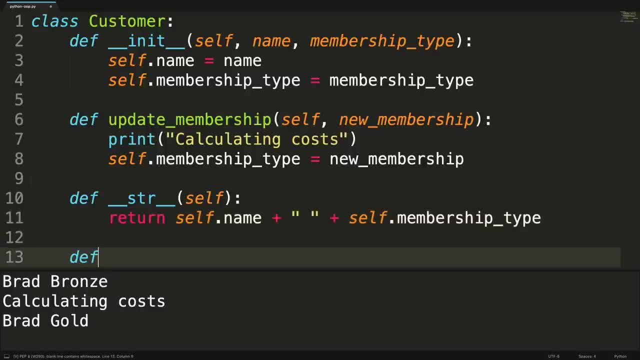 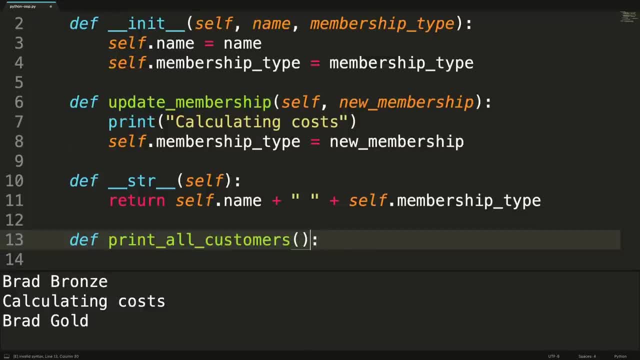 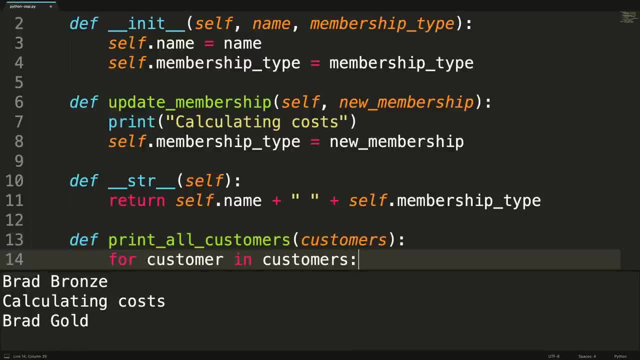 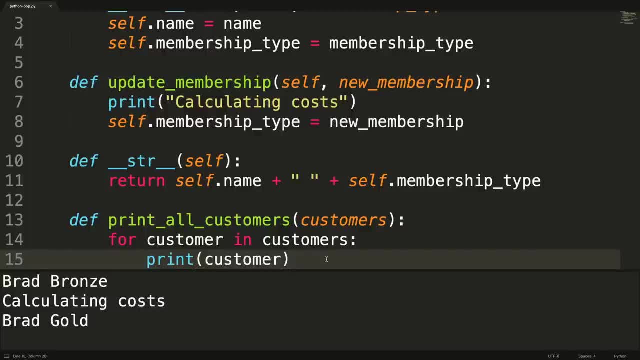 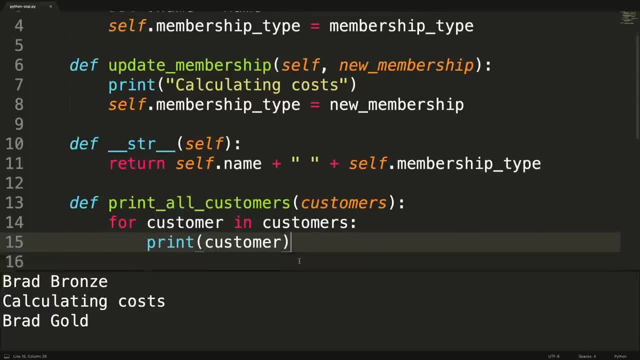 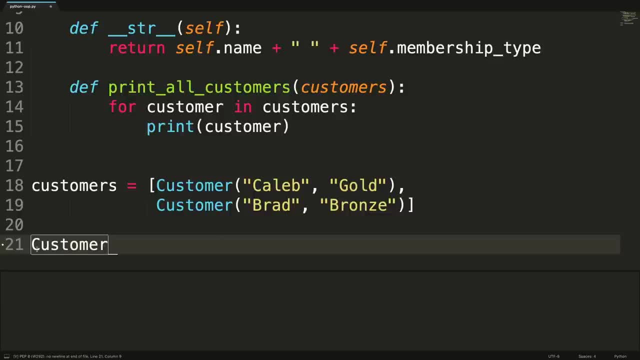 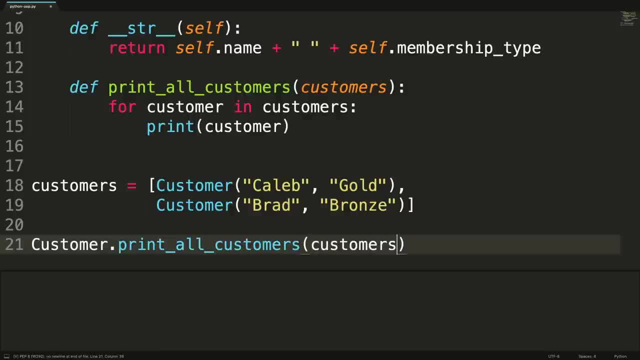 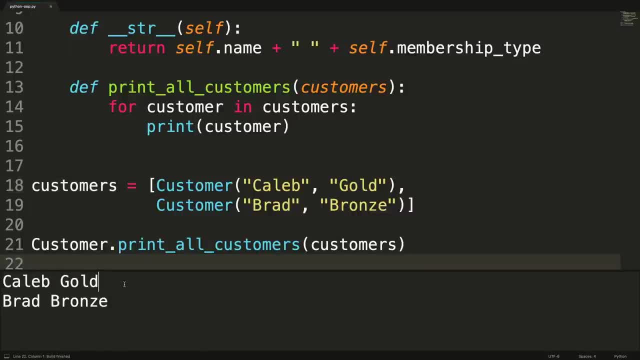 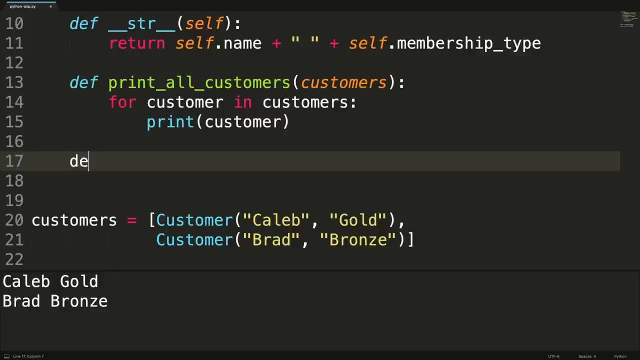 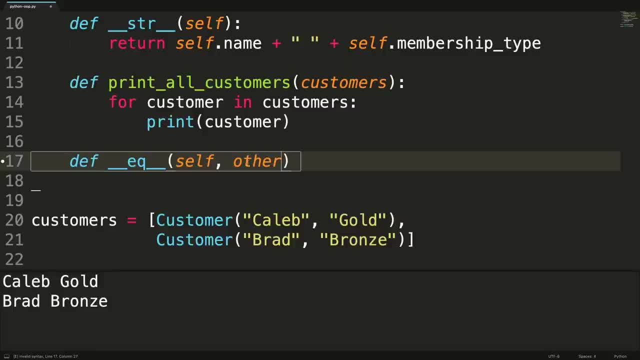 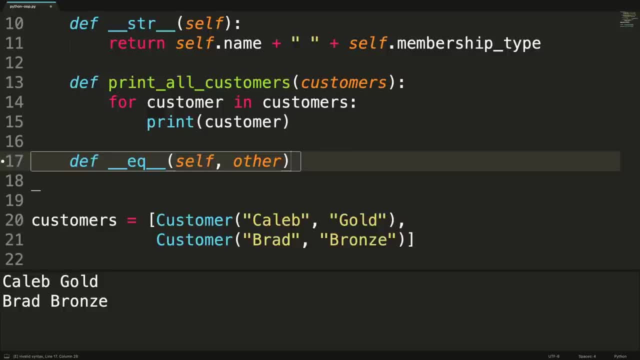 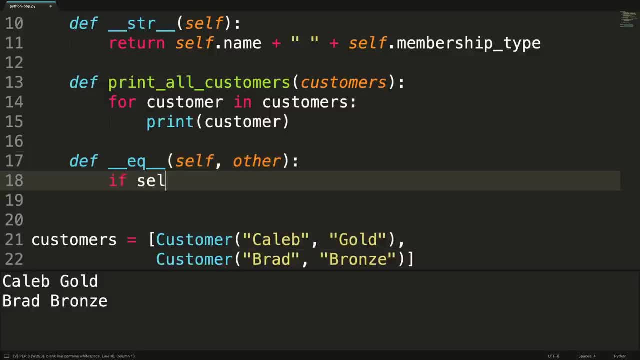 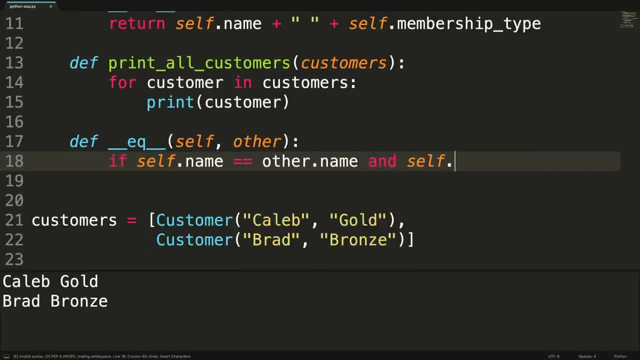 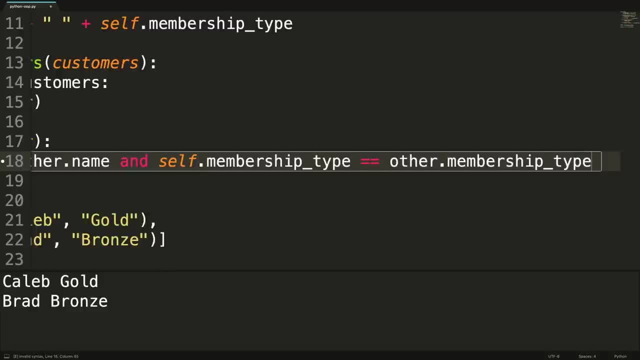 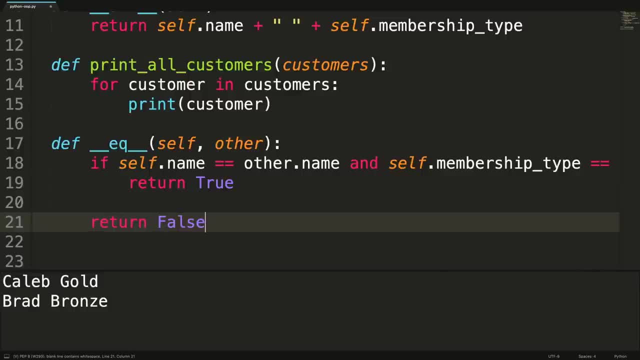 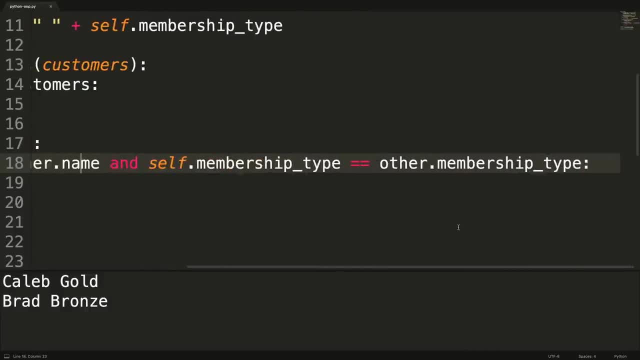 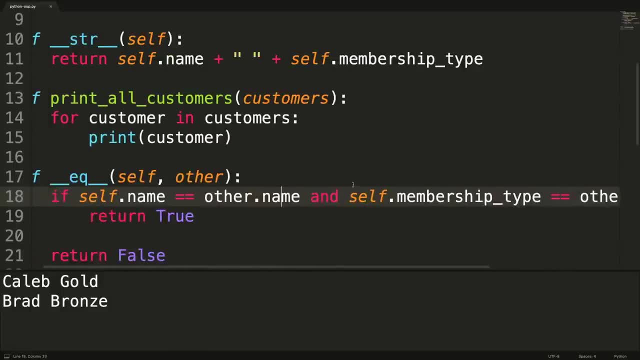 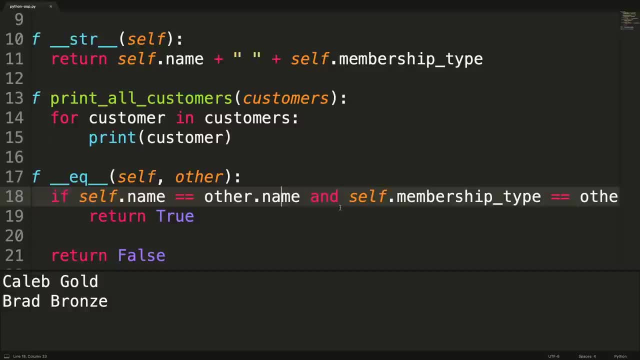 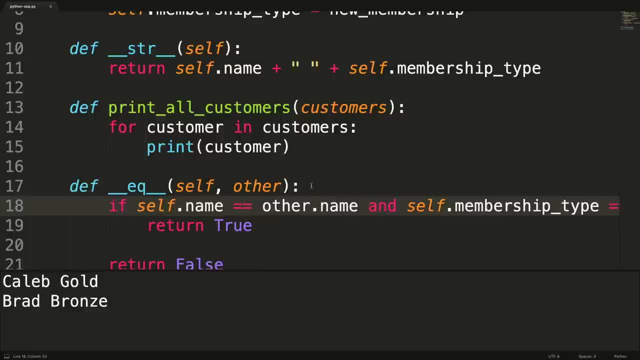 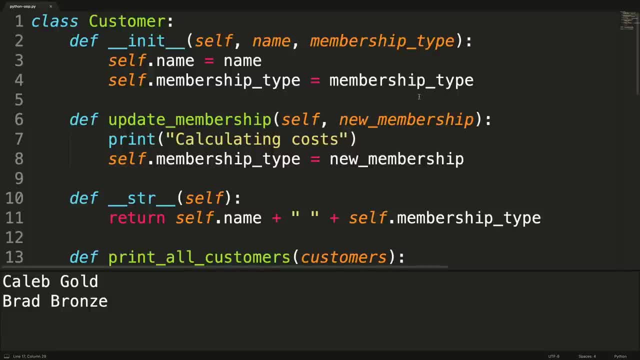 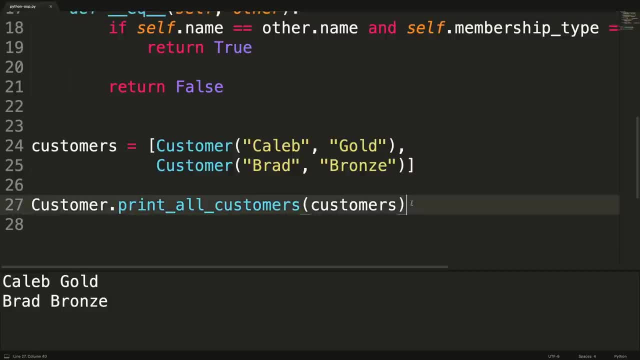 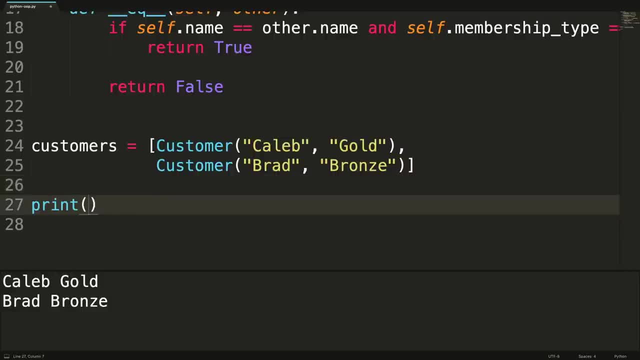 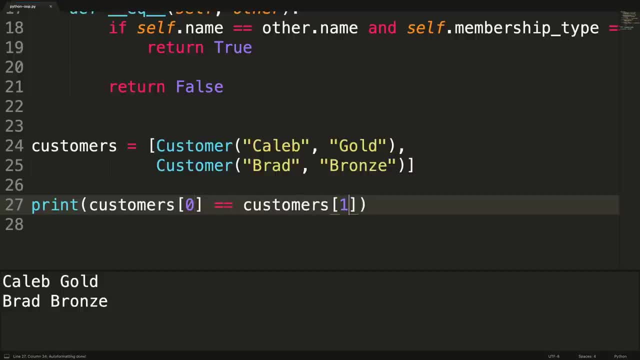 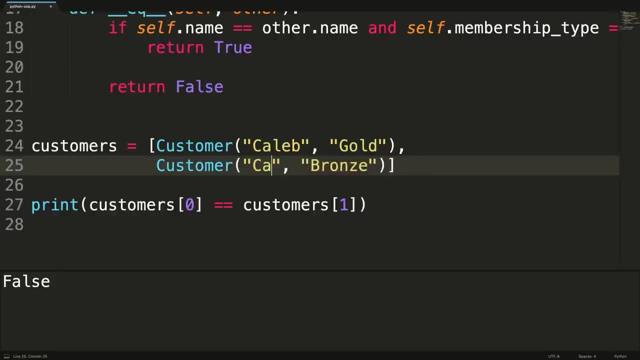 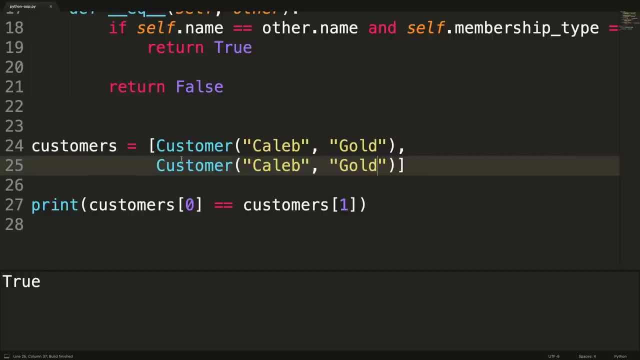 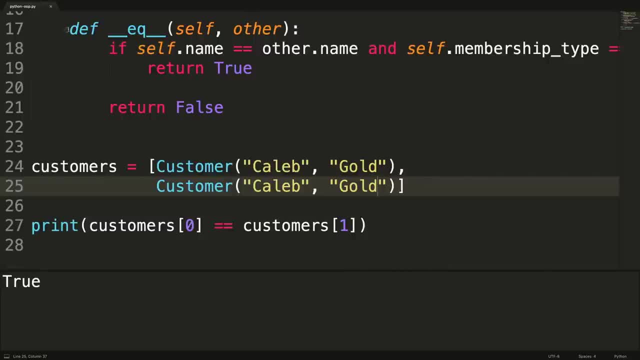 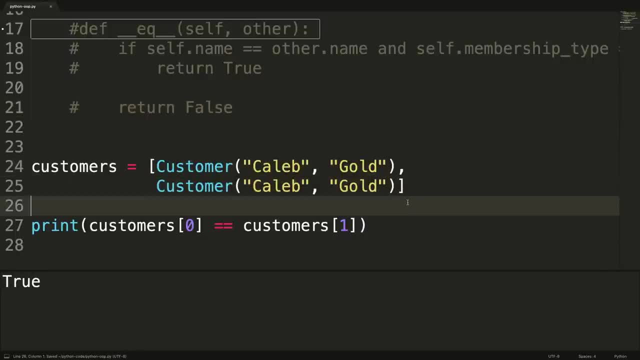 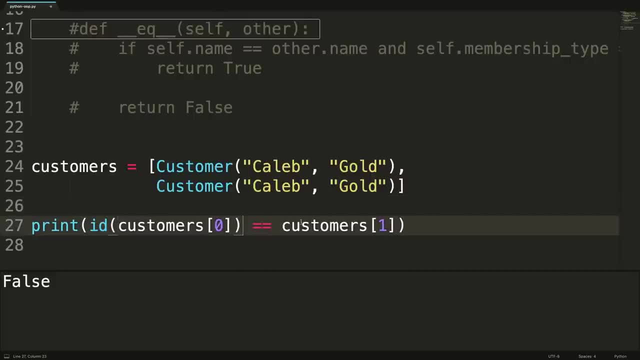 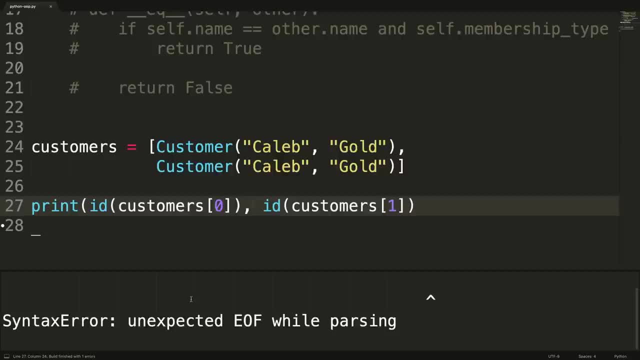 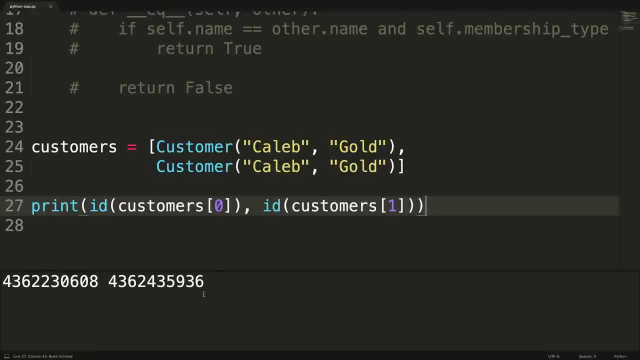 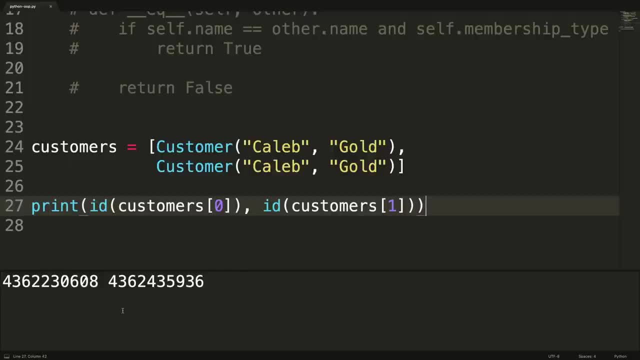 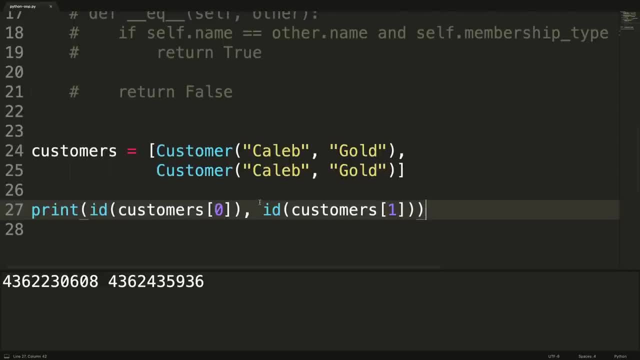 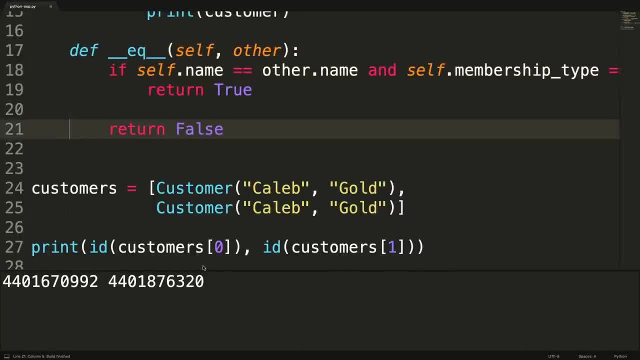 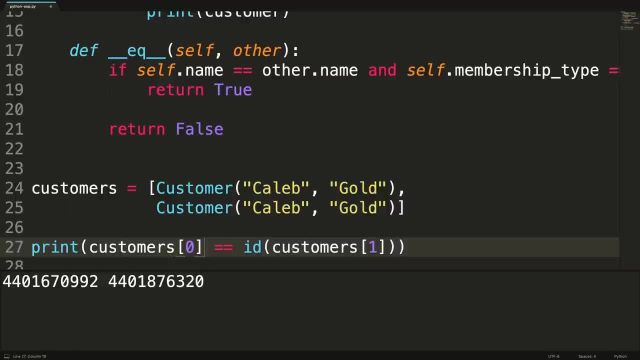 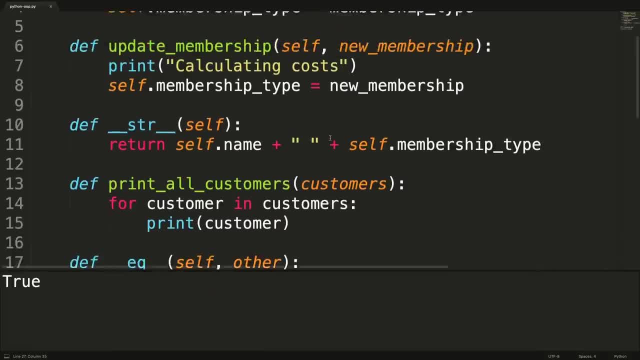 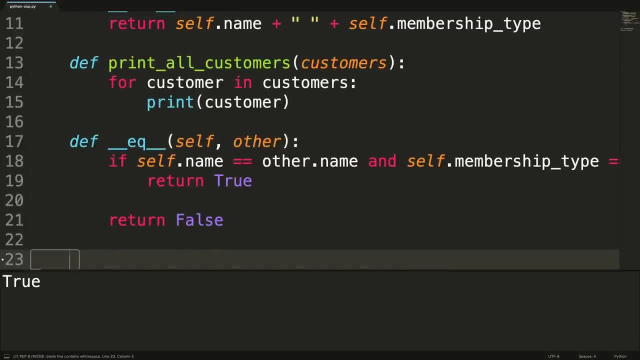 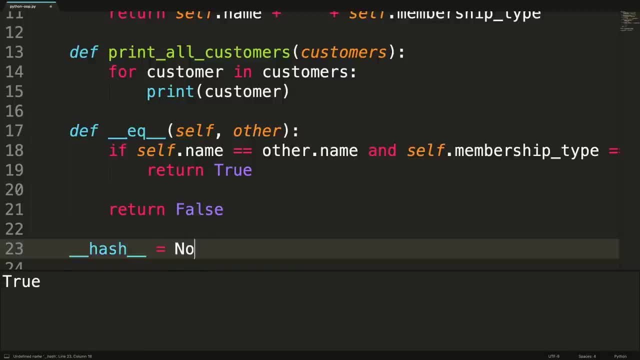 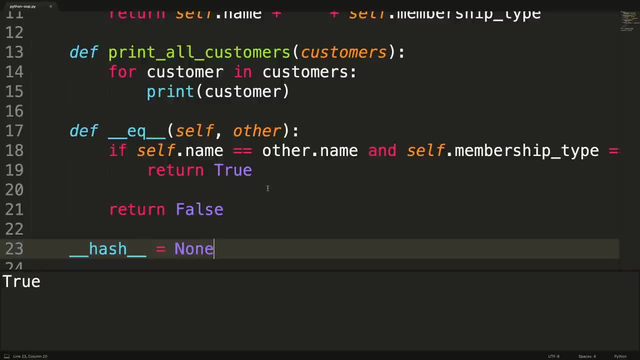 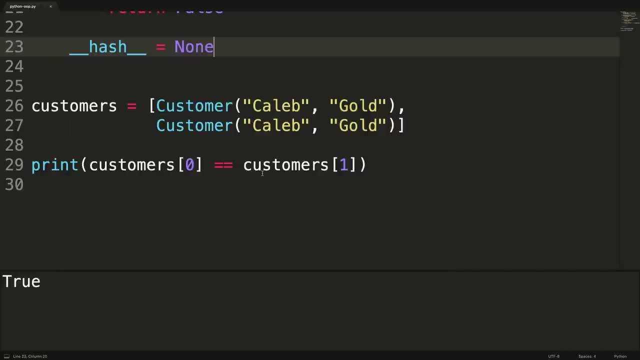 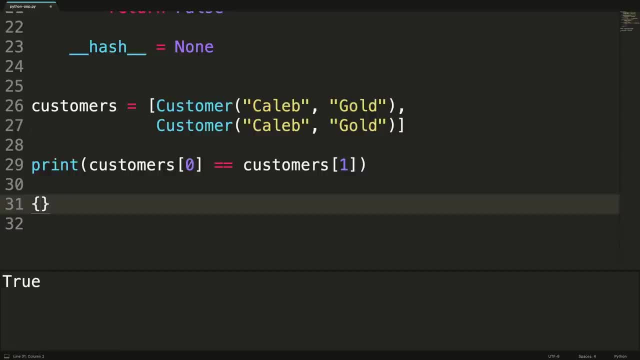 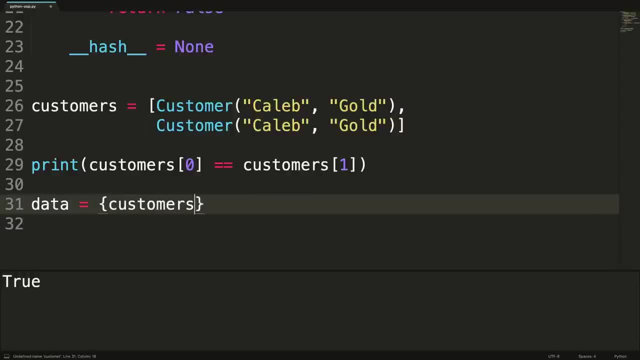 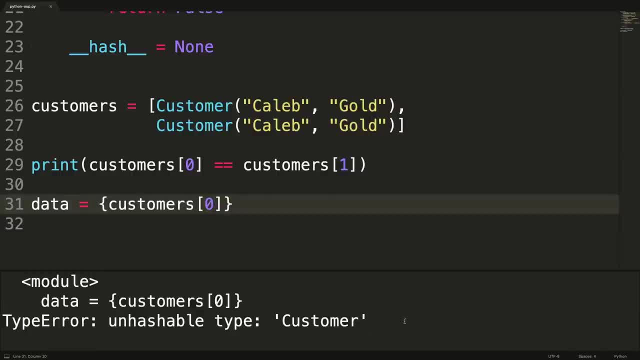 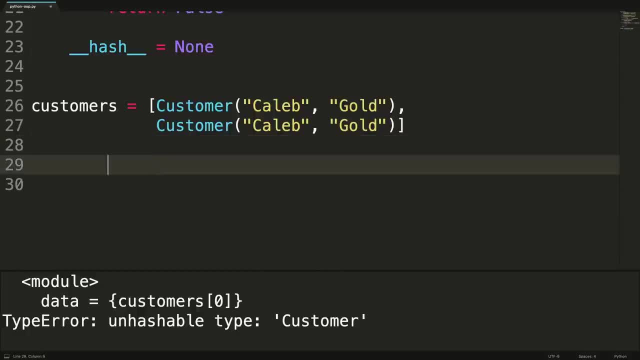 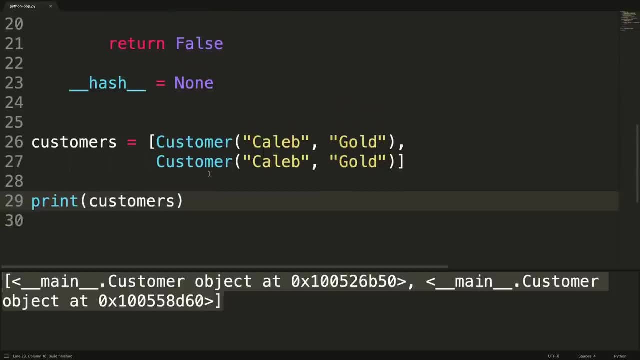 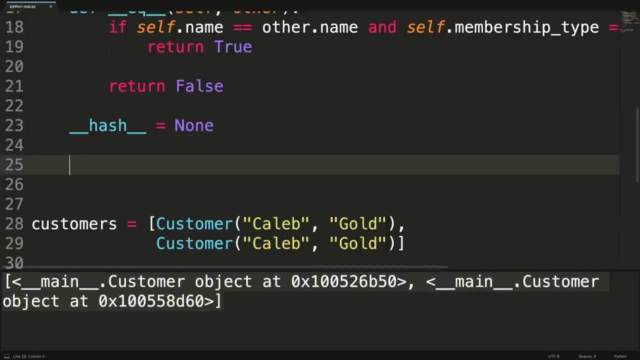 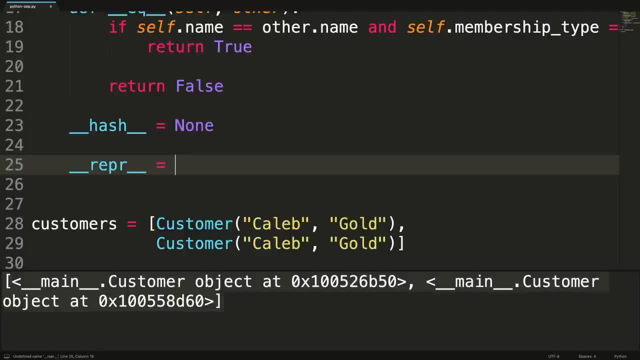 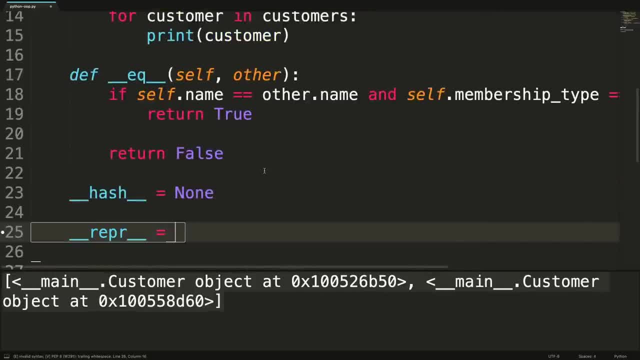 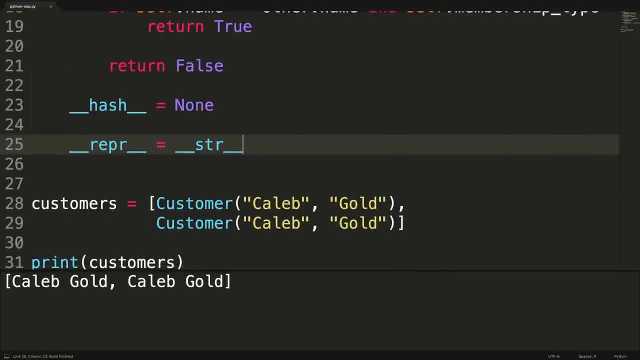 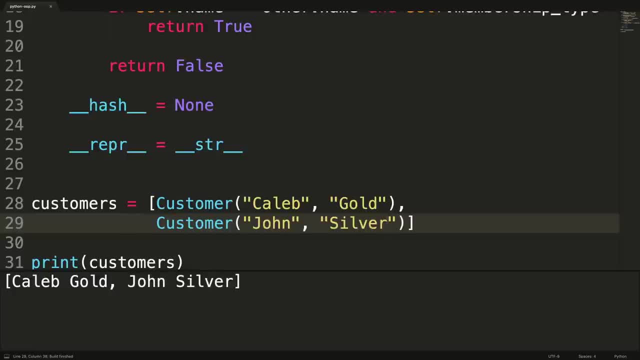 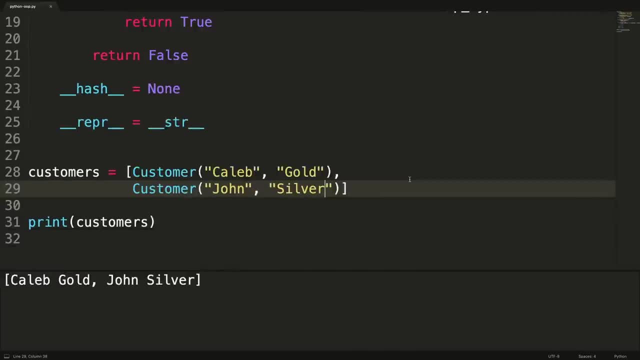 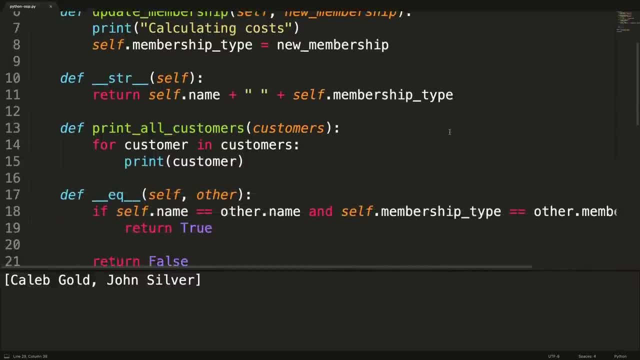 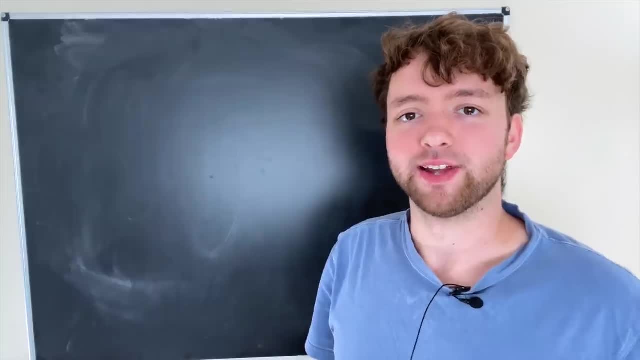 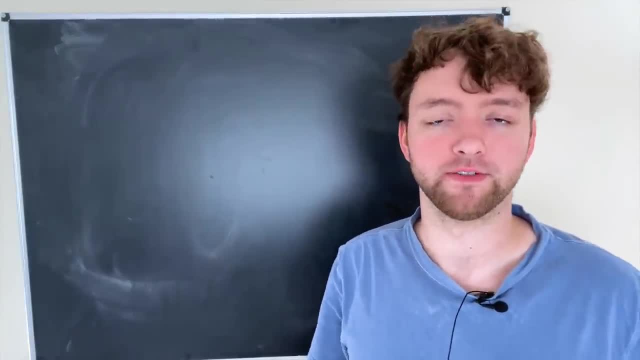 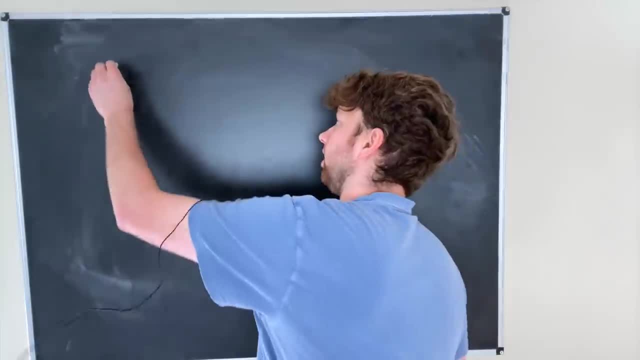 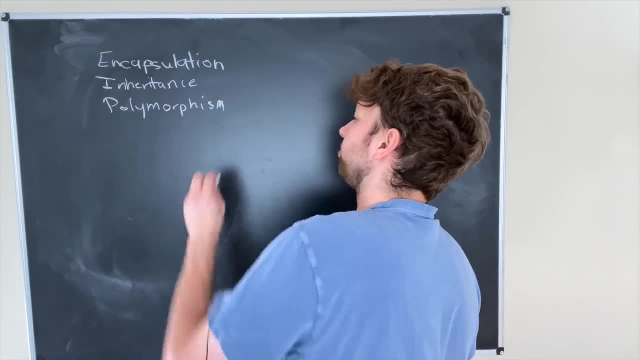 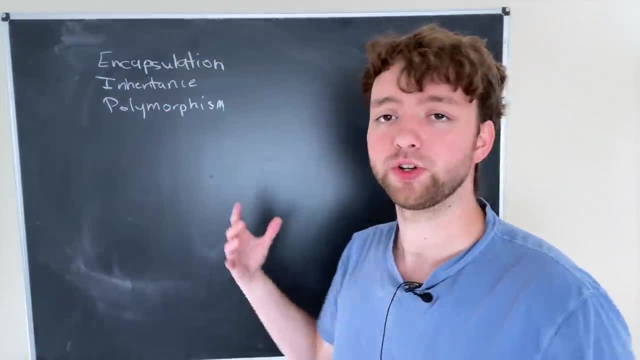 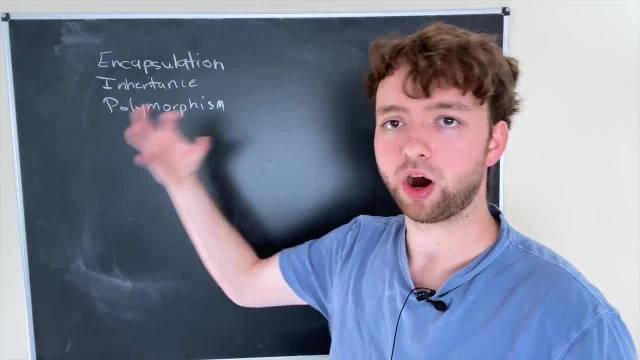 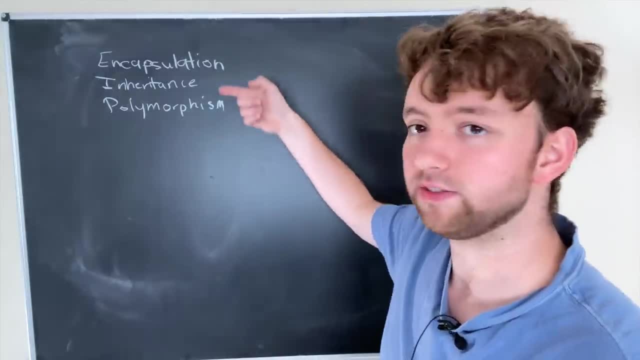 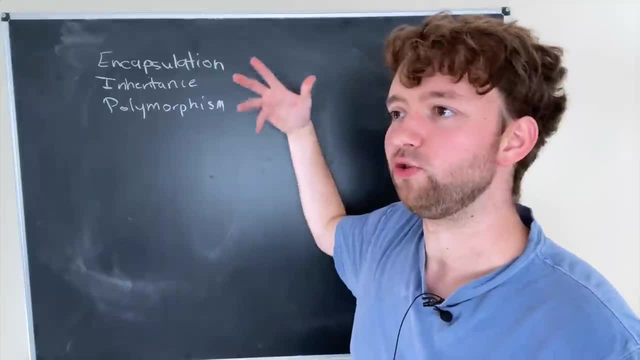 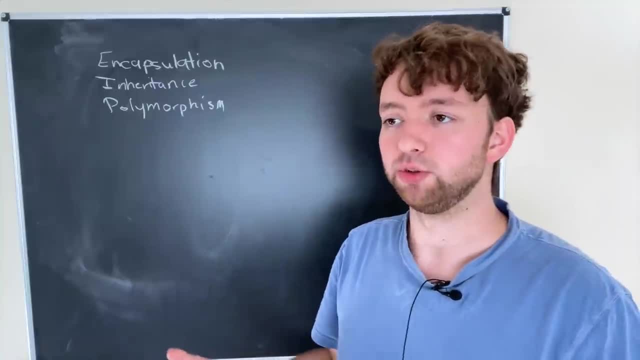 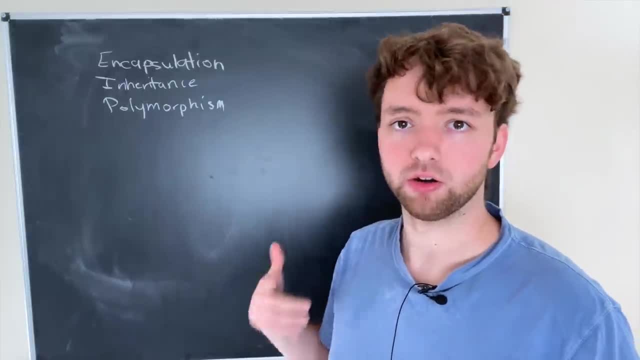 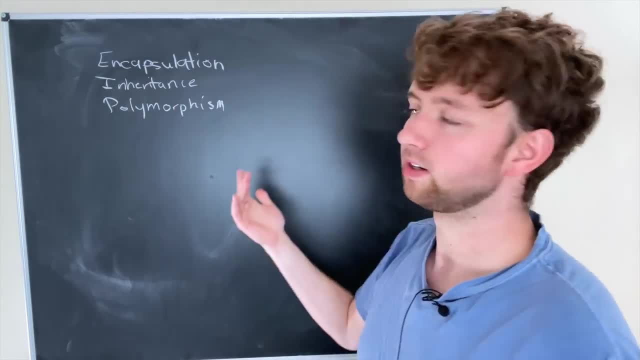 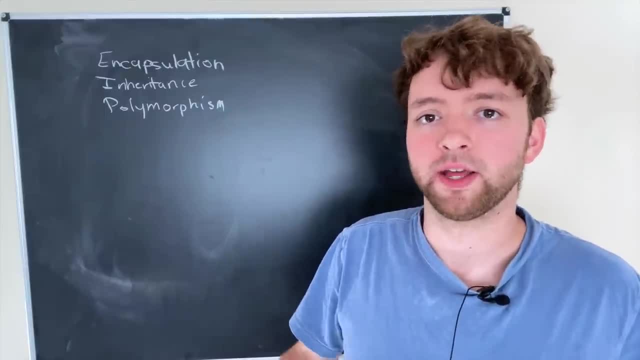 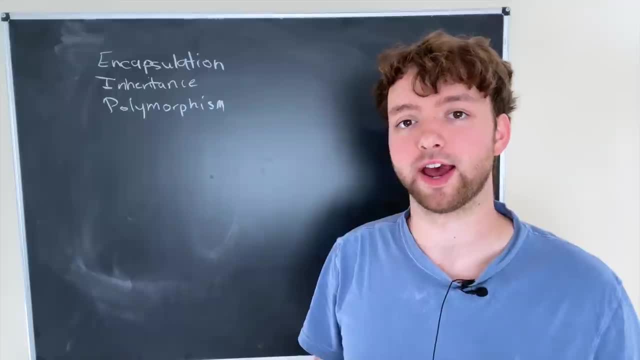 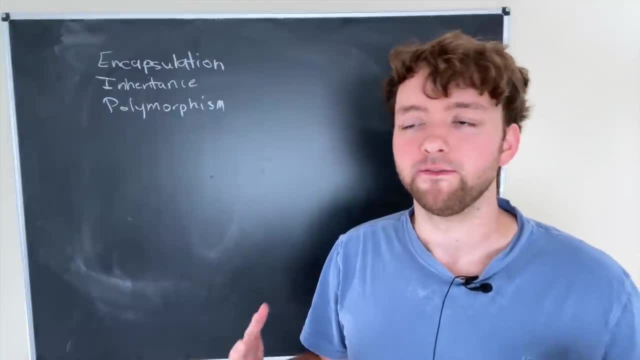 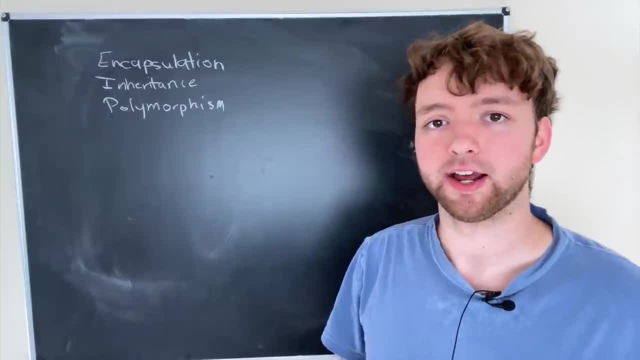 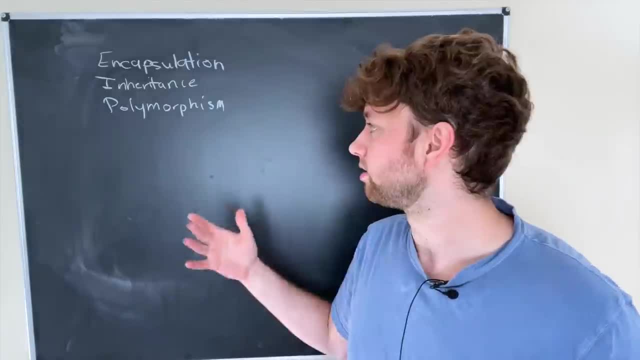 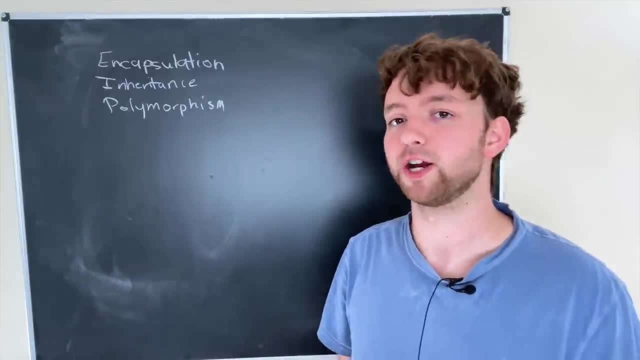 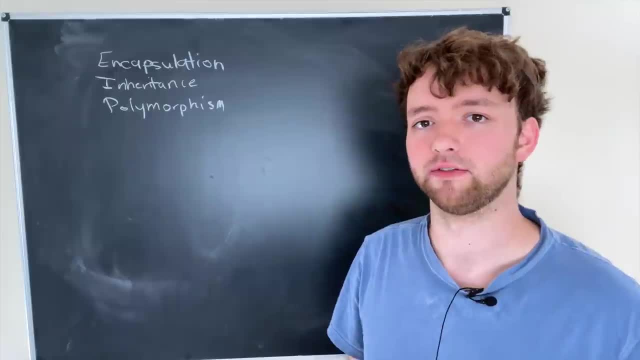 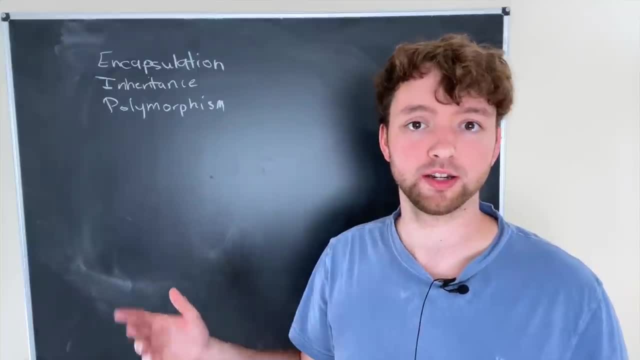 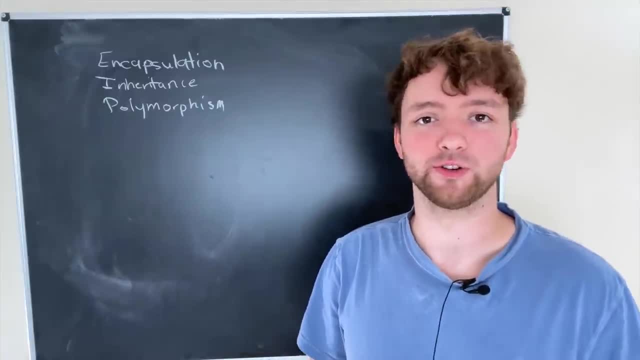 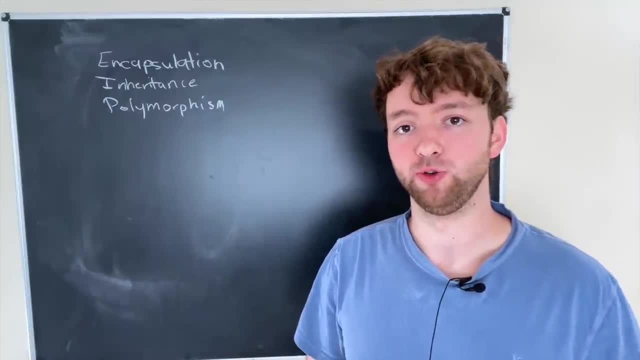 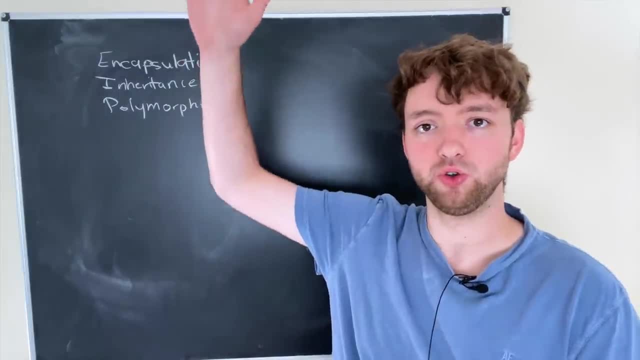 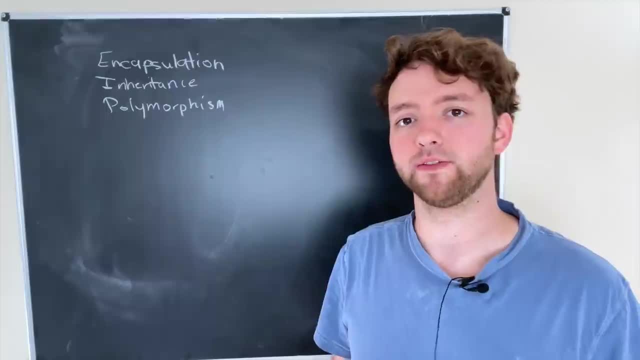 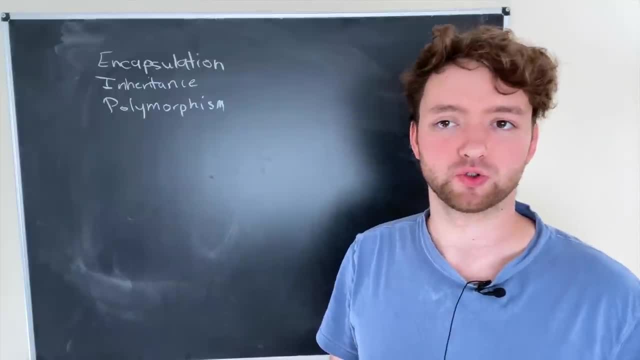 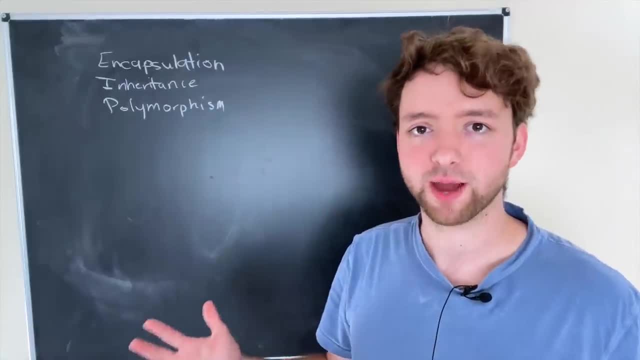 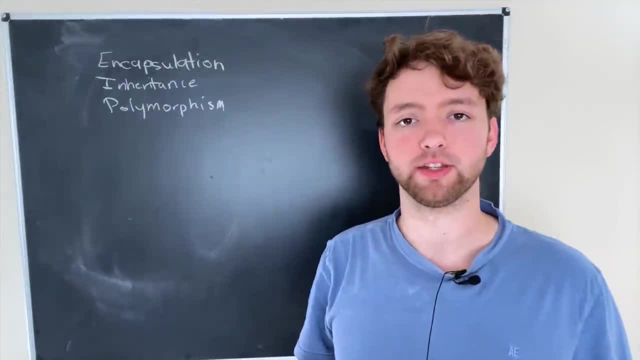 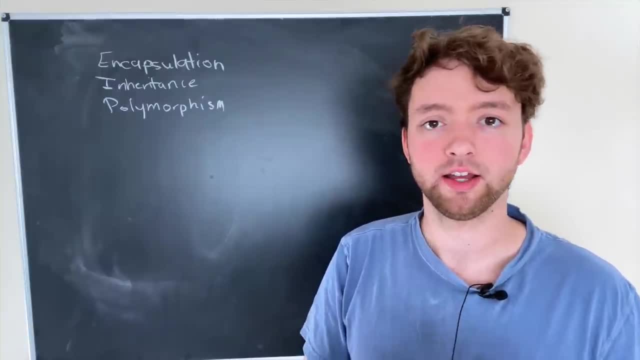 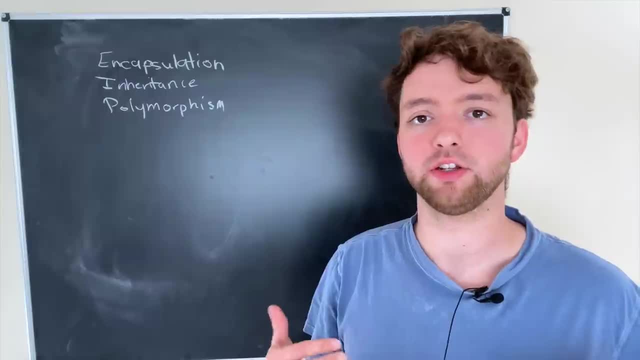 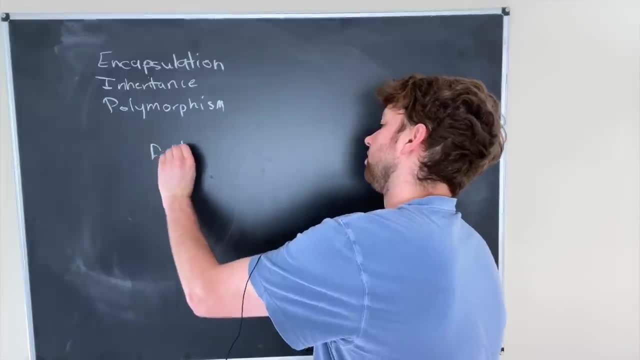 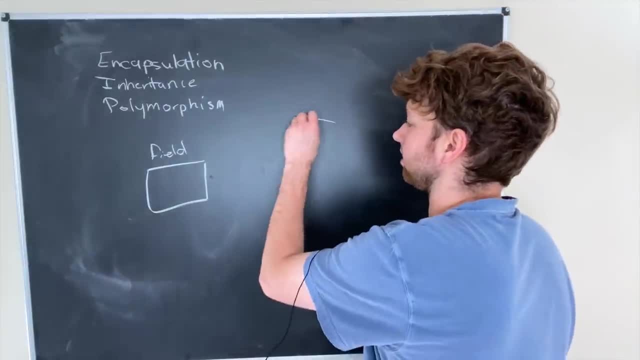 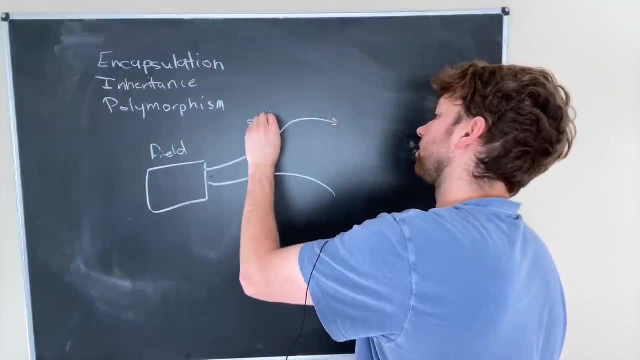 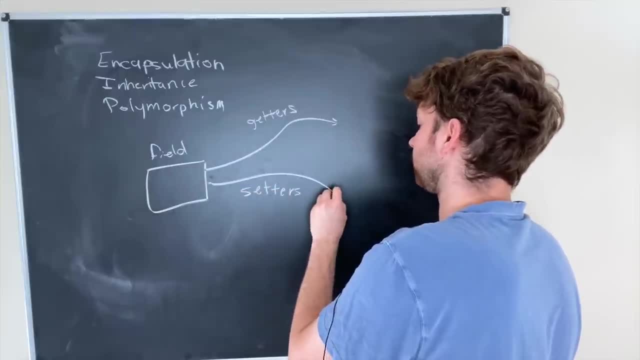 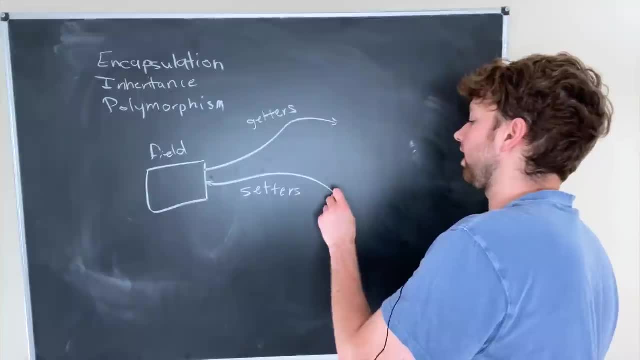 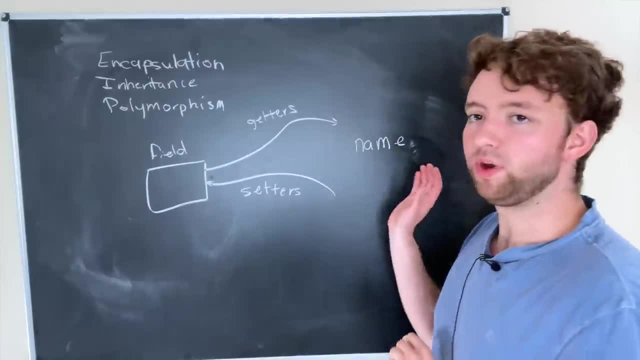 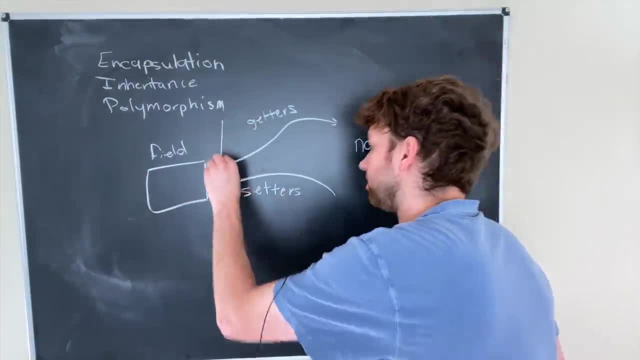 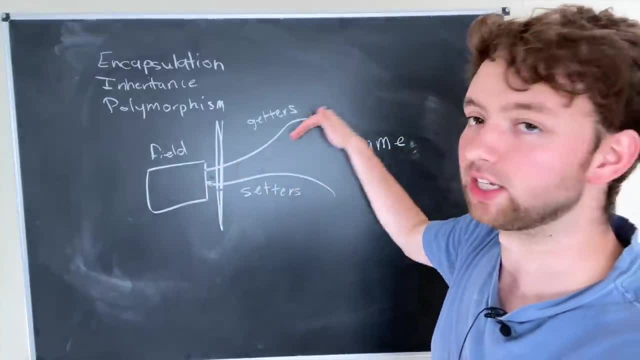 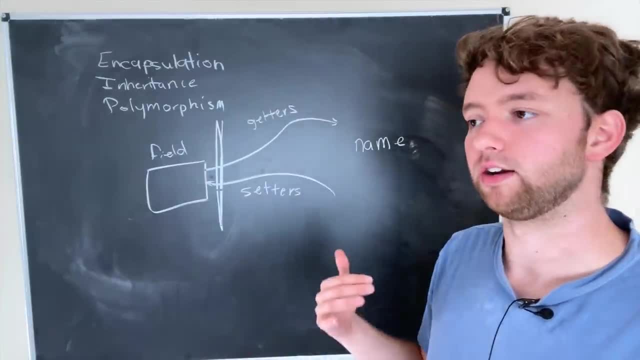 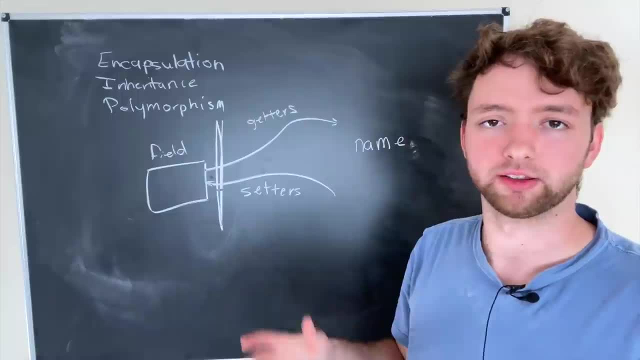 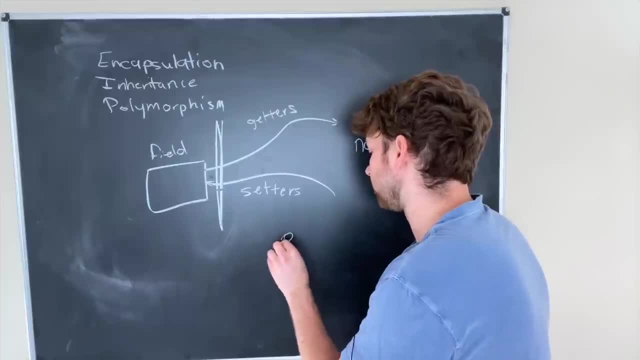 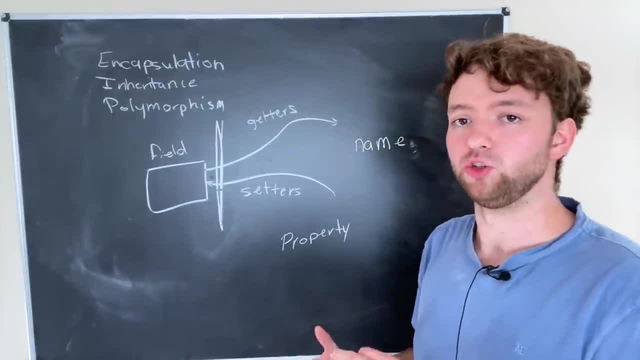 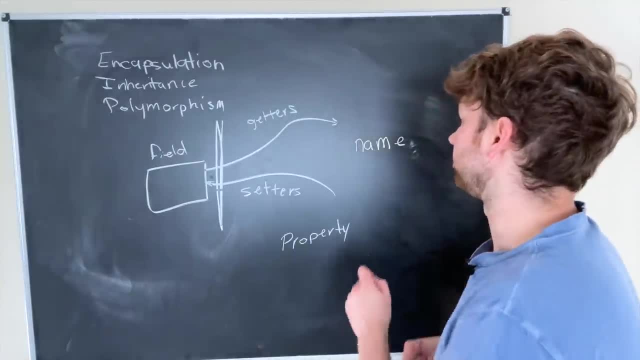 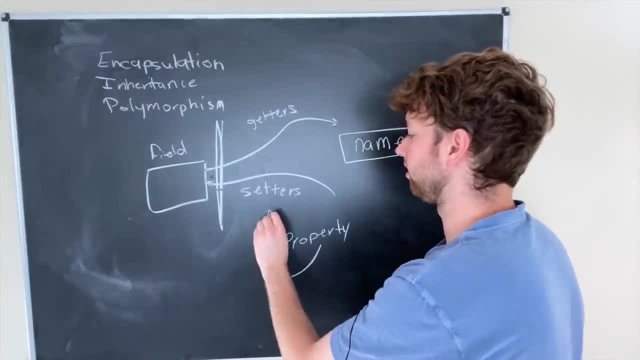 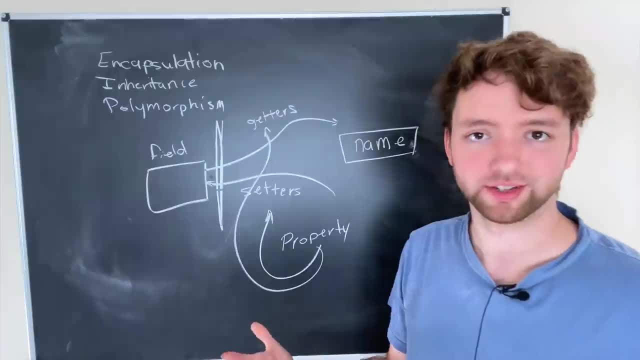 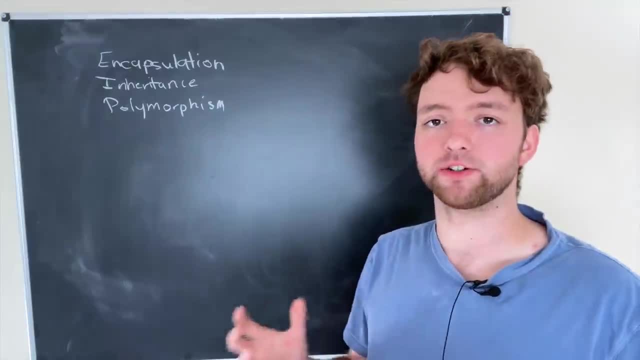 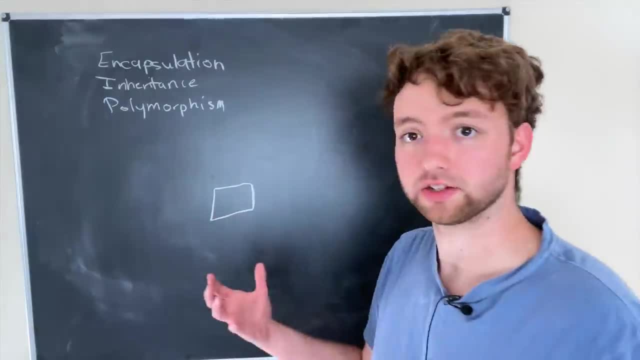 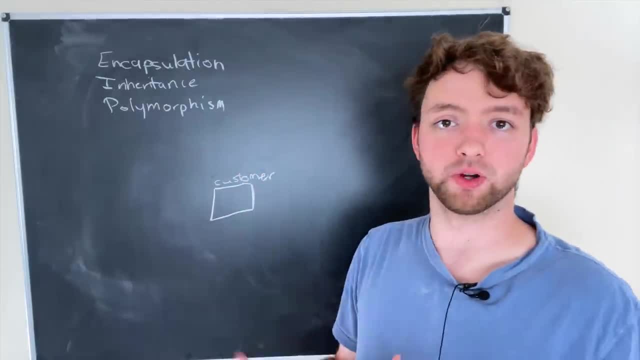 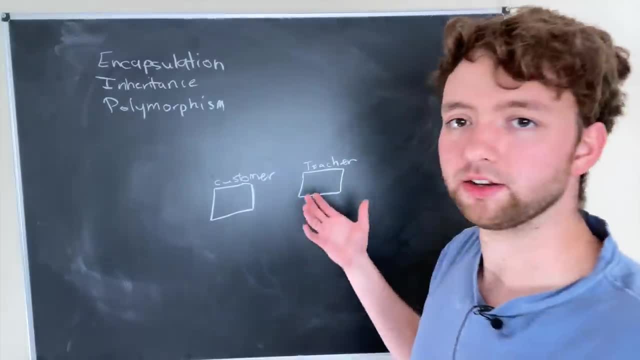 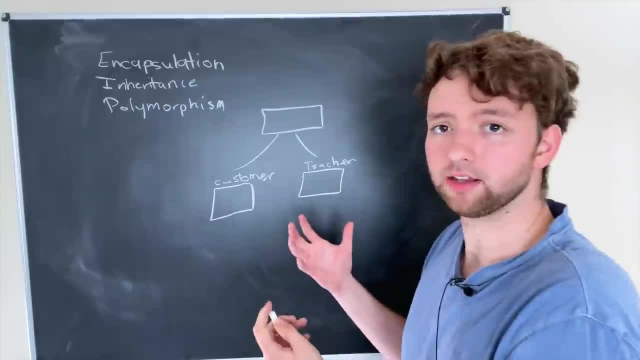 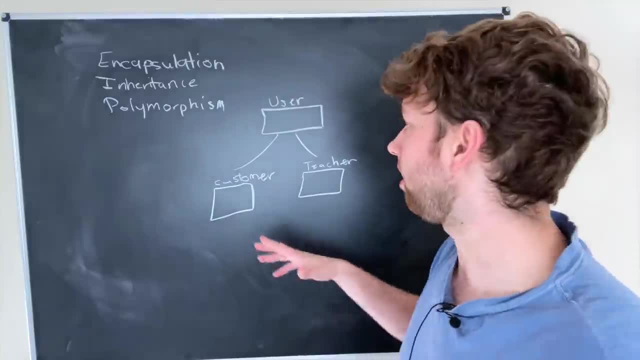 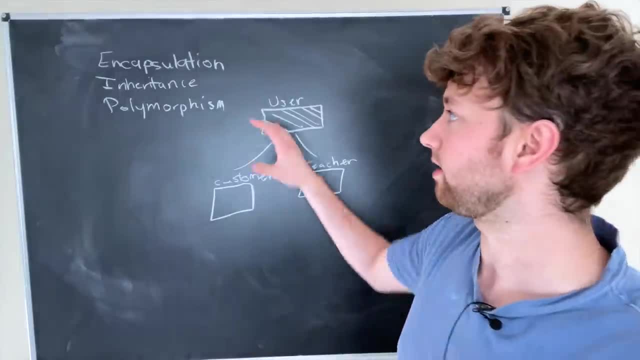 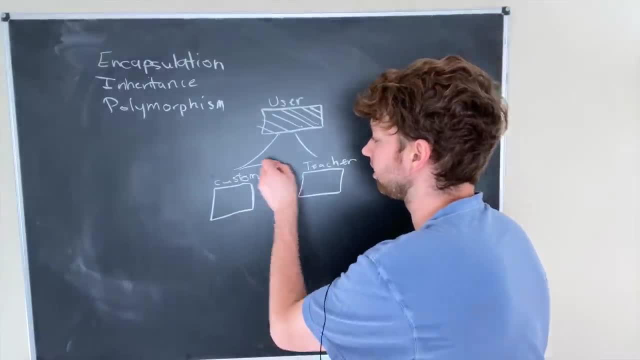 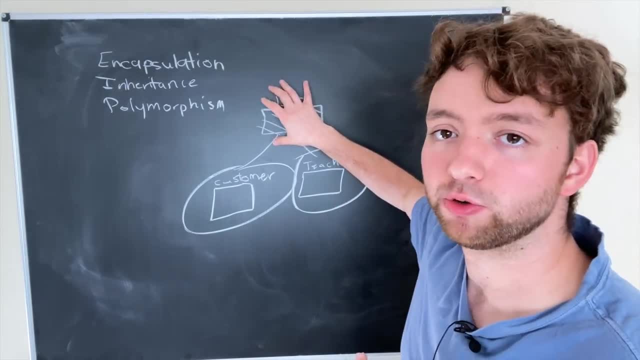 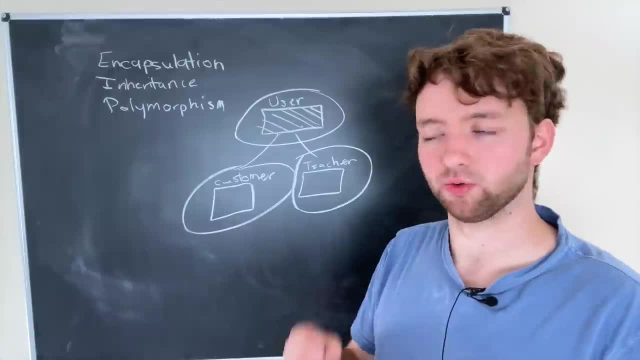 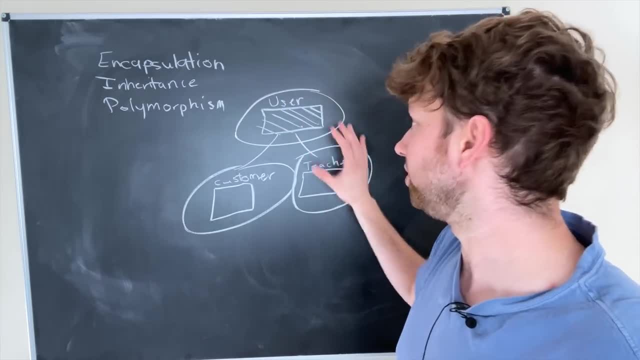 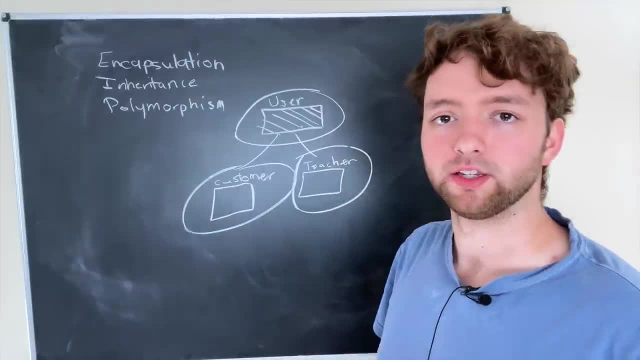 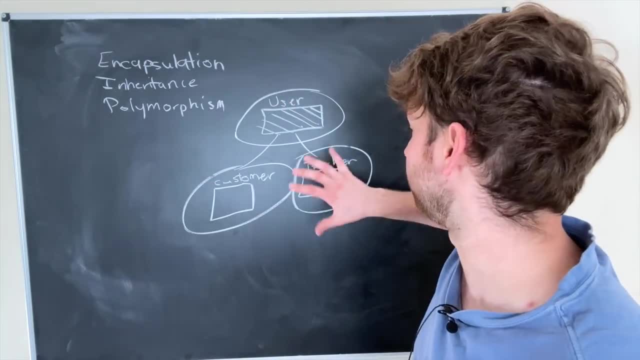 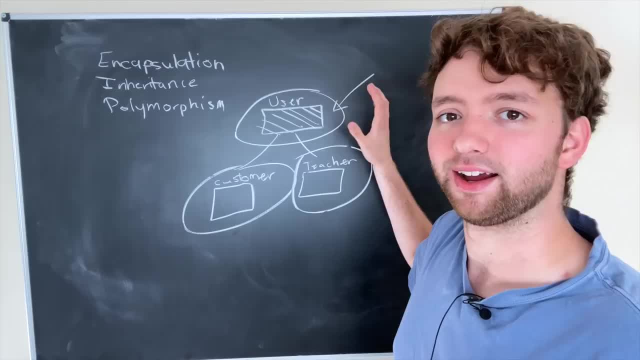 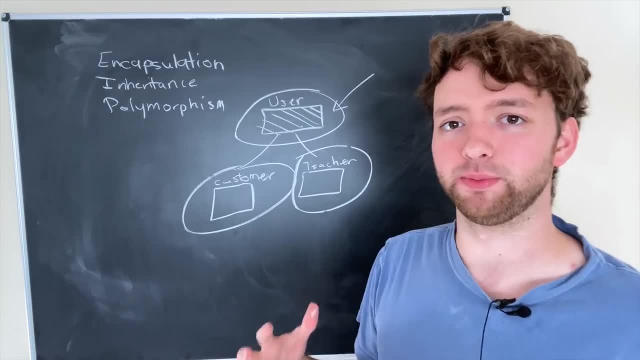 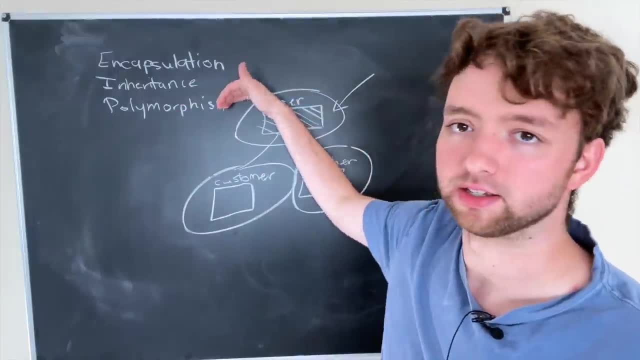 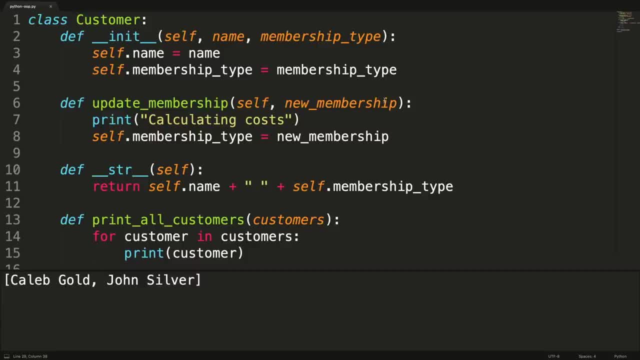 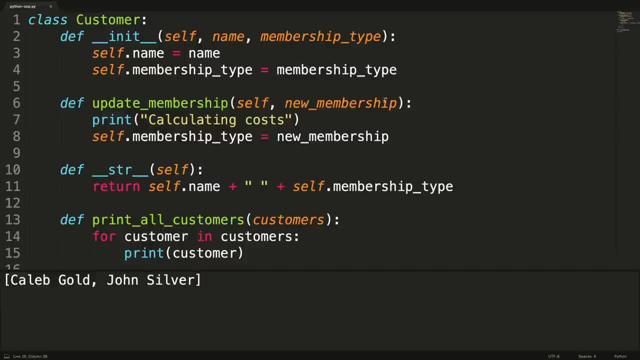 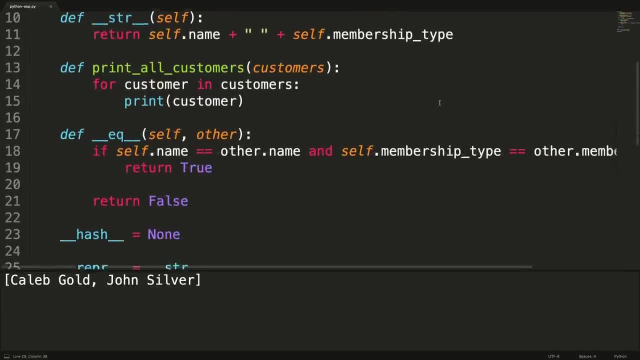 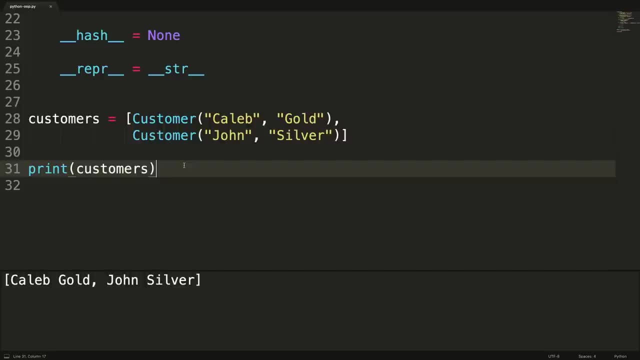 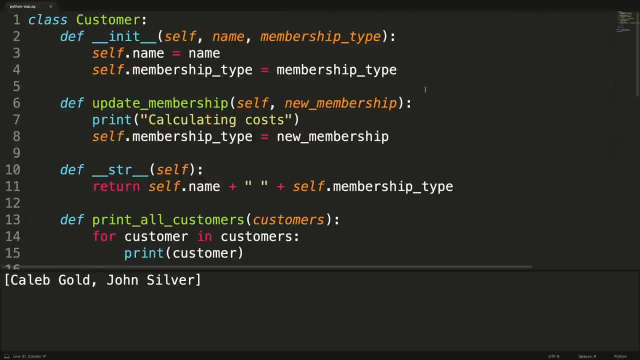 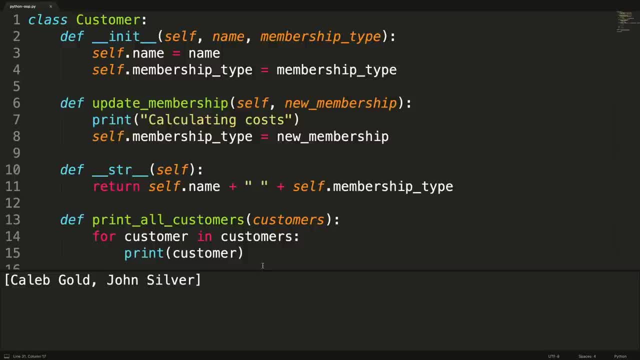 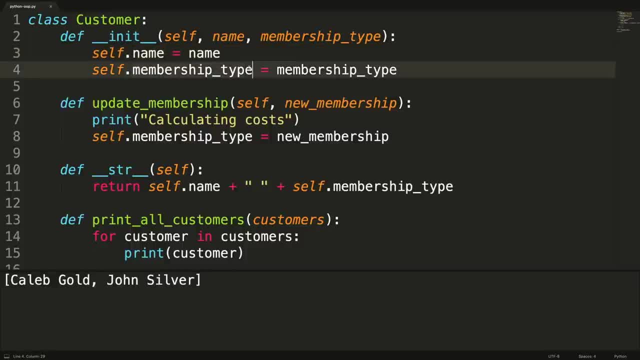 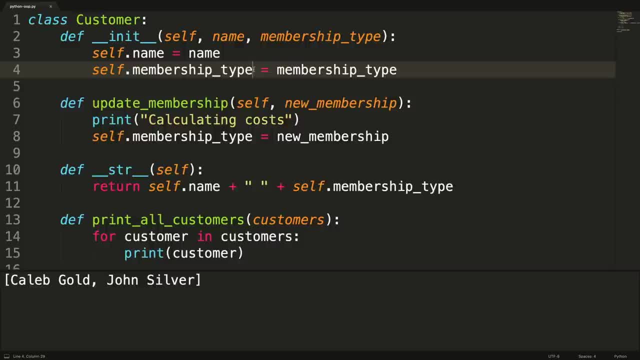 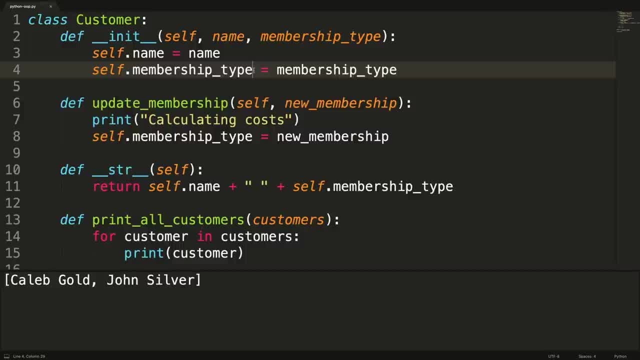 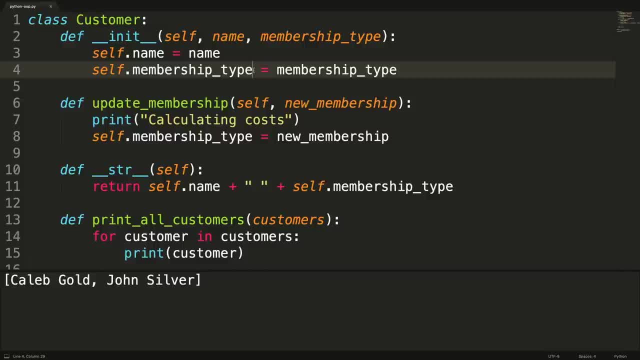 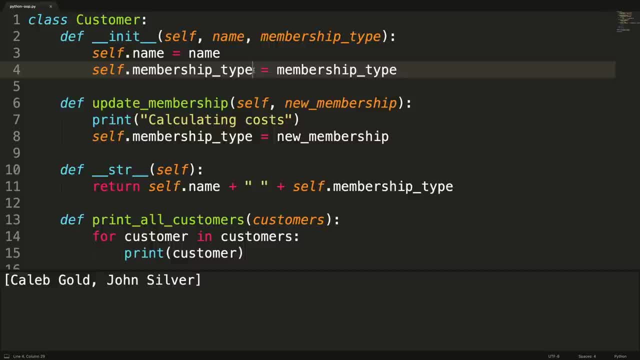 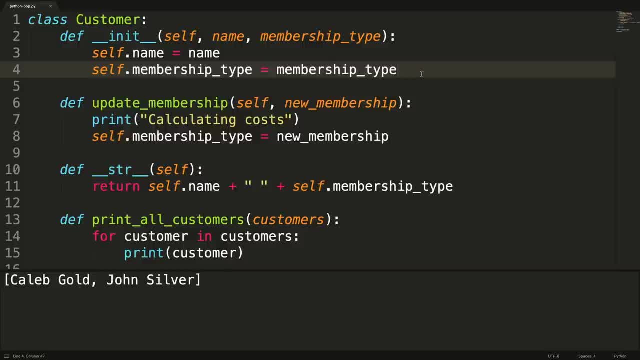 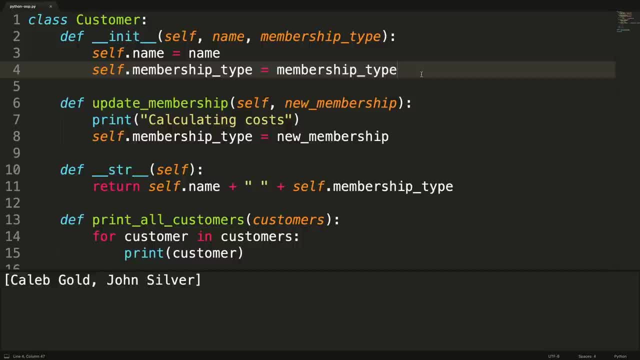 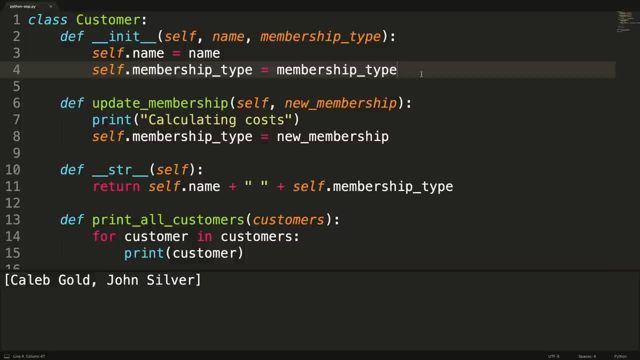 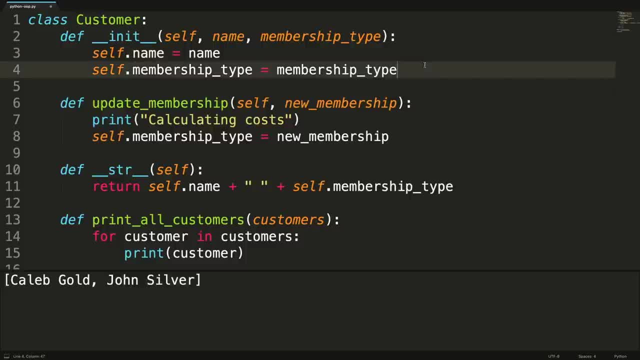 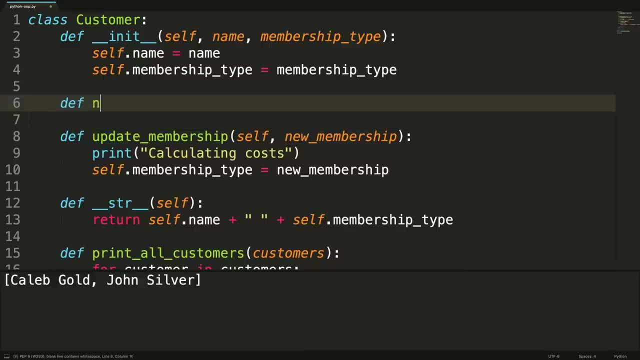 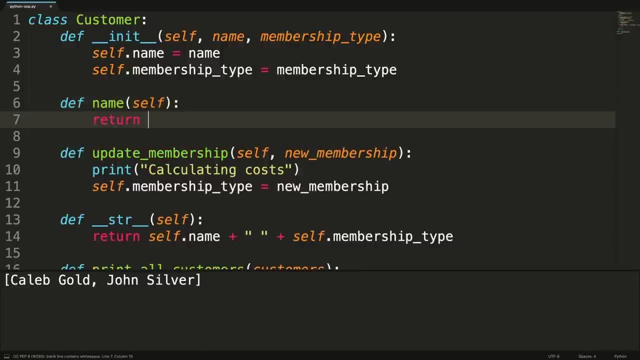 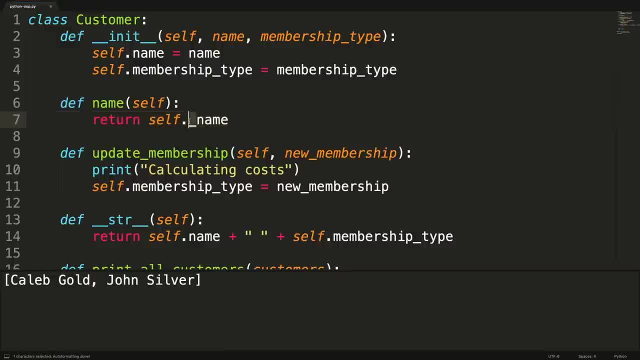 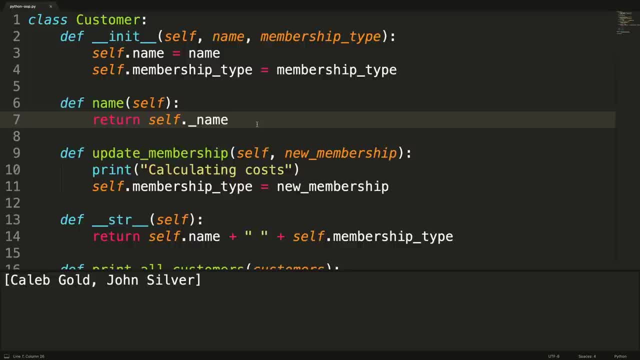 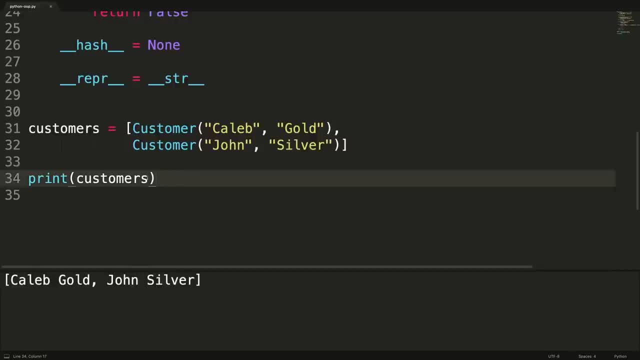 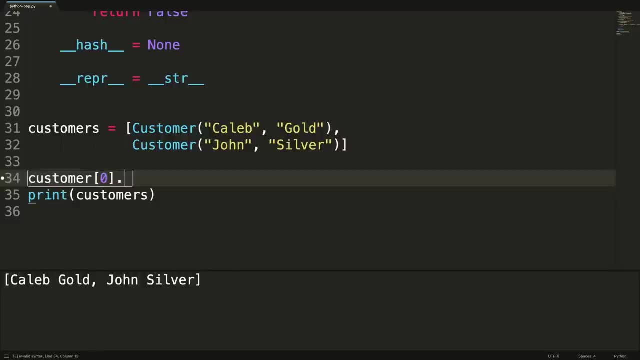 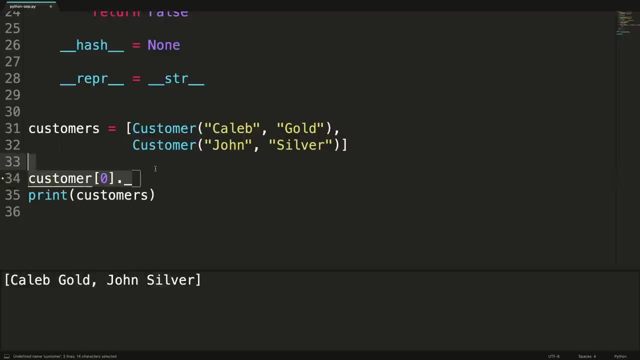 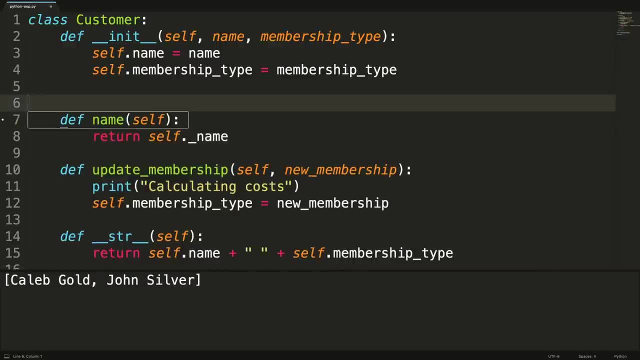 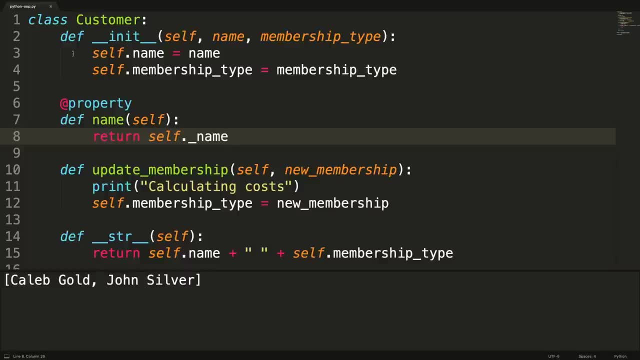 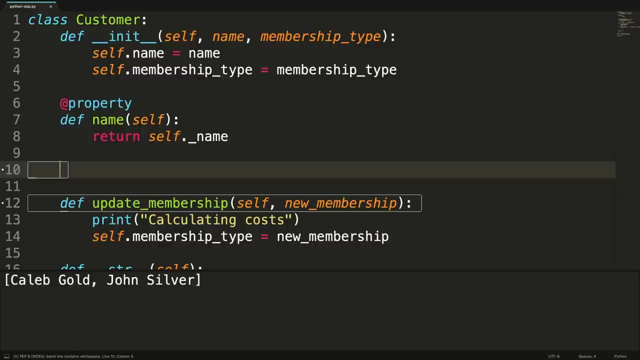 say that this is a property. so when we try to get the name, this is going to be invoked. the underscore name is basically the backing field. it's the data behind the scenes and anytime we try to set this data we need, we're actually going to invoke another method and the way you define that. 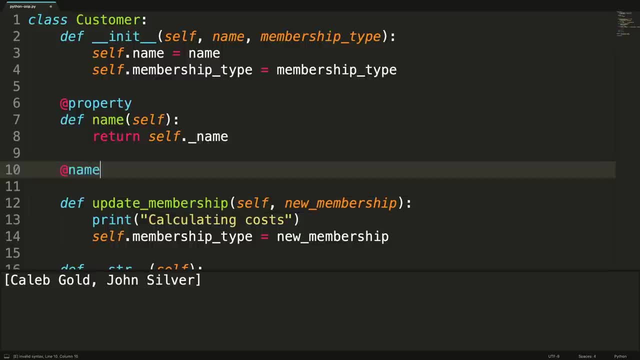 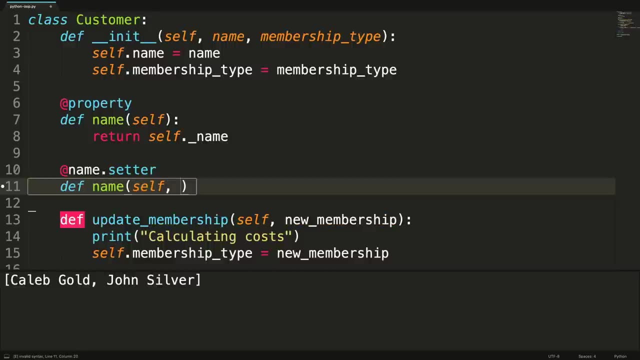 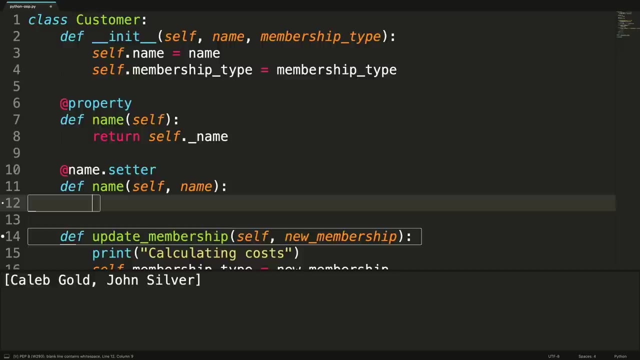 is. you say at, and then you put whatever the attribute is, so name dot setter, and then we say def, name self and then the data that we're going to assign it. so we'll just call that name here and then inside of here we're just going to assign a value to self, underscore name and we're going. 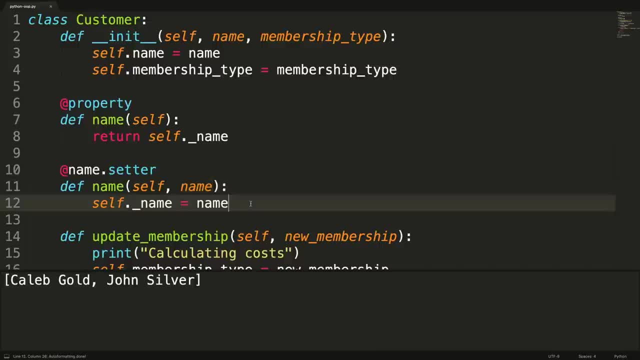 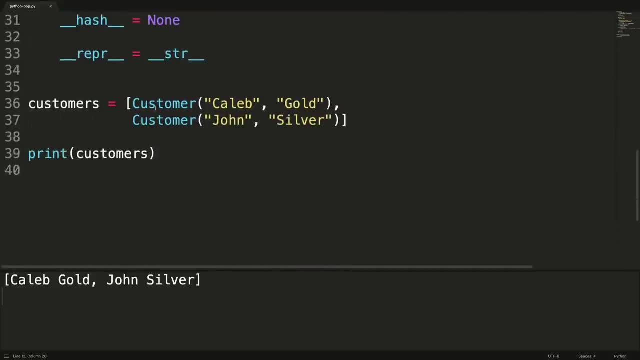 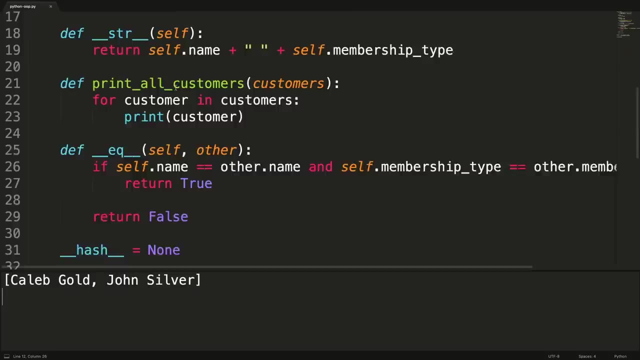 to assign it the parameter value here. so if we save this and run, we get the same exact output, which is what we want. none of the invoking code should have to change to use this. however, we can know that there's an extra step to get and set this data, where we can actually add functionality. 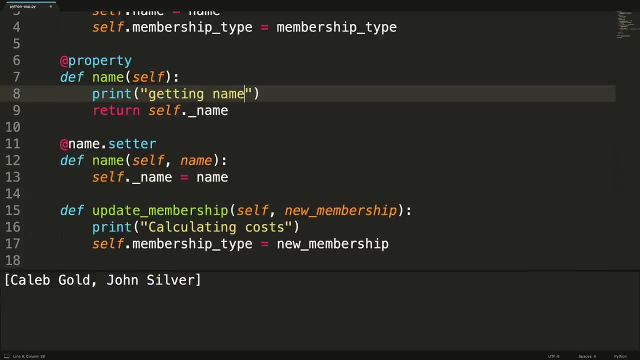 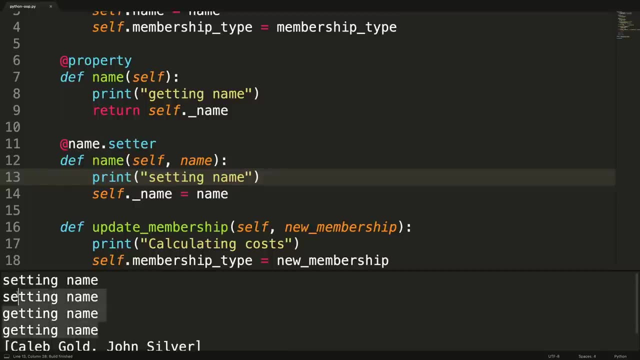 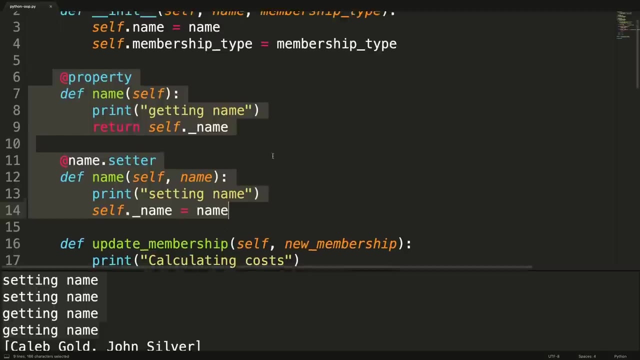 in here if we wanted. so we'll just say print getting name and print setting name running it. now you can see some extra stuff is going on behind the scenes. these methods are being invoked anytime we get or set the value of name. but note that we don't actually have to invoke it like a function, we can just get it like: 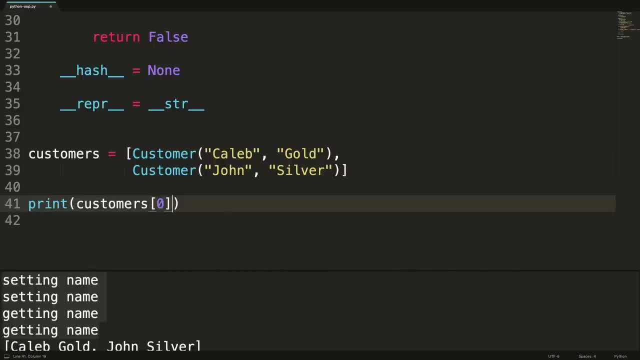 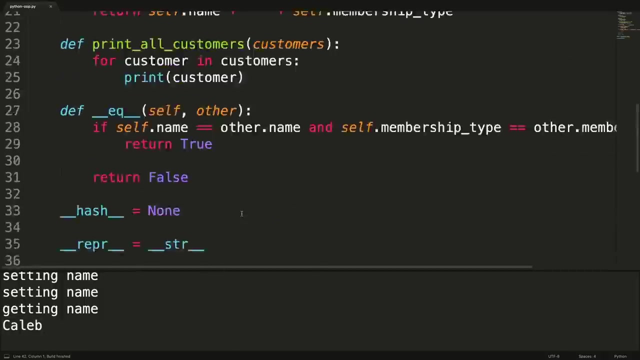 normal, so we can say: customers, let's say we want that first customer dot name, run this, we get Caleb. we did not have to say name with parentheses or get name or anything like that, we just used it like normal and that's what we want. so that is how to create a property. you can do any kind of. 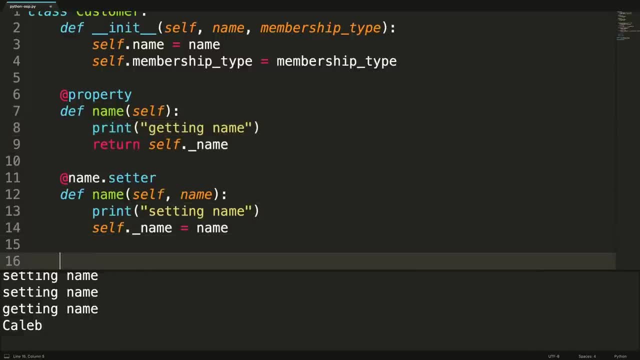 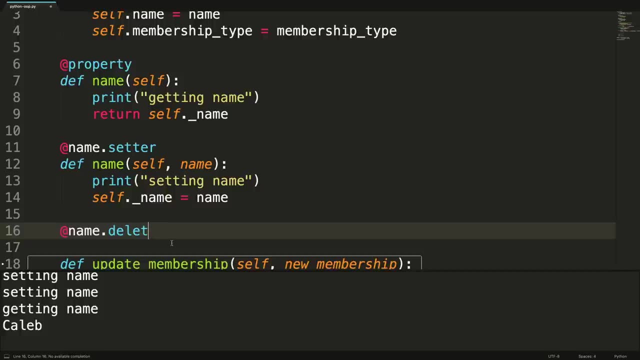 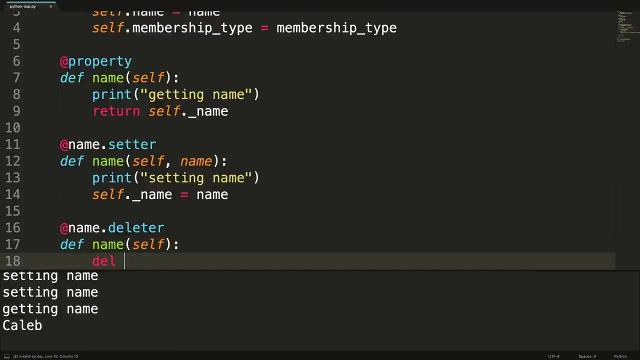 functionality you want in here. you may also want to create a property. that's going to be a property. you can also see what's known as a deleter, which will be used if you use the Dell operator. so that'll look like this name: dot deleter, def name self, and then we just say Dell self, dot underscore name. so 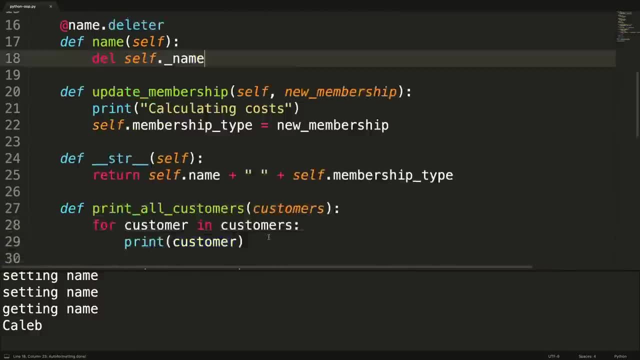 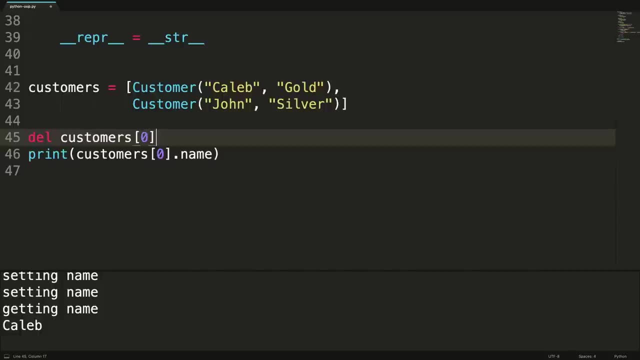 we're not going to use that a whole lot, but just in case you want to know about that now. what that means is we can go down here and we could say Dell customers index zero dot name and running this, it's going to delete it and it's no longer available. if we got rid of that, 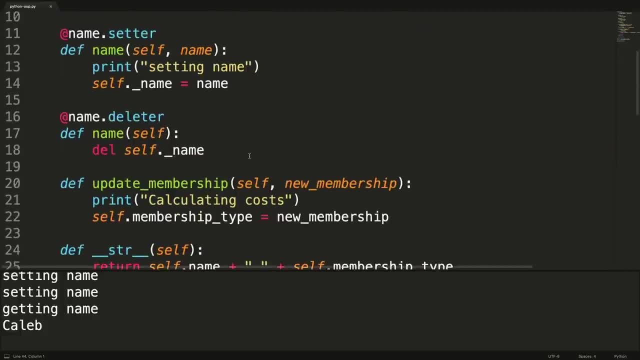 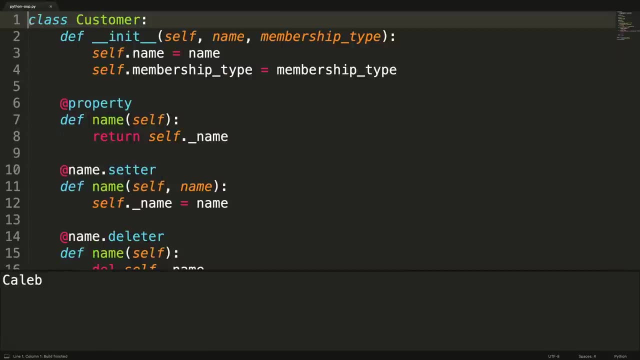 line. it works fine. so let's go in here and just delete that extra printing because it's not really doing anything. just know that. that is where the functionality would go. now let's take a moment to talk about inheritance, and I'm going to keep this really simple. but basically we can create. 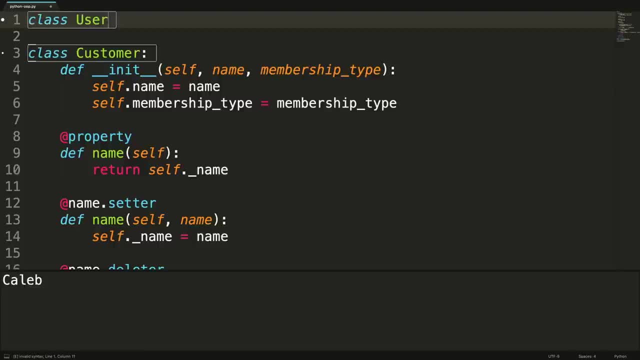 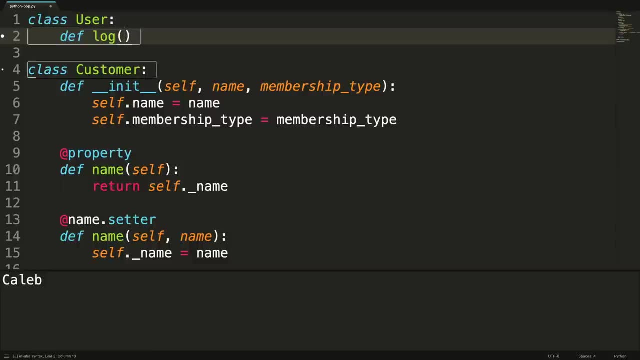 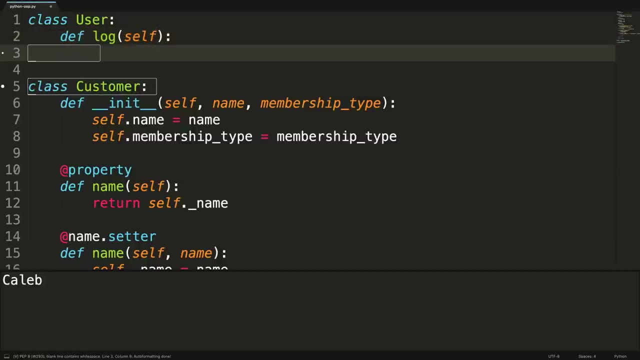 another class that customer derives from, such as user, and we'll just give this user a method. so, for example, we'll say def log. so if we wanted to log some data or something, and inside of here don't forget self, we always want to put self there. inside of here we could just say print self. so as 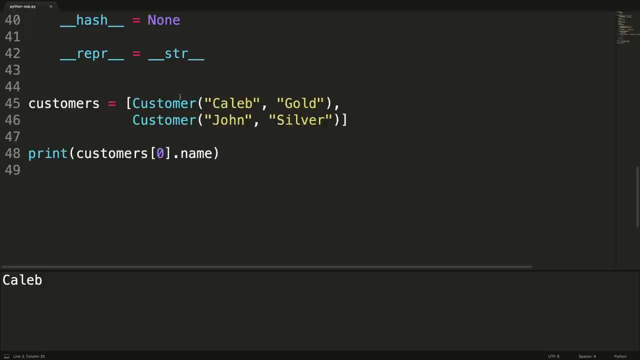 is if we go down to the very bottom of our code and we try to invoke that. so let's just grab our first customer and we say log, we run this and it has an issue. but if we inherited from that base class, then this would be available to us. so here's how. 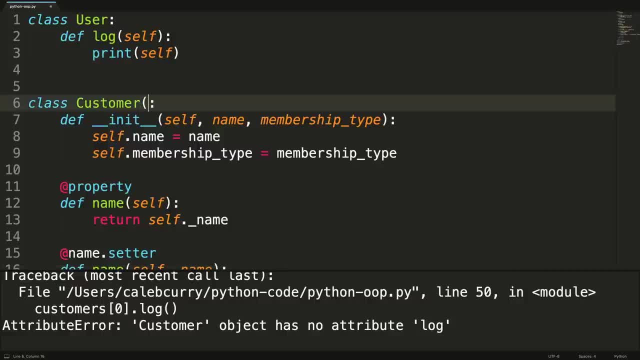 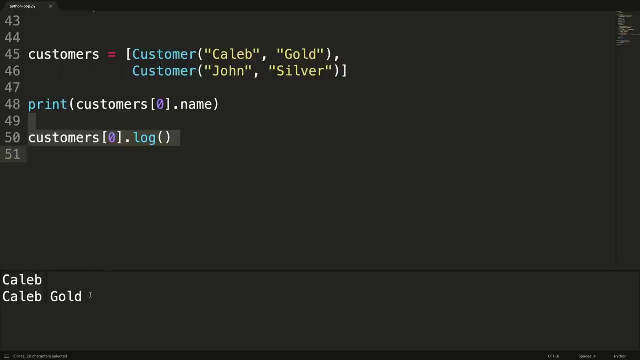 you do that. let's go back up to where we define customer and inside of parentheses you can put user, and now anything defined inside of a user is also going to be defined in a customer. so when we run this now, you can see that this, this log here, works and actually prints all of that: users. 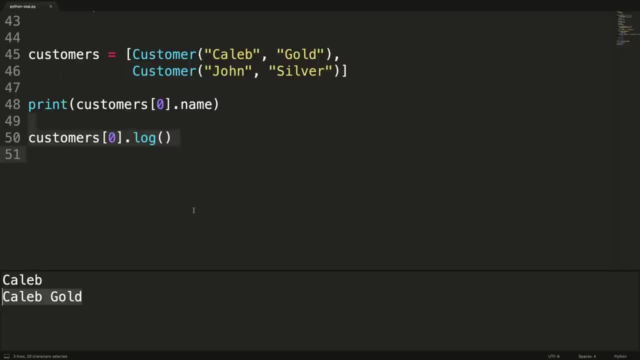 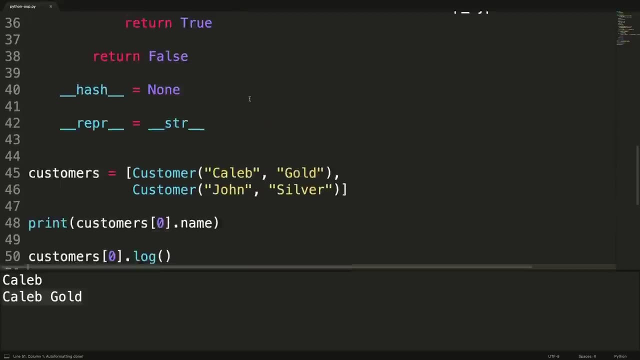 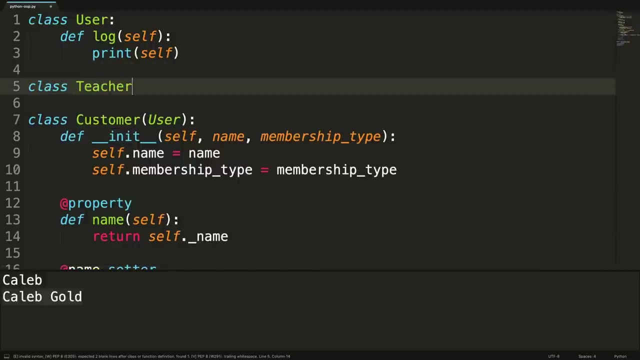 data. so that's pretty simple. when it comes to inheritance, nothing too crazy. the next step of this is polymorphism. so if we actually had a couple of classes that inherited from user, let's say we want to hear and we created a teacher something, and it's also in here. its from. 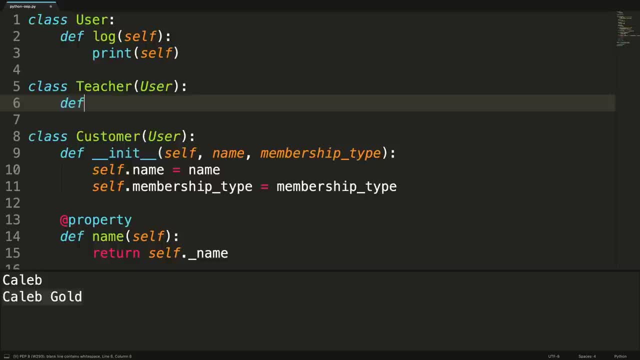 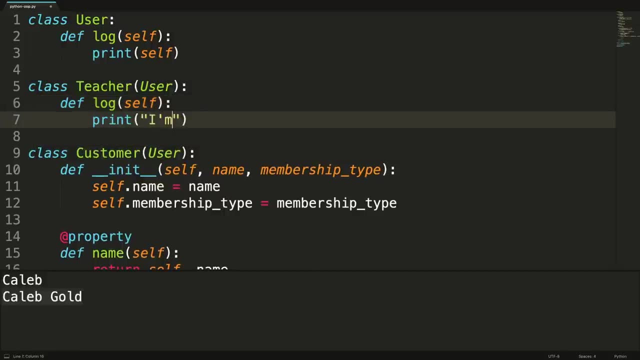 user and we'll give teacher a newланh method and what this is gonna do. its gonna do pretty much the same thing, but it's going to say: I'm a teacher instead of just bringing all the details about them. do this blanket statement for all teachers. So now you can really see polymorphism if you have. 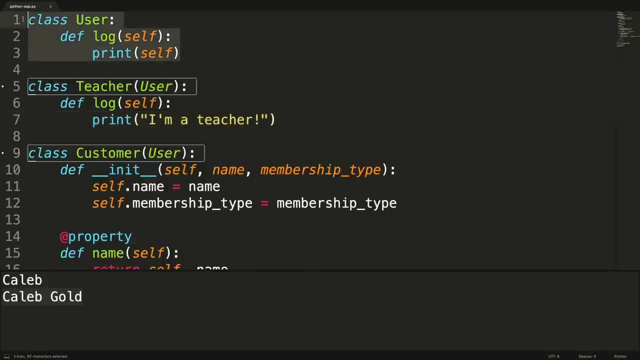 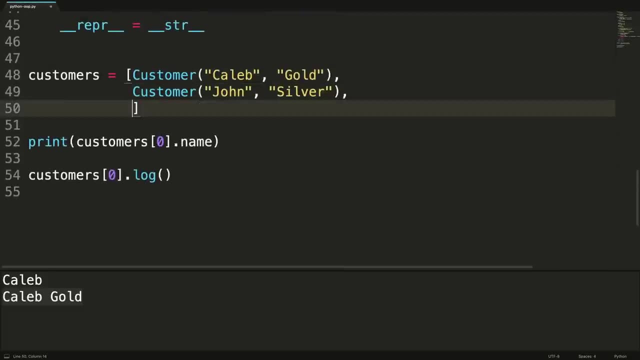 a list of teachers and customers. You can treat them all as users. So let's scroll down to the bottom of our code. here and we have two customers in here, Let's go ahead and add a teacher and just to make sure that we can invoke the log method on each one of these, we'll try it on the second. 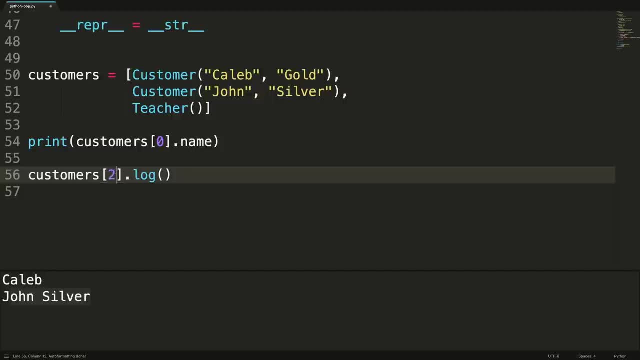 customer. That works, and we can also try it on the teacher and you can see that works. So what we can do now is we can basically take this concept where we take the log method and we're going to do that for all of these people. So instead of customers here, we're going to have users and we say: for user. 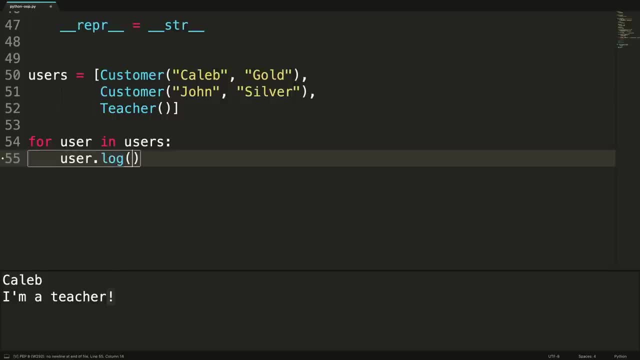 and users and we say: user dot log. So we invoke the log method on every single item in this list and we run it And we don't get any issues. So what exactly is the magical part here? Well, we treat them all as users. 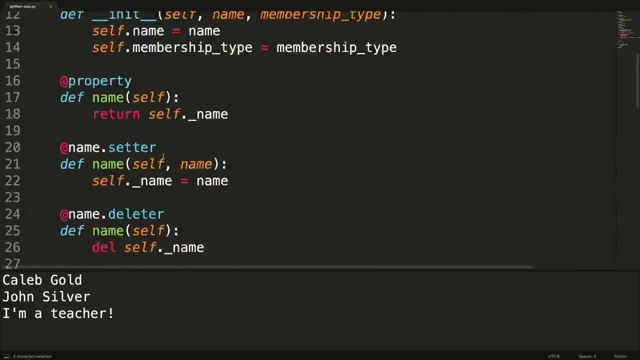 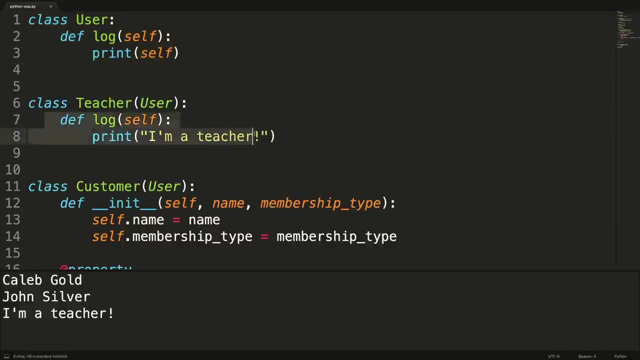 and we invoke dot log because that is part of the user definition. But if a derived class has an override, such as in this case here we overrid the log method and gave a new implementation, then it's going to do the teacher version of that. If we did the same thing for customer, it would do. 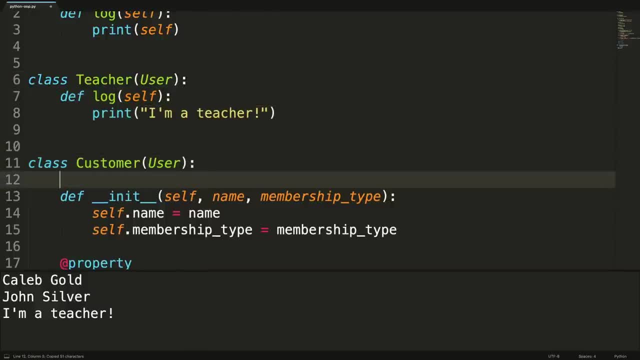 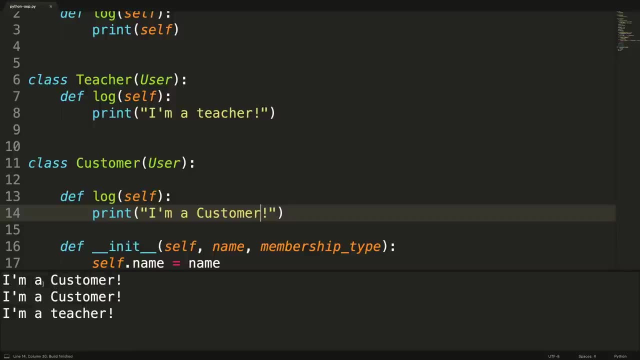 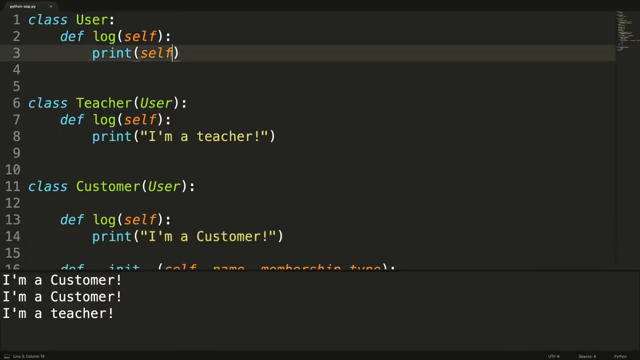 the same thing. So let's see. So let's say, we take this and paste it in here. We can say: I'm a customer And running this, we get I'm a customer, I'm a customer and I'm a teacher. Nowhere does it just do this general print. This would just be. 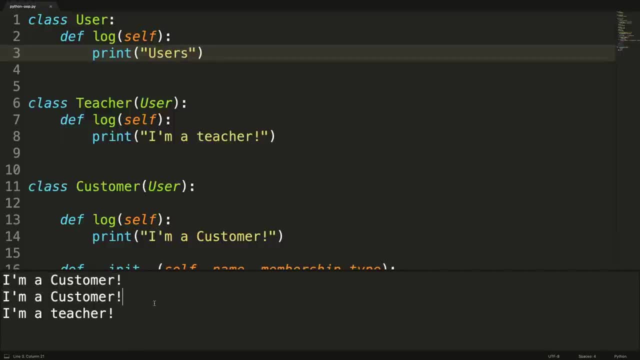 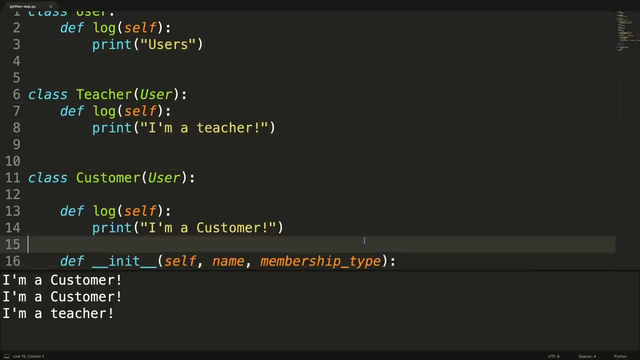 for the users, and you don't see that anywhere. So that is the basics of polymorphism: Basically, the ability to create code that works with general users but is still a user. So that's the basics of polymorphism. It's still fully functional when you're past something more specific, such as a teacher or a customer. 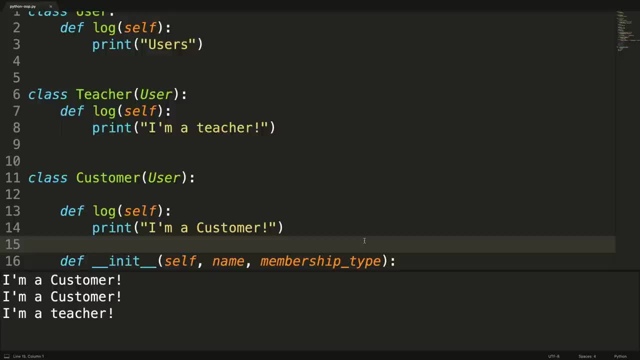 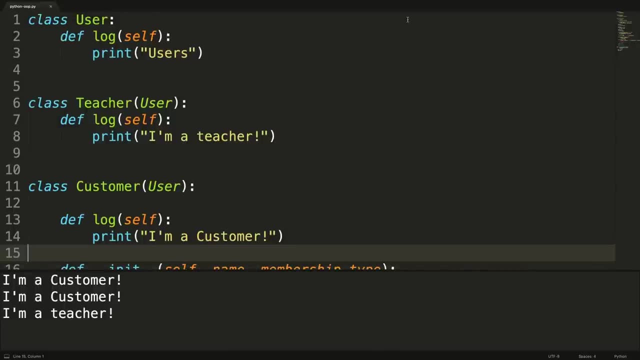 Now I know that's a lot and probably these principles will take a lot more practice to truly grasp and see where to apply these. We've touched all the basics of object oriented programming and now some more advanced stuff might come a little bit easier. If you're looking for other stuff to research you, 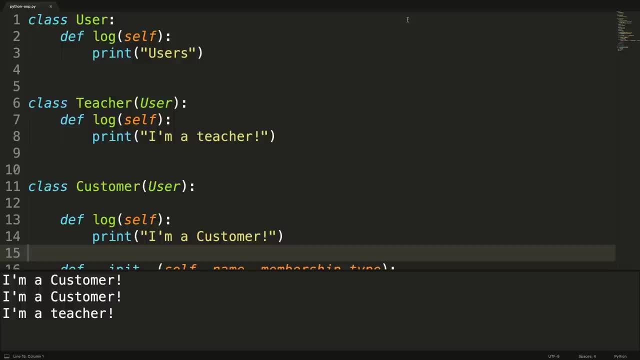 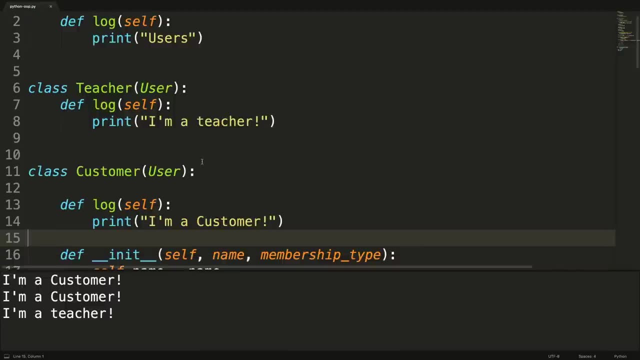 can look into object relational mappers. This is basically going to take database data and correlate it to a bunch of objects in your code, and then you're going to see that there are other ways of doing this your code. So instead of just working with hard-coded stuff in here, you could 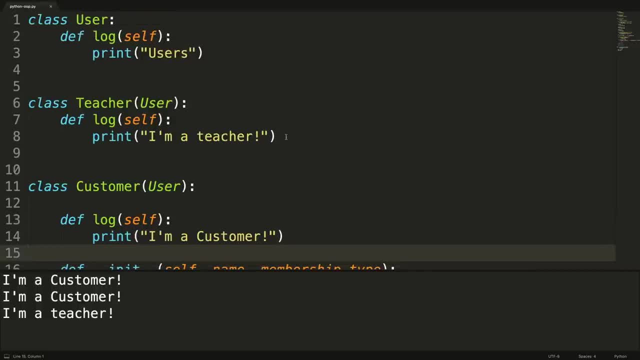 be working with actual teachers and customers. in a database You could also look into some different object-oriented design patterns. These get pretty advanced and basically teach you how to design programs using these OOP principles, And there's probably like six quadrillion other things you can study, so just look. 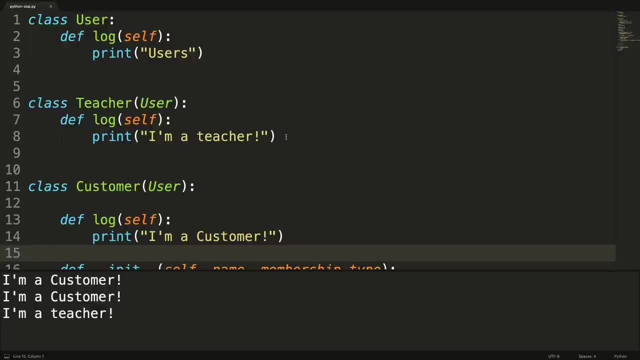 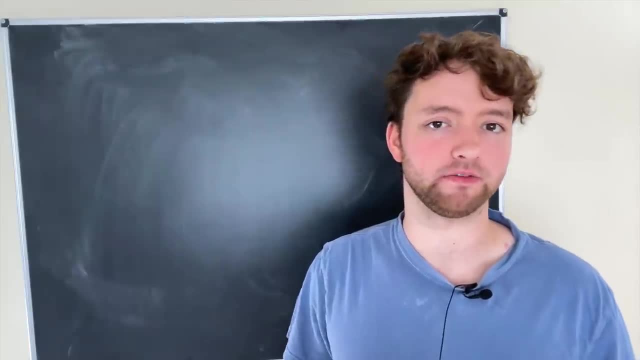 up some more advanced object-oriented programming things and start learning. Thank you, guys, for watching. If you've enjoyed this content, please be sure to subscribe to this channel. Also, be sure to check out my channel, Caleb Curry. We got stuff on Python, JavaScript, C++, Java C, sharp database design, all kinds of.